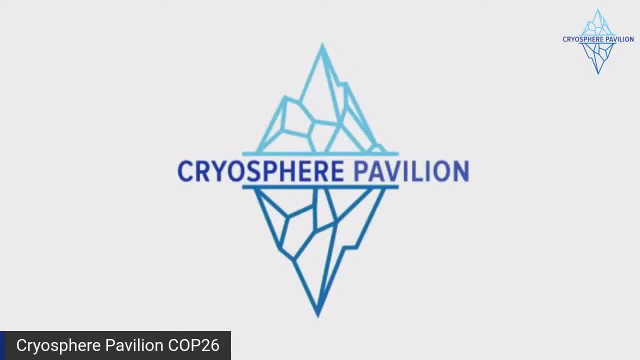 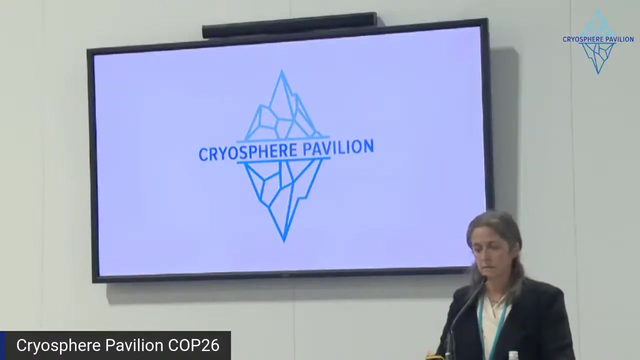 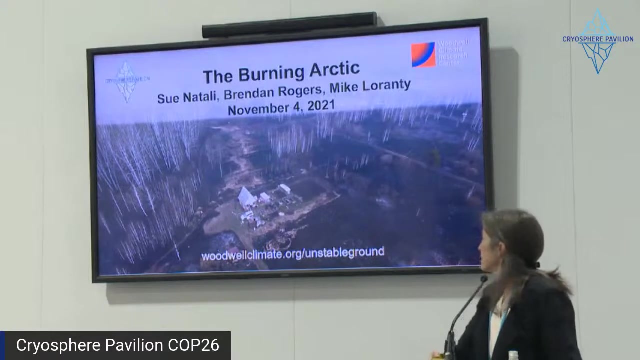 Thank you. Thank you, Excellent, All right. Hi everyone. My name is Suna Talley, I'm a scientist, I'm the Arctic Program Director at Woodwell Climate Research Center, And this next session is going to focus on wildfire and permafrost in northern regions. 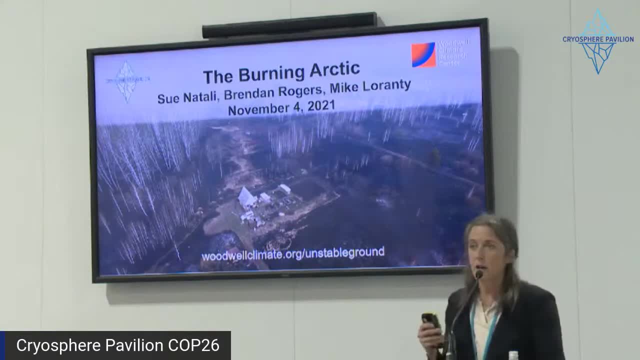 We had some sessions about wildfire yesterday And what we want to highlight in this session is that the interaction between wildfire and permafrost thaw. So I'm going to start with a quick overview of the processes and what's happening now in the Arctic. 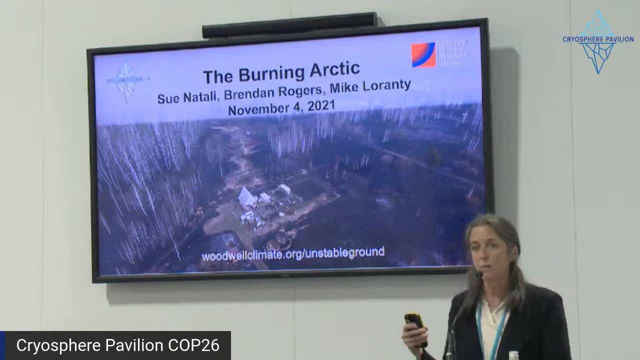 The next speaker will be talking about projections of future change, incorporating wildfire and permafrost thaw, And then we're going to have another panel. We had just an excellent panel. I hope you are all here for it. We have another panel that will feature Arctic residents to talk about the changes that they're seeing on the ground. Okay, So wildfire in the Arctic and boreal regions have been happening for a long time as part of the sort of natural ecosystem processes. This isn't a problem when we think about greenhouse gas emissions, or hasn't been, because regeneration is happening fast enough to sort of make up for the carbon that's lost during emission. 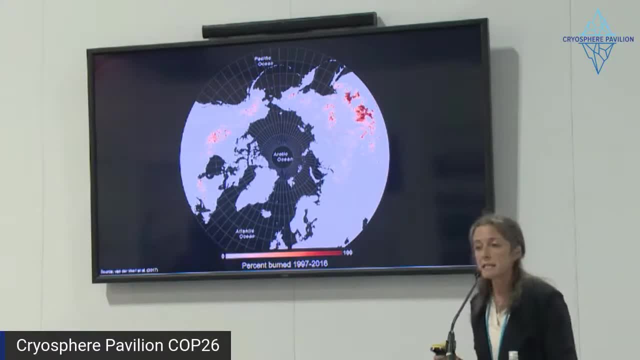 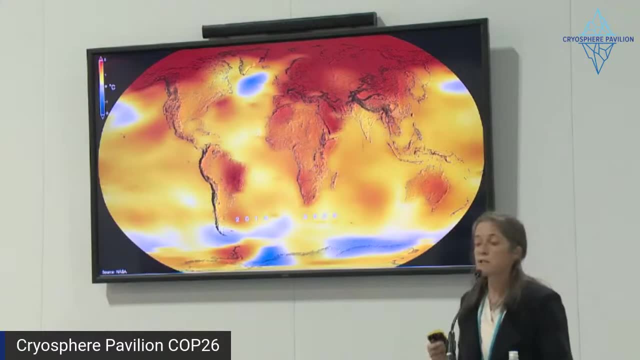 But recently the fire intensity and severity have been increasing across the Arctic, similar to other parts of the planet, And there's a number of reasons for that. I mean one of the big reasons why wildfires are increasing in the Arctic is because the winters have been warmer. 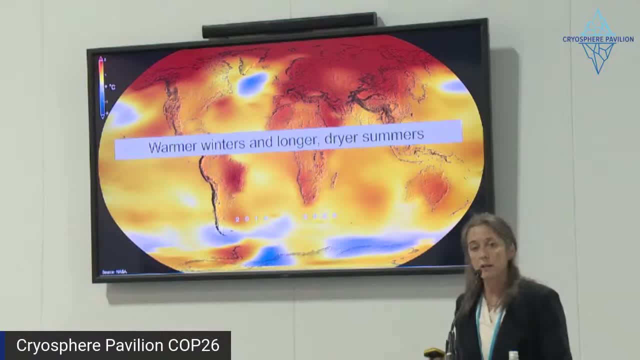 The growing season has been longer. 2020 was a record fire year in Siberia. 2021 broke that record. The winter before 2020 was quite warm. The growing season started earlier. it was quite dry. There were temperatures above 100 degrees fahrenheit above the Arctic Circle. 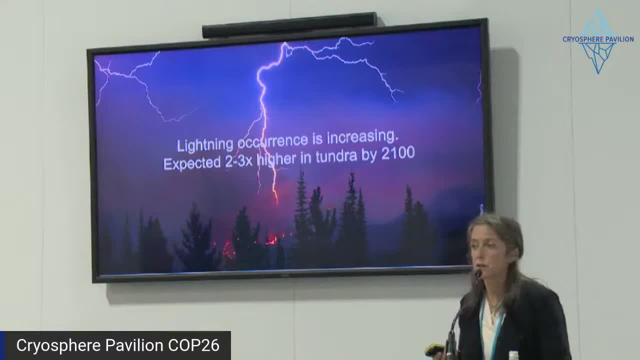 The other thing that's happening in these northern regions is that lightning is increasing, And so you know lightning was very infrequent, if occurring at all, all in the tundra, And, anecdotally, more and more you talk to Arctic residents and they talk about 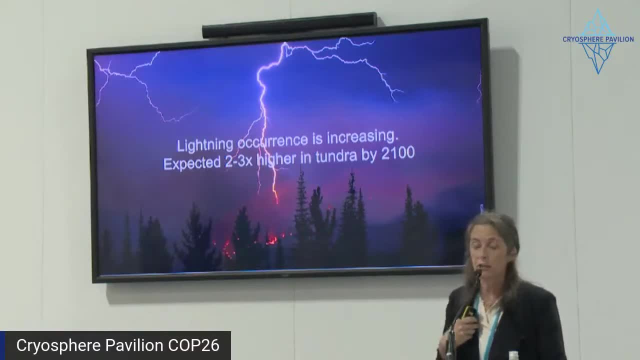 seeing lightning. I had never seen lightning in tundra until a couple years ago, And now lightning training is part of our field safety when we take scientists out to the tundra, And that was something that was never part of what we were thinking about. And then lightning. 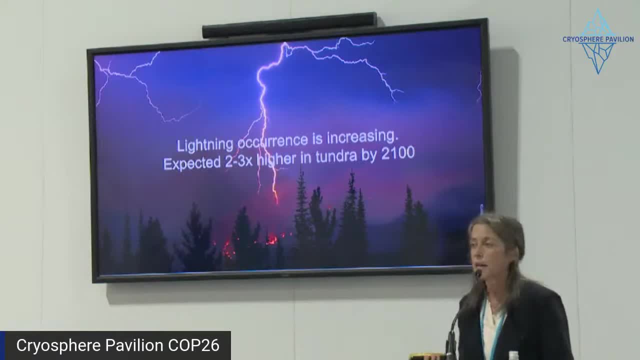 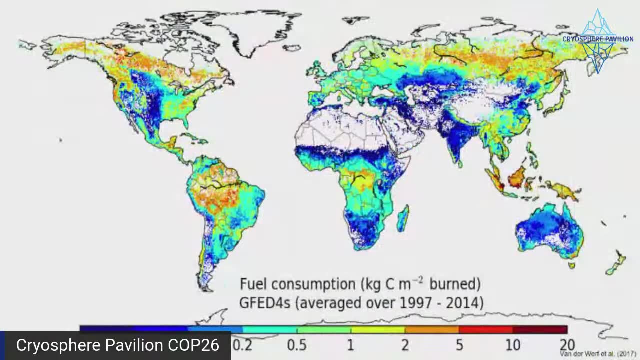 strikes are also expected to continue to increase two to three fold, And the reason for that is because of climate changes, changes in atmospheric conditions. I want to show this. This is a map of global fuel consumption And I think you know when we think of wildfire, at least in the US. 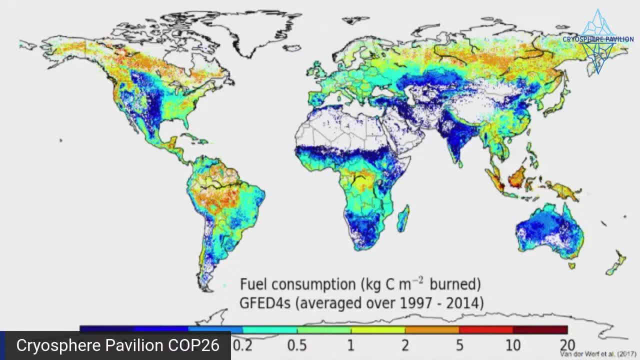 we think a lot about what's happening in the western United States, But if you look at this map, the orange and the red areas are areas of high fuel consumption And you see these places in the northern latitudes are some of the highest fuel consumption in the world. 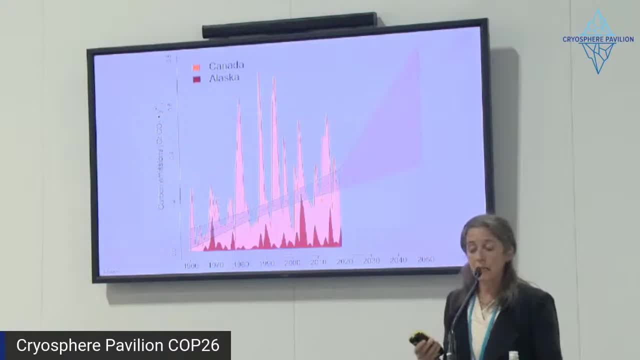 And so as fires increase, carbon emissions are also increasing, And one of the big reasons why there's such high fuel consumption in the northern regions is because, as you've been hearing in these previous sessions, all of the carbon that's stored below ground. So when fires burn in the Arctic. they burn the vegetation like everywhere else, But it also burns below ground because there's massive stores of carbon. Whoops, Okay. So this is just some trends of carbon emissions from Canada and Alaska. We see have been increasing fires over the past several. 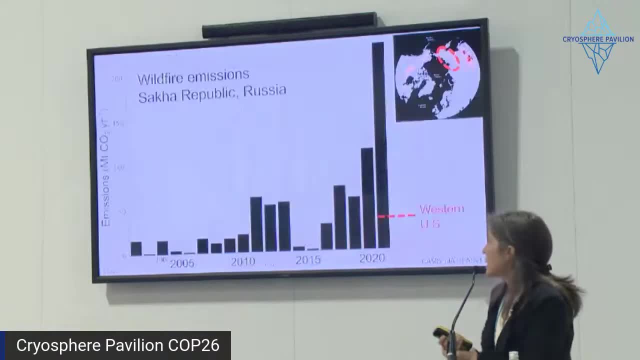 decades and projected to continue into the future. And then here are some fire emissions from Saka Republic, And this is where I want to point out: you know, if you look in this last bar, this is 2021, and it's almost off the charts If we think about what's been happening. that dash line is: 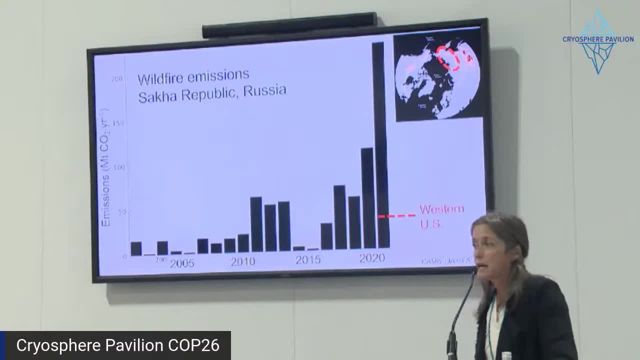 the emissions from the fires in all of the western United States. So this is really quite substantial in terms of carbon emissions from Canada and Alaska. And then here you have some fire emissions, of carbon emissions in terms of black carbon, in terms of smoke impacts and all the other impacts. 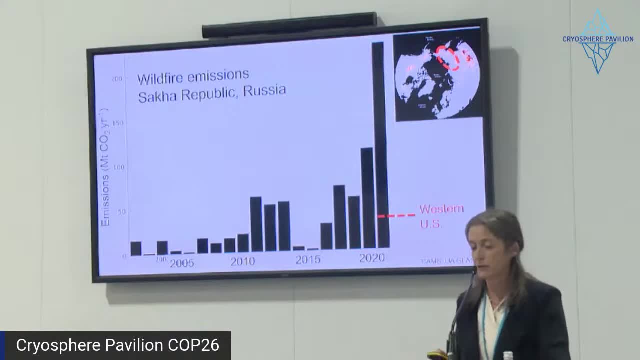 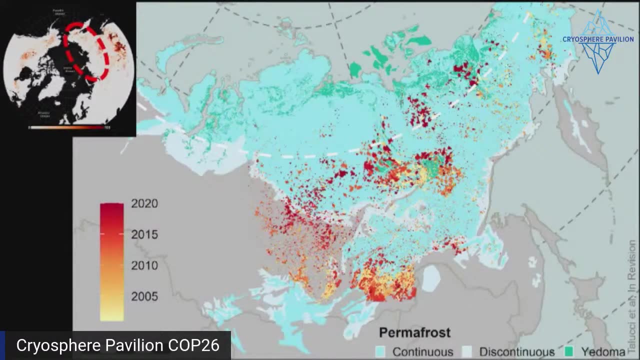 that are happening on the ground, which you'll hear about in the piano at the end of the session. so this is another view. this is northeastern russia and fires. you can see the dark here. the dark red areas are fires that are happening. in the past five years we see this increase in. 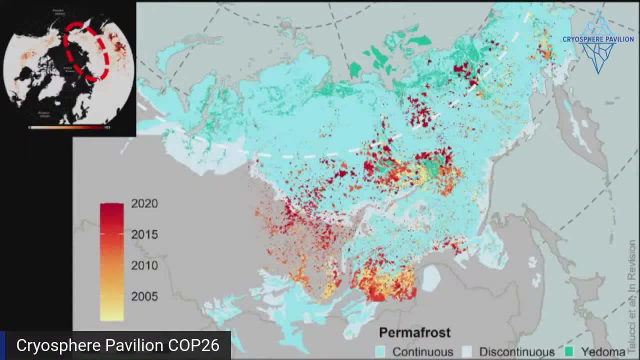 fires in the recent years. but also fires are moving north, so we're seeing more fires in tundra regions and areas where there are very deep peat deposits. but the other reason i think i want to point out here is that the blue shading here is all areas where there's permafrost. so 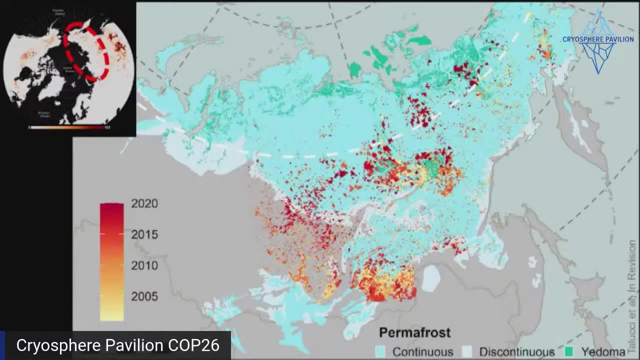 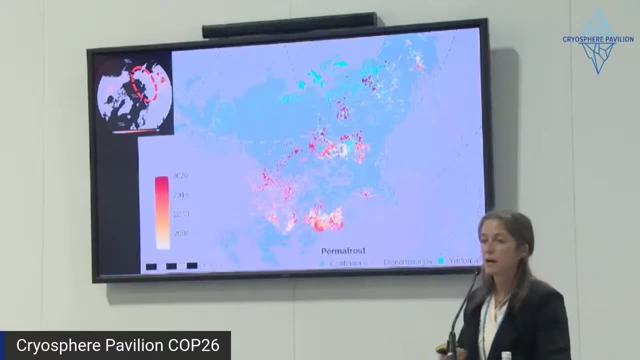 perennially frozen ground and we're starting to have fires increasing on areas where there's permafrost. and that's a problem because when the fire burns off the vegetation and it burns off the organic matter, that vegetation or the organic matter is really good insulation for permafrost. so 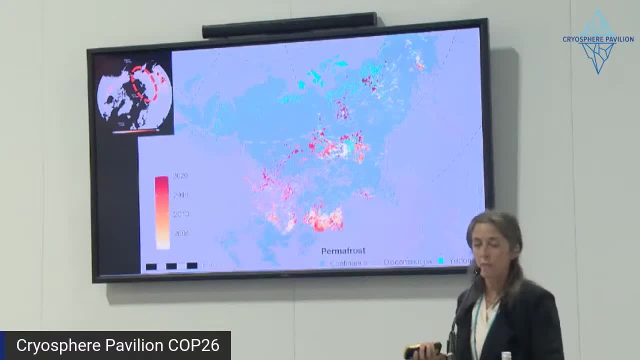 when you remove that in the summertime, it's essentially like opening the top of a cooler. so all of a sudden now this permafrost is going to be a little bit cooler and it's going to be much more vulnerable than it was before the fire. so you get this carbon pulse with the fire. but 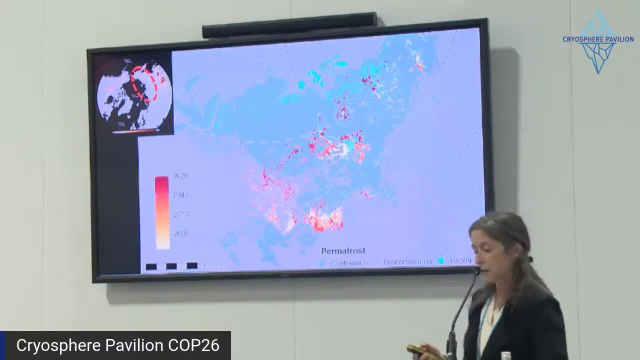 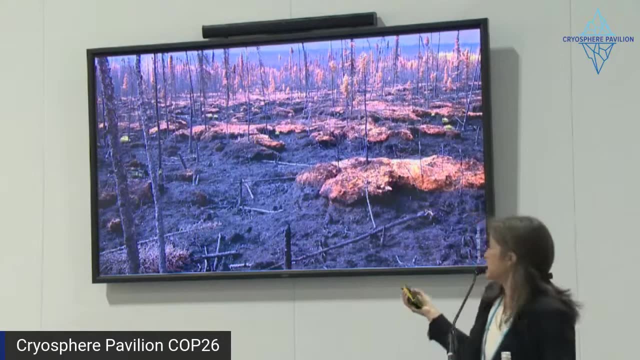 now you're also making these systems vulnerable over very long time frames. so this is what it looks like when fire burns in a permafrost area. you can see this is an area with these areas that are light brown, that's kind of sphagnum moss patches, and the fire is burned off all the vegetation and down into the soil. 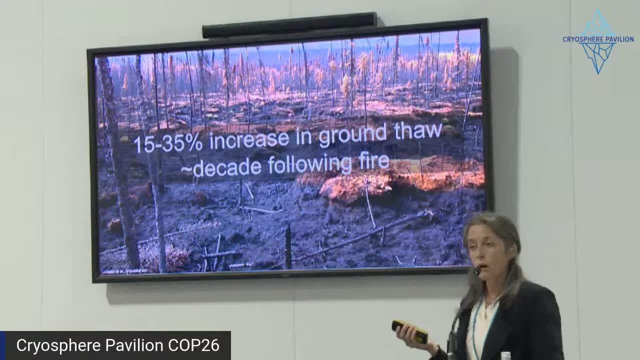 as i said, the impacts of fire can last for decades or more. um, ground thought increases anywhere between 15 and 35 percent, up to a decade or more following fire. okay, so the other thing i want to talk about, which has gotten quite a lot of headlines, is: 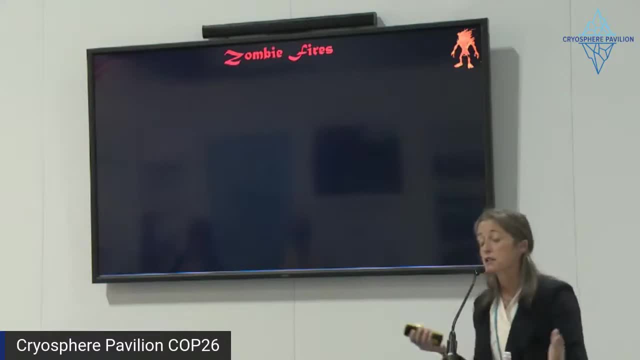 zombie fires. um, zombie fires aren't something that's new, but they are happening more frequently and they got a cool name. so now everybody's talking about them. but essentially a zombie fire is just a fire that overwinters really. hopefully the drought eases up higher and higher by the end. 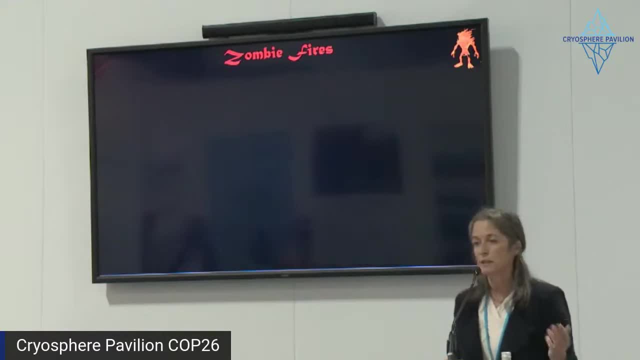 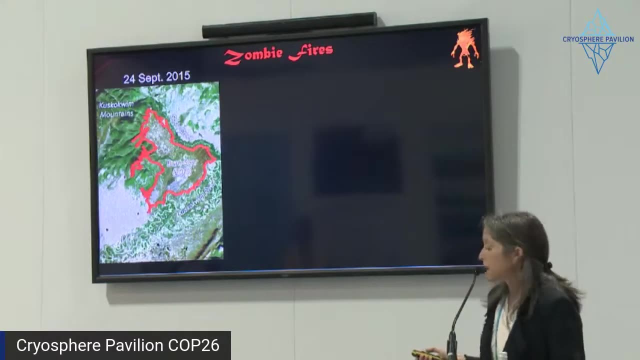 of the year, but we know those dangers are actually dying down longer. but we know that this is from one year to the next, and the reason this can happen is because the fires are burning below ground, because there's so much carbon, and so here's some satellite. 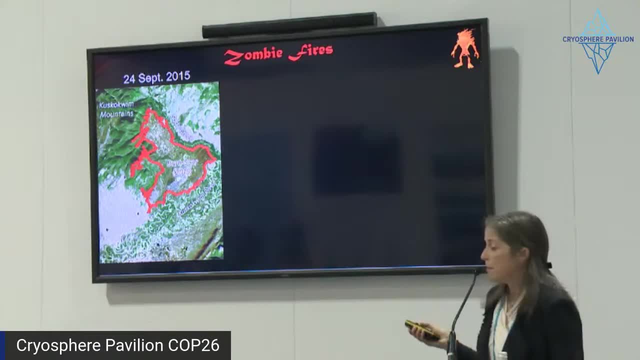 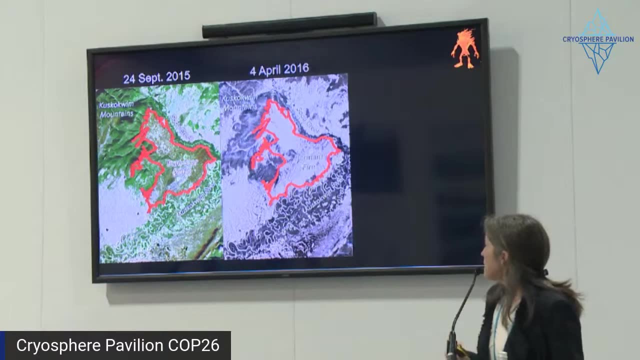 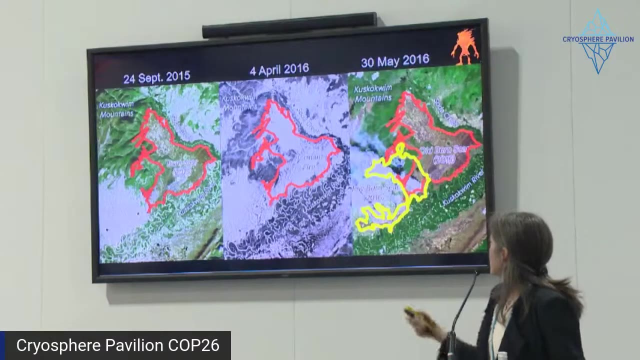 imagery. this is a fire from 2015 in Alaska and you can see this is the outline of the burn scar from September. and then here we see that burn scar in April and then this is a new fire that ignited in May and and people who live. 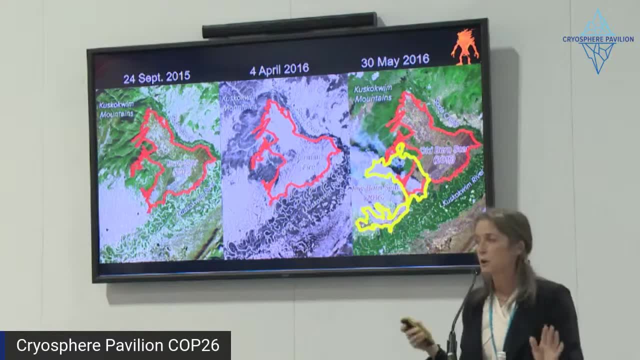 in Alaska. know like, know this is a sorry live in the Arctic. know this is a thing that's been happening. you can see where there's a fire the year before, and then you go in the spring and you start seeing the smoke again. the reason that these are increasing is they're related to the. they're related to climate and 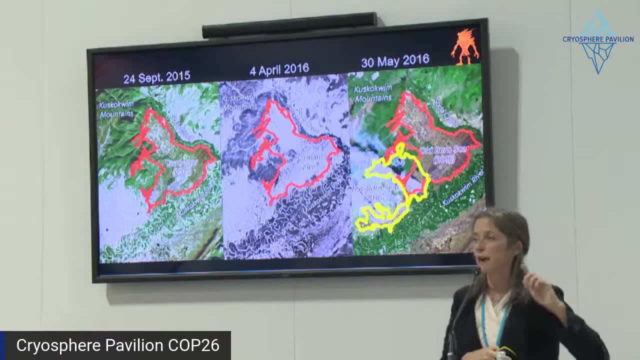 they're particularly related to the previous year's climate, and so increased fires cause a lot of damage to the environment, and so you can see that those increased fires, so there's a positive feedback. when you have more fires, you have more of these zombie or overwintering fires, so you can see that. 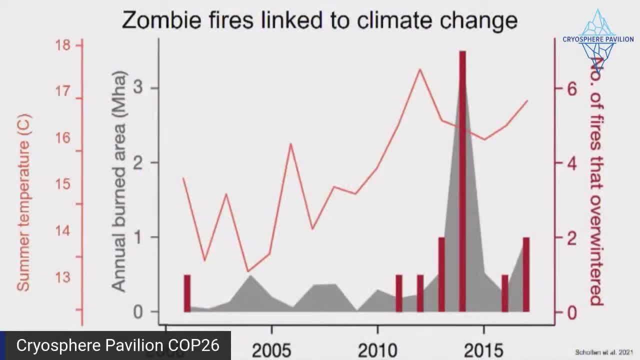 in this figure here. so the um. the orange line is the previous summer's temperature um. the gray bar is the annual burned area, so this is from the previous year, and then the red bars are the number of fires that overwinter. so we see in years where there was a lot of fires the previous year and also there was a very 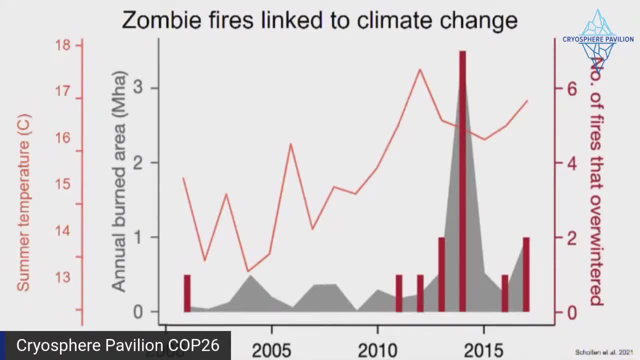 warm previous year. this then leads to increased overwintering fires, But the other thing that's important about these overwintering or zombie fires is that they also burn deeper. So we've had and one of the things that's happening in the Arctic. 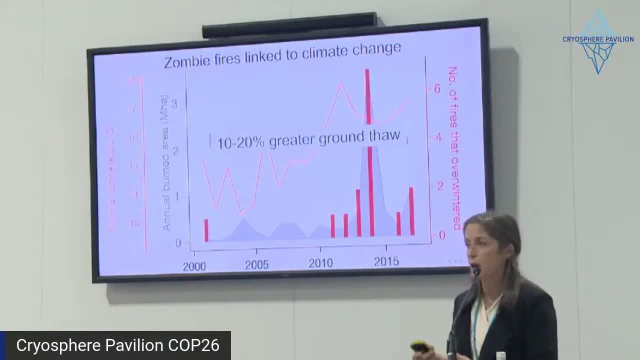 is, soils that used to freeze through the winter are now staying thawed throughout the winter. This is the other reason why allowing these overwintering fires to increase, And so they're causing more fires and then also causing fires to burn at a deeper level of thaw. 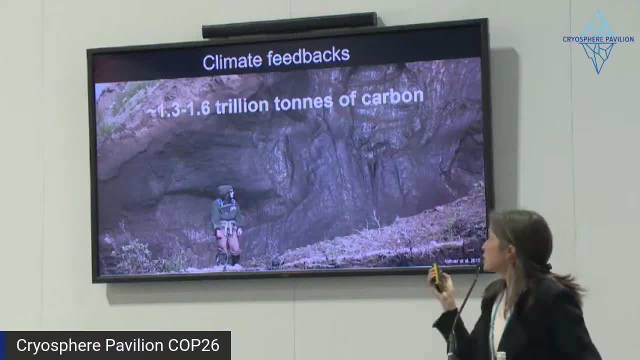 Okay, so just to keep in mind, the next speaker is going to be talking about the global implications and then we're going to talk about the regional and local implications, But I just want to point out: globally, there's a lot of carbon that's stored below ground. 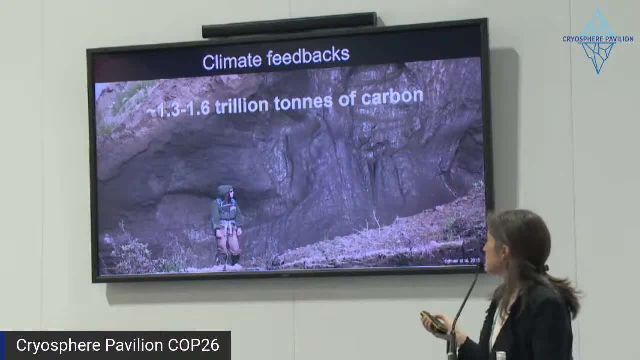 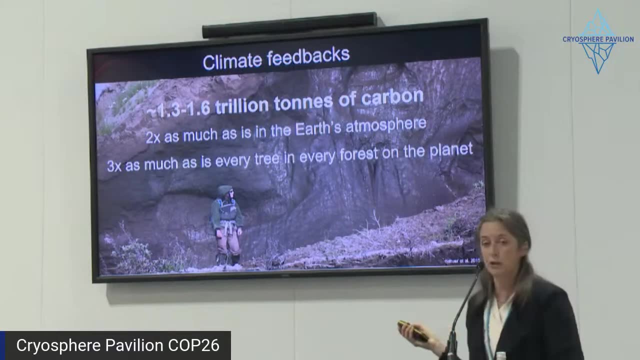 The fires are burning off this carbon. You know 1.3 to 1.6 trillion tons of carbon stored in the northern permafrost region, twice as much as in the atmosphere and three times as much as in every tree and every forest on the planet. 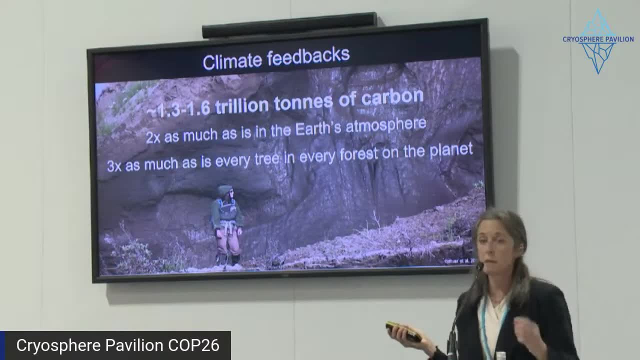 So this is a large pool. This is a pool of carbon that's becoming more vulnerable, and it's becoming more vulnerable both because of thaw and because of fire, And one of the things that's important to keep in mind is, yes, this last IPCC report, so AR6,. 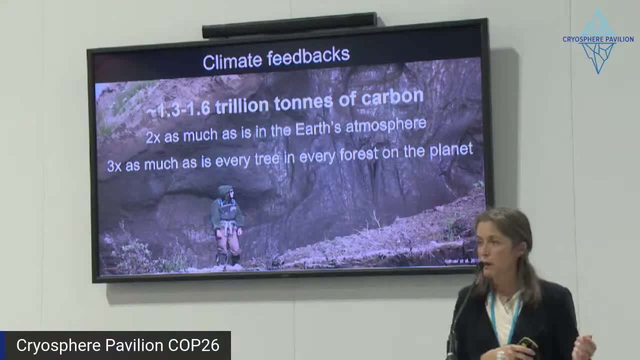 did incorporate in the carbon budgets permafrost feedback. It did not incorporate wildfire impacts on permafrost thaw. It did not incorporate burning below ground from wildfires. So there's carbon emissions from the Arctic that are happening that currently still are not incorporated. 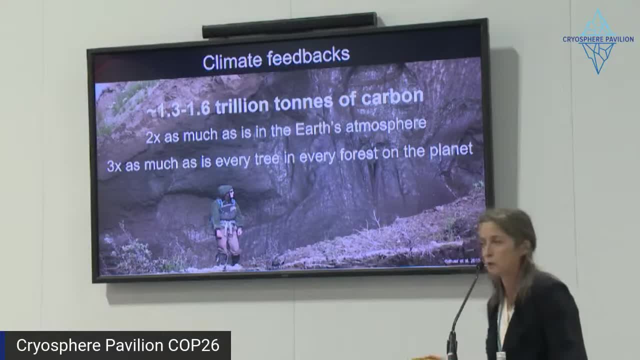 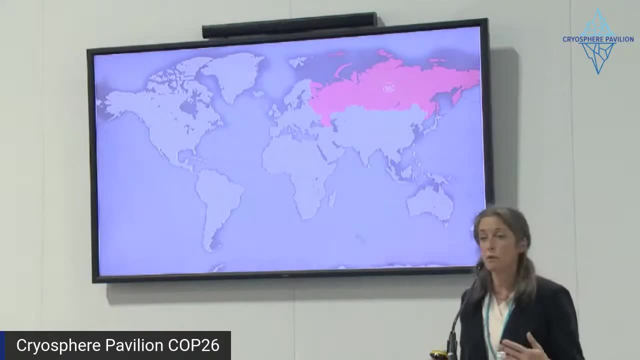 One. we're thinking about how much carbon will be released as a result of climate change in northern regions. Okay, so what does this mean in terms of how much carbon will be released, The estimates of carbon emissions? there's still a lot of uncertainty. 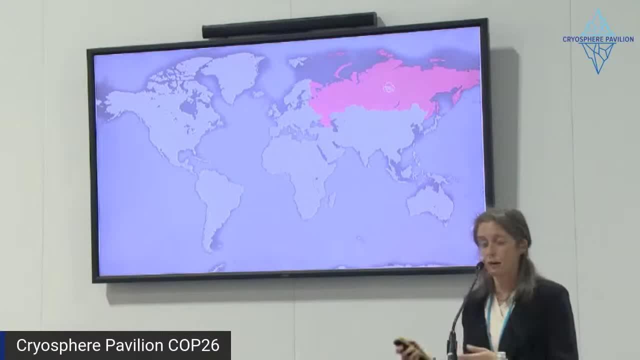 but I just want to point out- and partly because we're not accounting for fire- and our next speaker will talk about this some more- but by the end of the century they may be on par with Russia, with India or with the United States. 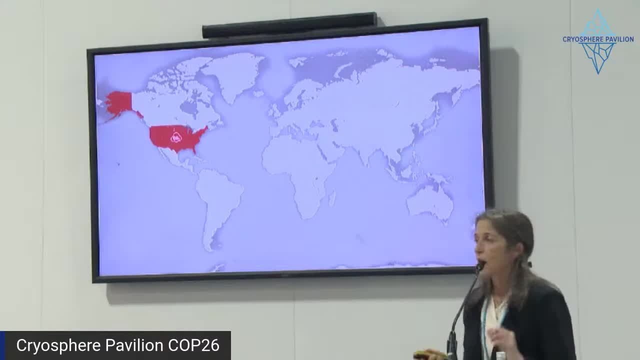 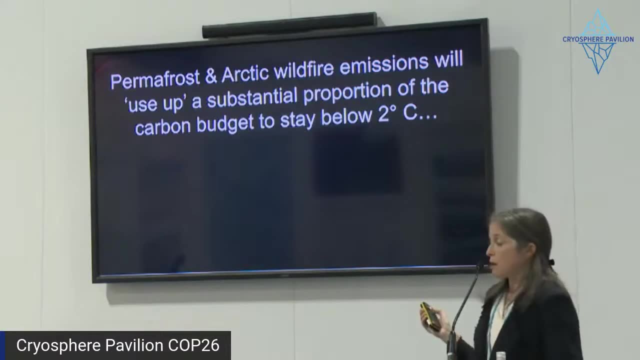 So these are some of the largest global gas-emitting countries And not fully accounted for in an appropriate way. Okay, so permafrost and Arctic wildfire emissions that will use up a substantial proportion of our carbon budgets. We'll hear just how much in our upcoming talks. 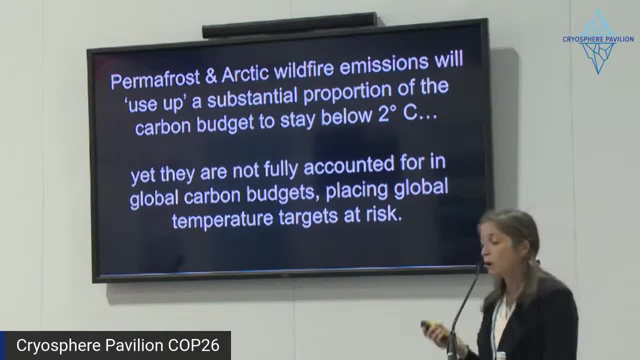 Yet they're not fully accounted for placing the global temperature targets at risk. There's no way we're going to make 1.5 or 2 degrees Celsius for many reasons, but we're never going to make it if we don't do the accounting properly. 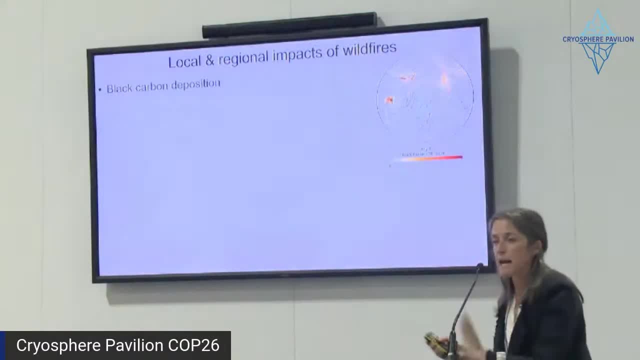 And I just want to touch on this. We're going to touch on some of the local impacts and our speakers will be able to hit this much better than I am, because I am not an Arctic resident. But we know there's concerns from wildfire because of black carbon deposition. 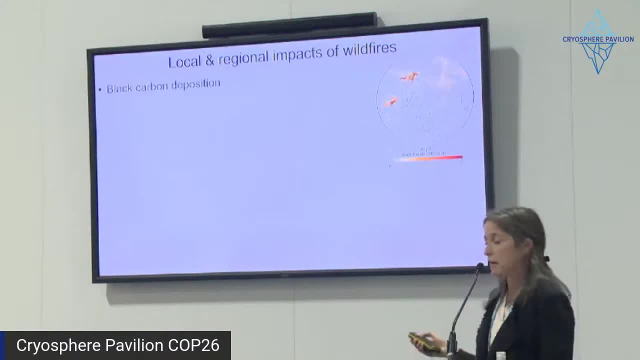 which can land on ice and snow, leading to additional melt and regional feedbacks, Of course, impacts of smoke inhalation and human health. You know aviation- in northern regions- flying- is how most places are accessed and this is a big problem in terms of bringing in food and other resources. 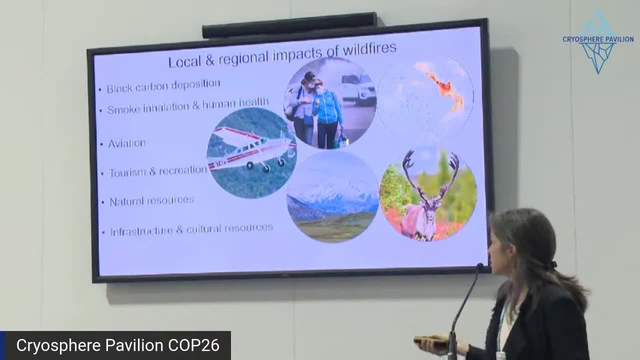 Tourism and recreation, natural resources, infrastructure, cultural resources, water quality, erosion, direct deaths, injuries, military installation. So there's a number of local and regional impacts that are really important: important economically, important culturally and important for human lives and well-being. 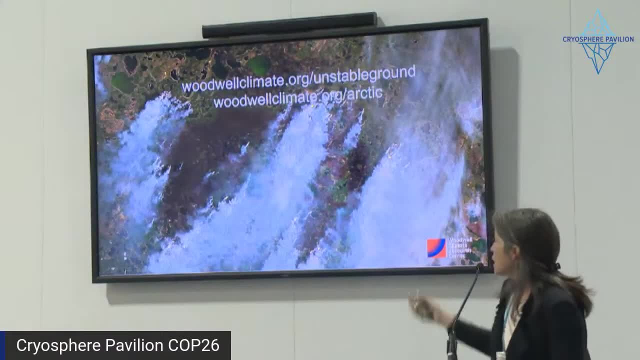 And with that I'm going to two web pages if you want to find out more information, And I'm going to pass this off to the next speaker, which is Rachel Treharne, and she will be talking about the impact of climate change. 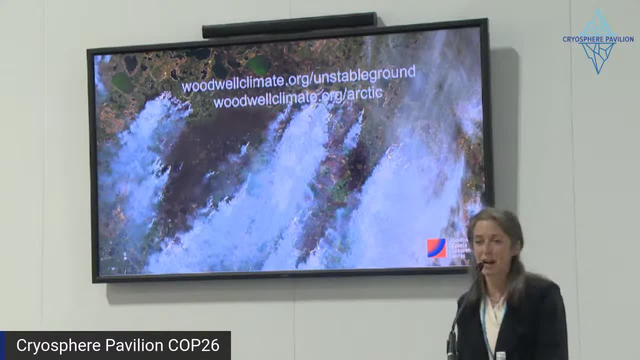 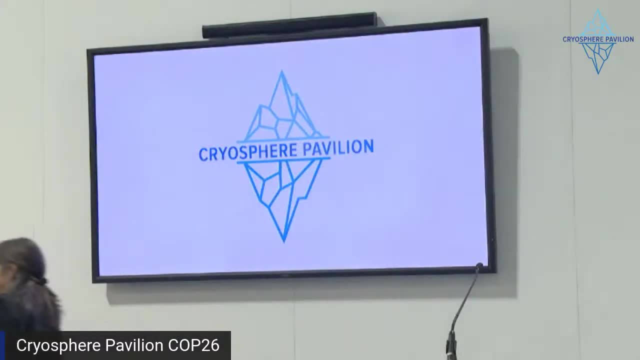 Thank you, And she will be talking about sort of future impacts of wildfires and permafrost on carbon emissions. Thank you, Hi, and thank you so much, Sue, for that fantastic overview of fires and their role across the Arctic, And thanks all of you, of course, for being here. 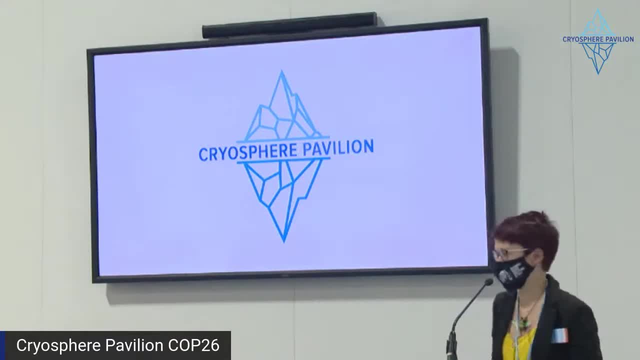 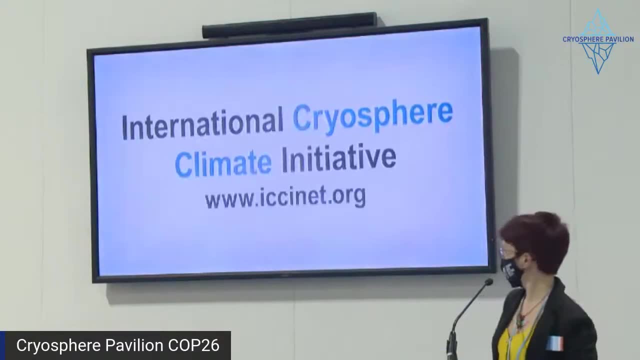 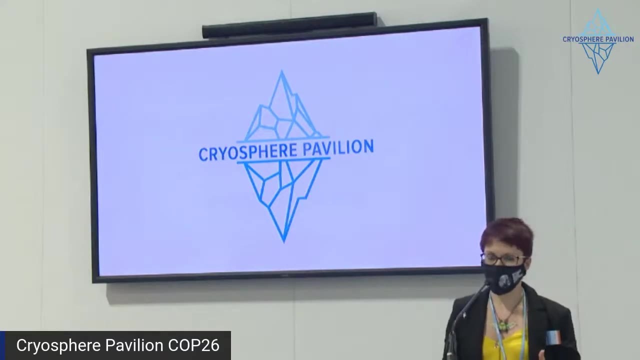 You've almost made it through the first week of COP, So that is fantastic. Thank you for joining us. And so, Oh, I broke it. but so so really. as Sue said, I'm a researcher at Woodwell Climate Research Center. 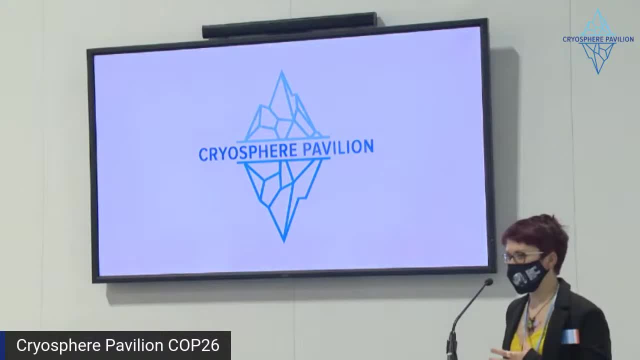 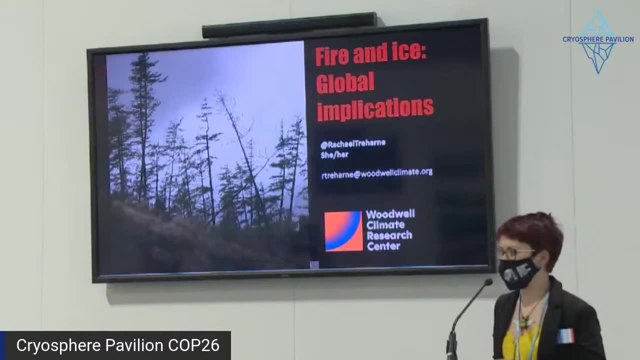 I'm interested in permafrost thought and fire and I'm going to pick up really quite directly from some of the points that Sue made about the impacts of fire in the in the Arctic, And you've heard about some of the those local and regional impacts which, of course, are really quite a broad range. 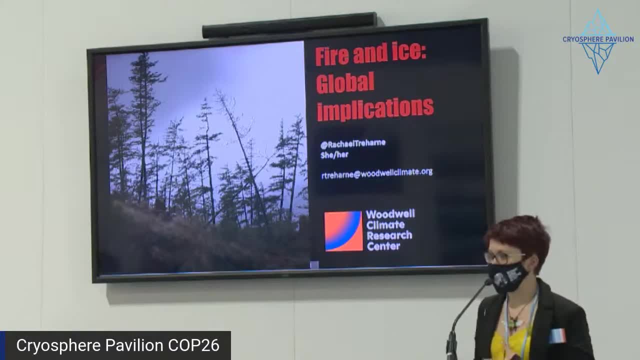 So impacted Everything really, from food security to the impacts of smoke, the impacts of smoke on human health, and we're going to delve into those and what it's like to really experience those- the panel discussion in a moment. And but we also know that, on top of these really critically important local and regional impacts, what happens in the Arctic- and that includes the impacts of fires that happen in the Arctic- really doesn't stay in the Arctic. 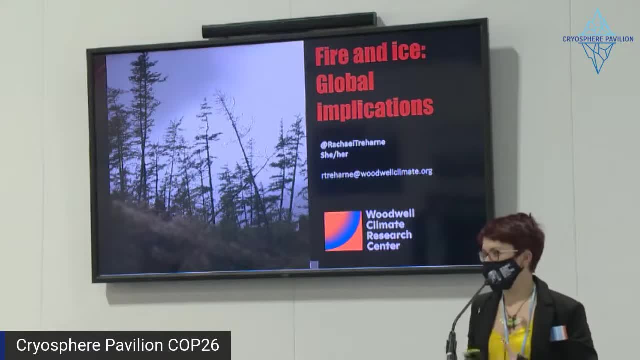 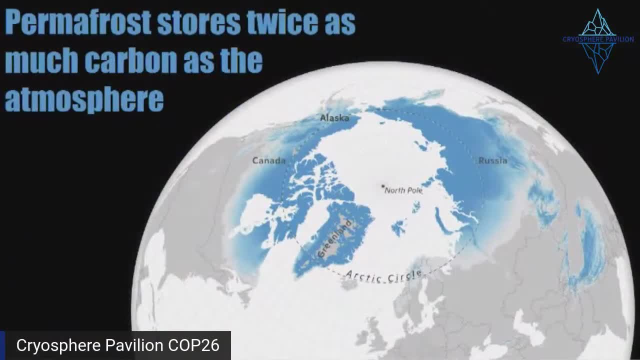 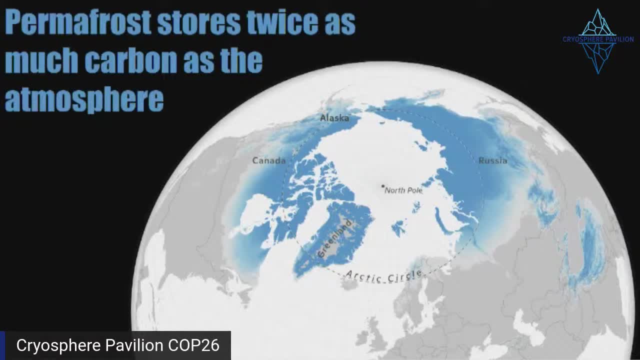 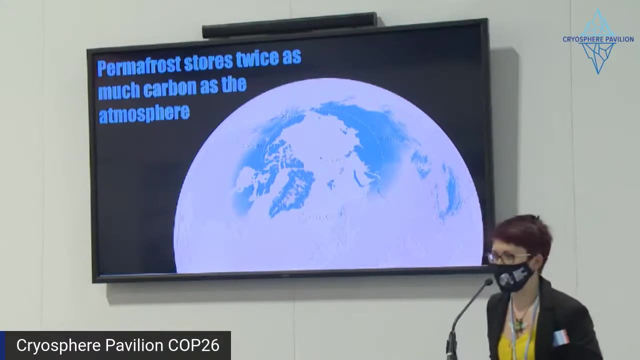 And this region, in the permafrost region. it really only covers something like 22%, so less than a quarter of the land surface, But in this comparatively quite small region this stores almost the same amount of carbon, almost twice as much carbon as there is in the entire atmosphere today. So that's. 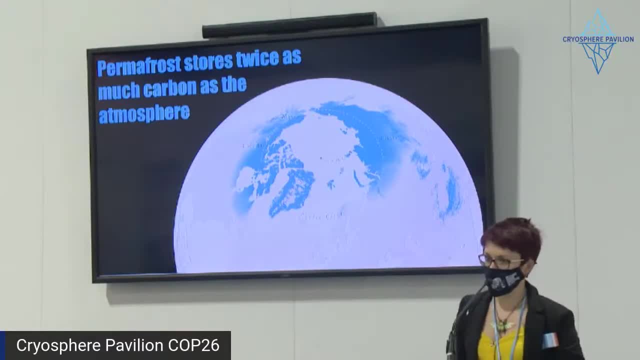 more than twice as much carbon as there is in all of the trees on the face of the planet. And, for a little bit of context, if we saw just 10% of this carbon that's stored in Arctic permafrost being released into the 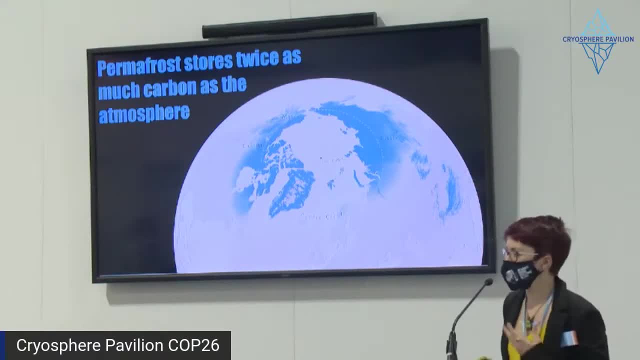 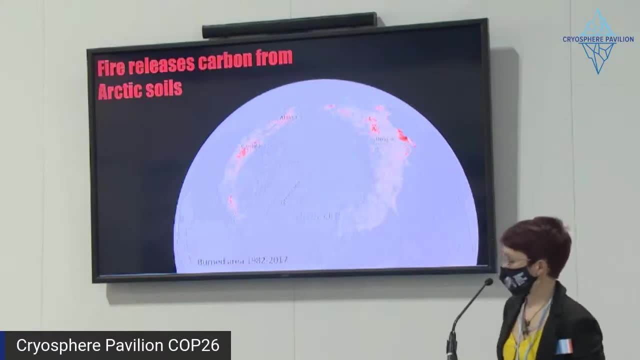 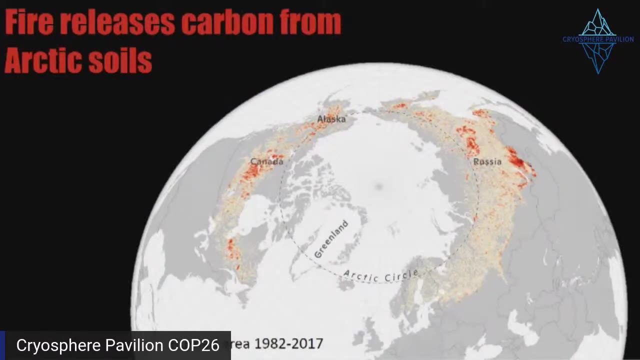 atmosphere, then we're looking at an increase in atmospheric CO2 concentrations of something like 75 parts per million. So this is it's really a pretty significant change, And, of course, one of the threats to the carbon that's stored in the permafrost in the Arctic is fire, as we've talked. 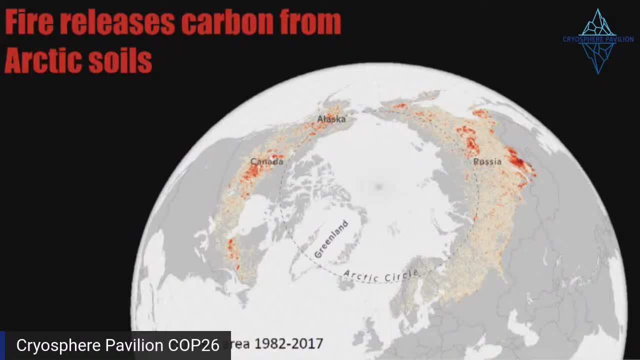 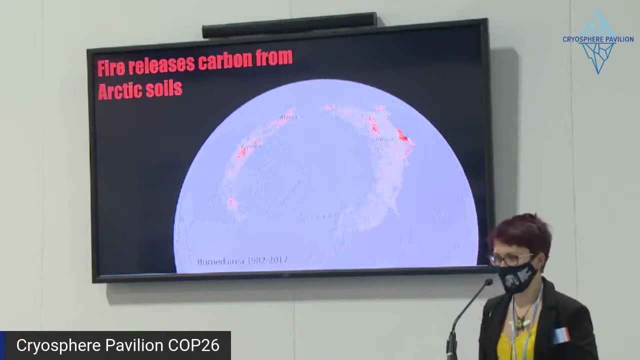 about So. again, as Sue mentioned a little bit, when the Arctic burns or northern ecosystems burn, a lot of the emissions that happen during the fire are actually coming from below the ground rather than from the burning of the vegetation itself. So we have these really deep, rich, carbon-rich soils in the 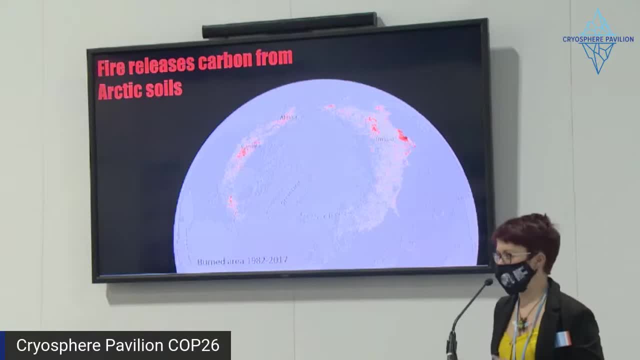 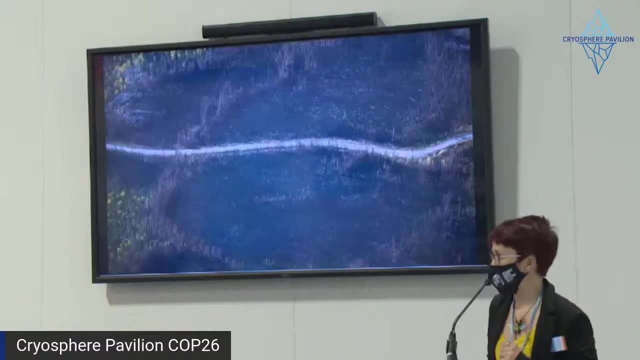 Arctic, and often those fires are smoldering away in the ground and releasing carbon that way, And on top of that there is this very close relationship between fire and permafrost thaw, And I think you can really quite intuitively see one of the main reasons that this is the case from this photo. So 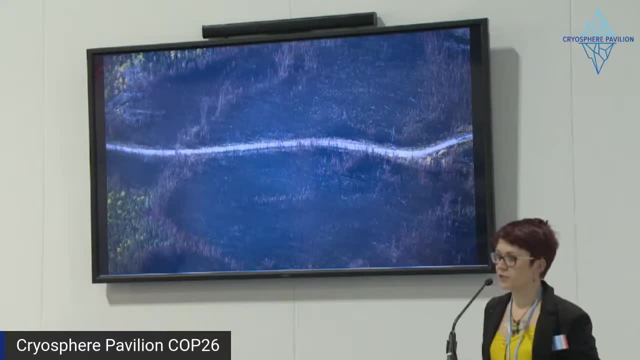 when we have these fires happen, of course you're losing the vegetation and, as well as that, you're really darkening the surface of the ground. So you've got this very dark heat-absorbing surface. So really, this is raising the temperature of the ground. It means that 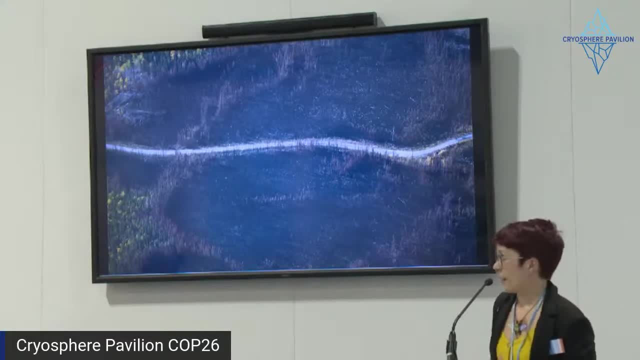 these areas are absorbing more heat down towards the permafrost And of course this means that as the ground takes up that more heat, we're looking at either an initiation or an acceleration of both gradual permafrost thaw and these more abrupt permafrost thaw processes. So just for a little bit more clarity on that. 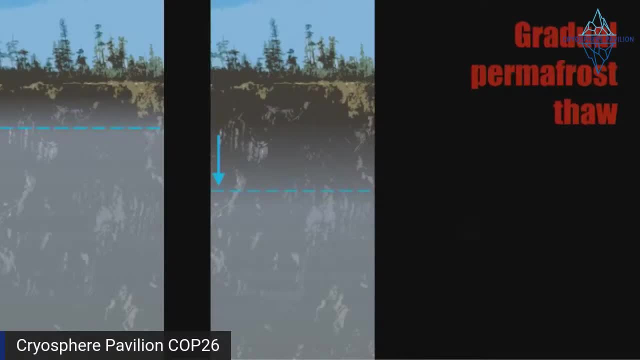 distinction. when we talk about gradual thaw, this is actually often what we're talking about. when you hear scientists or others talking about permafrost thaw, We're actually talking about gradual permafrost thaw. So this is referring to this kind of process where we see a gradual 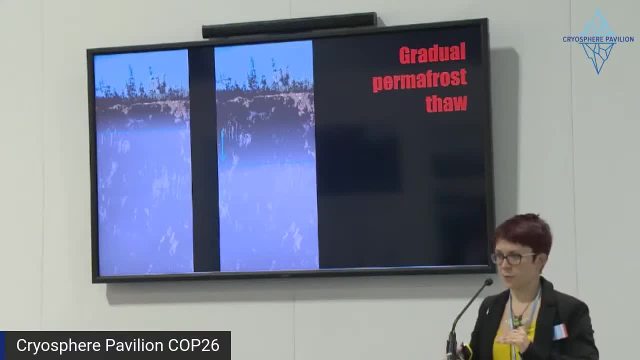 warming from the top of the ground, basically a grading down the surface of the permafrost. So it's this kind of centimeter by centimeter, year by year process. I mean this is the dominant sort of source of permafrost. 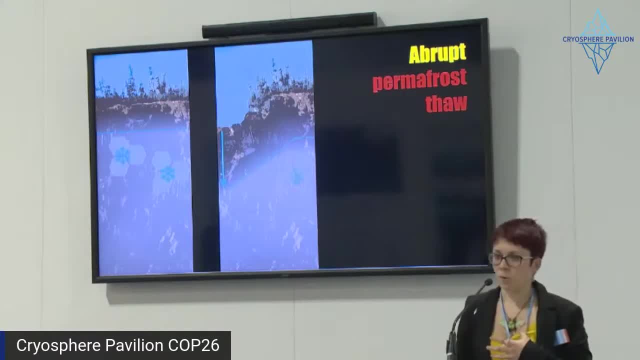 thaw, but it is not the only one, So we also see what I'm calling here abrupt thaw. Abrupt thaw is actually kind of an umbrella term for a lot of different processes. If you were able to catch Jens' talk earlier about deep carbon in permafrost and some of the ways that that is made vulnerable, these are: 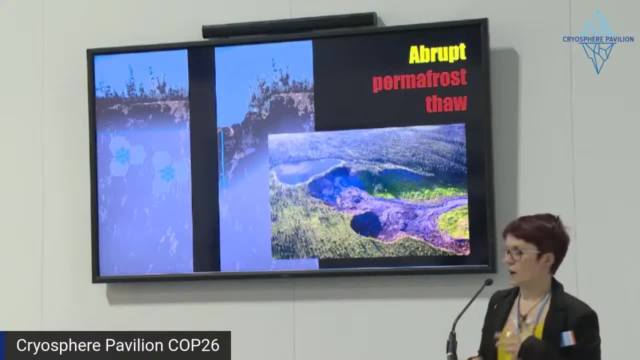 the kind of processes we're talking about here, So slumps and kind of large scale landscape changes that you often see in pictures like this one. And this is a process that happens, perhaps affects a smaller area, but it can affect several meters of carbon really quite rapidly. 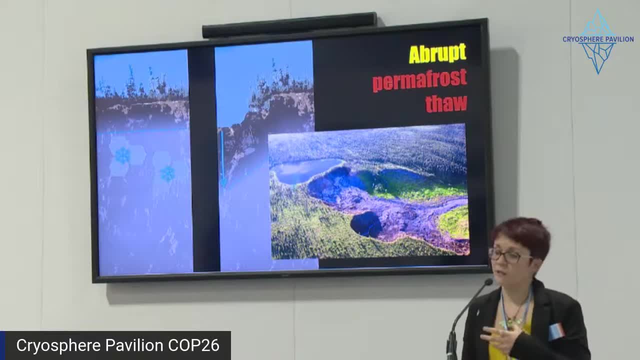 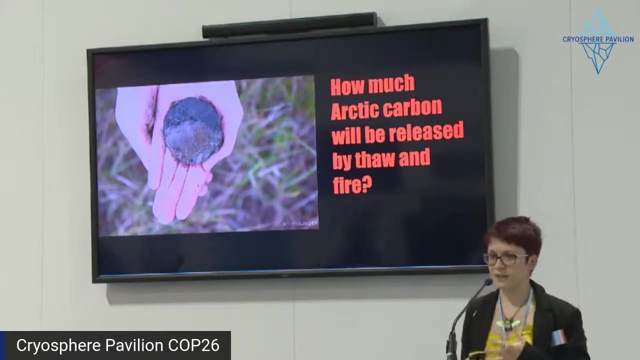 So these are processes that can be taking place on the time scale of years or even days, as opposed to that kind of gradual, consistent, slower process of gradual thaw. So we've talked about these processes. we talked about carbon released from fires and its effects on permafrost thaw. 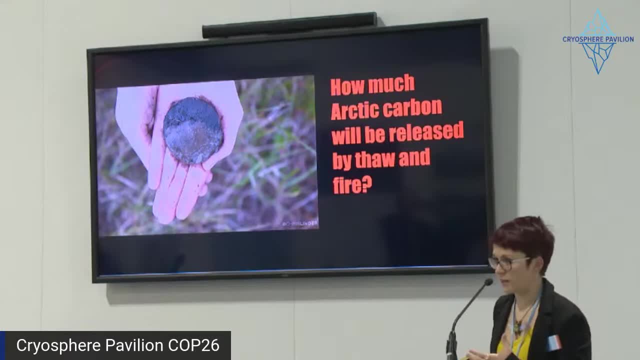 And then the question quite clearly for permafrost scientists and for fire scientists is how much carbon will be released from this, from this store in the arctic? and i'm gonna do the classic sort of researcher move here of talking about why this question is so hard to answer, rather than trying to directly go into the answer. 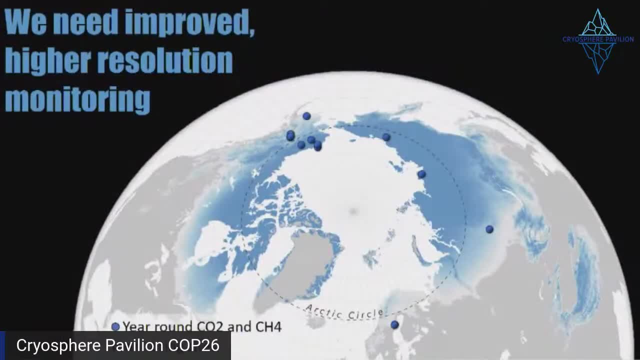 and the first reason there is is perhaps a little bit intuitive. so we know the arctic it's not just one place, it's a huge region, it's enormously variable, even over quite small spatial scales, and it's it's fairly sparsely populated. parts of it are quite inaccessible, and the outcome of that 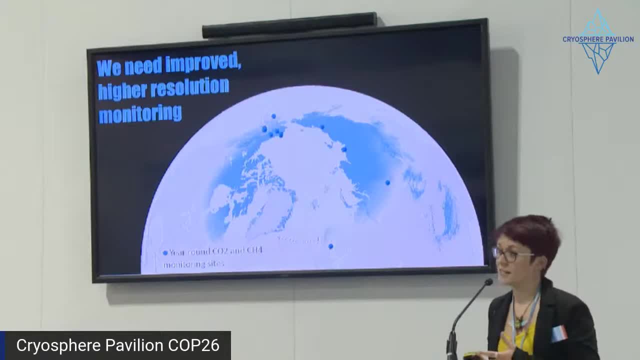 is that we don't have um the data that we ideally would like, and just to kind of highlight that, this is um the map you've seen already showing permafrost extent, but on top of that we plotted the locations of monitoring sites that are recording uh, carbon dioxide and methane fluxes. 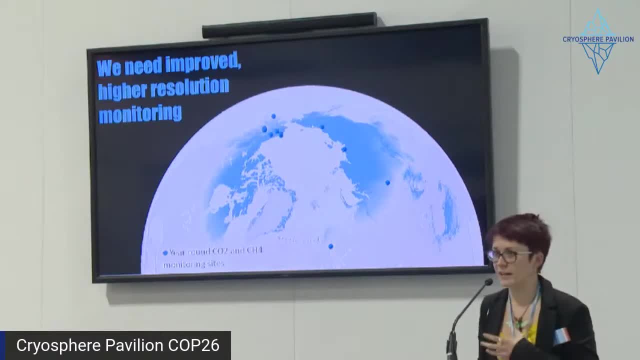 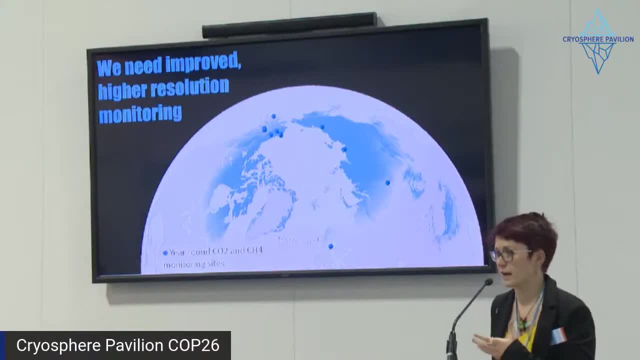 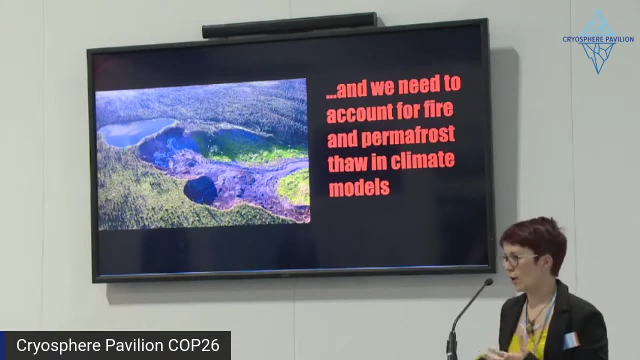 large parts of the arctic, but really flying blind um, trying to try and trying to understand what is happening here. the second reason is that we're really actually only beginning to try and account for some of these processes in climate models and in the policy tools that are developed from climate models, and this is something that sue um. 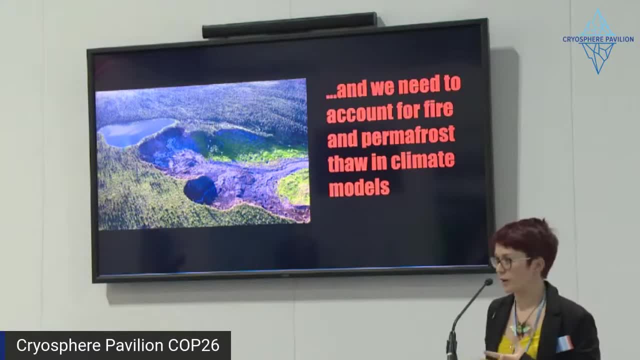 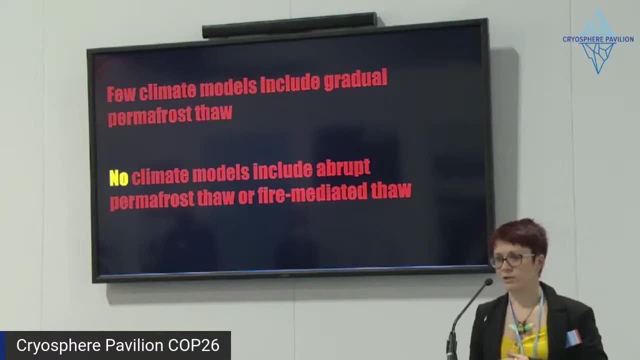 touched on as as well, and this is something that we're working on- quite a lot of woodwell at the moment. so at the moment, the situation is that a very small minority of climate models include anything to do with permafrost carbon at all. i think it's something, something like four uh models that are 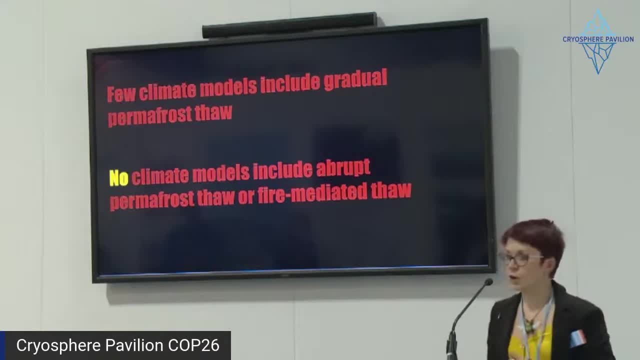 out there that that attempt to to look at permafrost carbon and no climate models at all currently include these other processes. so none of those are including the release of carbon from below the ground as a result of fires across the arctic. none of them are including those are more abrupt. 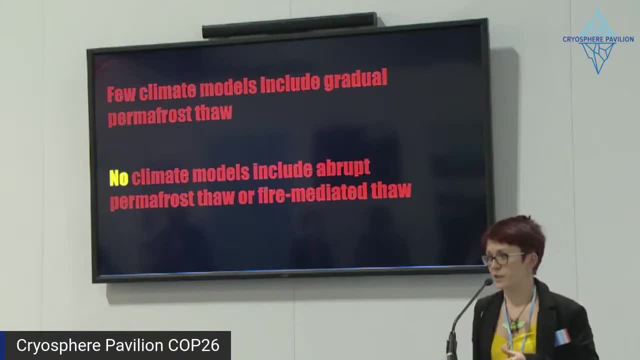 permafrost thaw processes, and none of them are including the interaction between those two things, which, of course, we know is something really important and that will become more important as we see those fire regimes continue to intensify across the arctic boreal zone, and so this is something, as i mentioned, that we're working on at the moment. there are a couple of uh. micro dose test distribution units which are figuring out what's happening in the future to kind of top each other. you know what? okay, so that's a handshake, i think very creative. what's happening this is a type of thing. we're honesty is that we've gotholic that option, as you can'tlles on and farmers come in and tomatoes and then buy a bunch ofč. 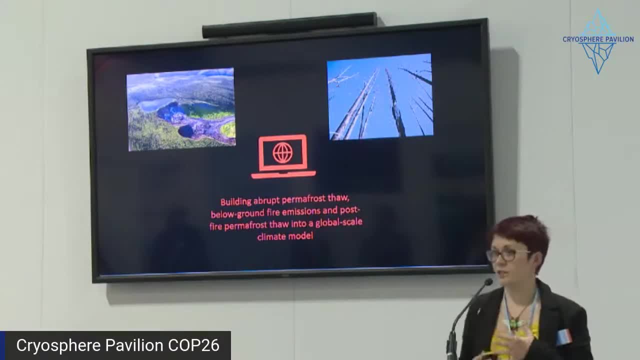 mentioned that we're working on at the moment, um, and one of the ways that we're doing that is some work i'm doing and this is taking a kind of a reduced complexity earth system model, so essentially a simplified climate model, and we're having a kind of first stab of putting some of 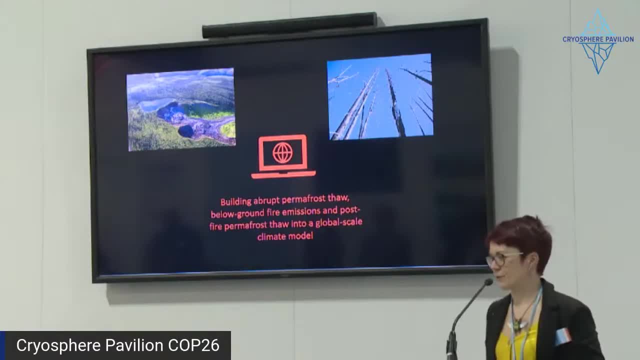 those processes into this model, um sort of in in the face of those challenges related to data and things like that i've mentioned mentioned already, and so this is- this is work in progress. this is not something that we've got to the stage of publication or peer review, but of course i 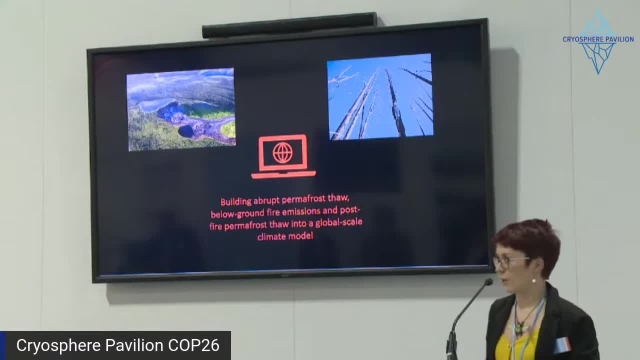 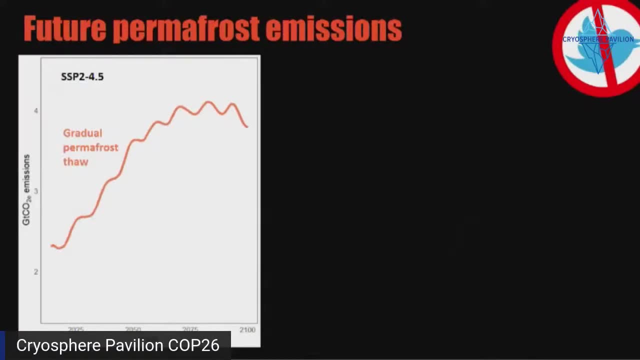 did want to try and give you a bit of flavor of what those outcomes might look like, and so what you're looking at here is, uh, one example of a sort of possible future of emissions from gradual permafrost thor, and this is under a pretty moderate warming scenario. we're looking at rtp 4.5. 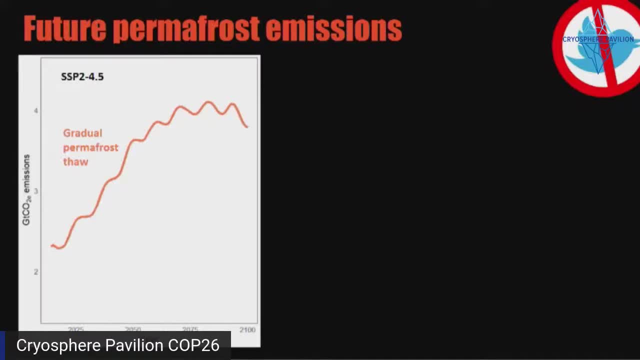 and this is um emissions from about the present day out to the end of this century. and, in contrast, if we kind of use this updated climate model, we have to rerun this scenario and look at the emissions that we expect to see from those other processes we've talked about. so from fire, from fire mediated thor and abrupt. 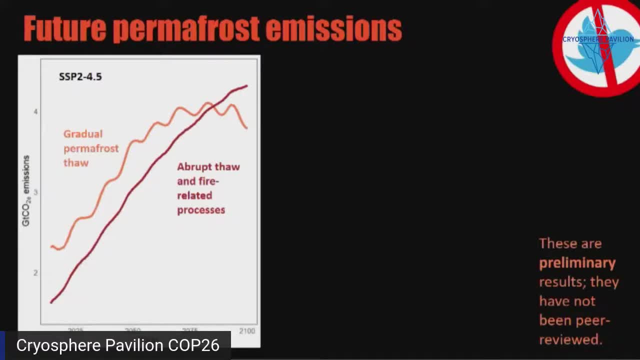 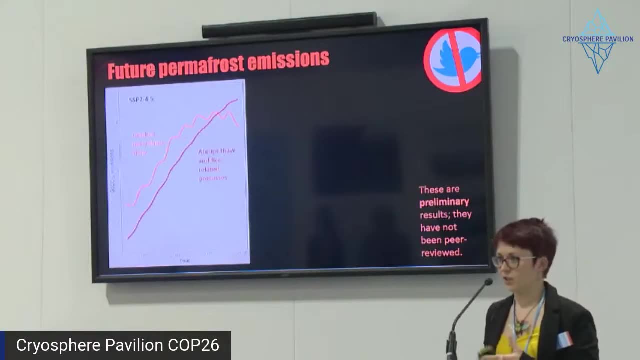 thor. um, this is what that looks like, so you can see that this is um, really something that is on the same scale by itself as gradual thor, which is the process that we tend to um to tend to focus on, and even when we look at a much more extreme warming scenario. so rtp. 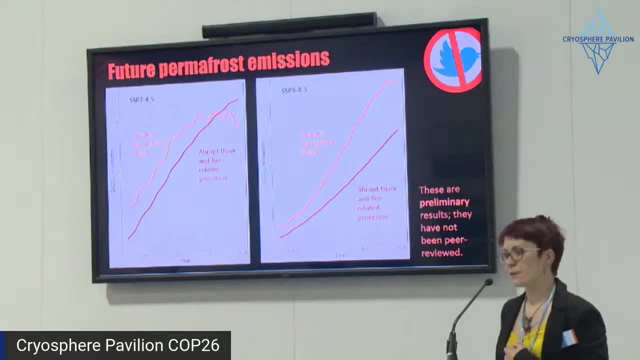 5.5, where we know we expect to see much more widespread gradual thor. even then we see that these underrepresented processes, which again are not included in any climate models, um, are really of a similar scale and for a little bit more context here, um, this is the emissions from the eu. 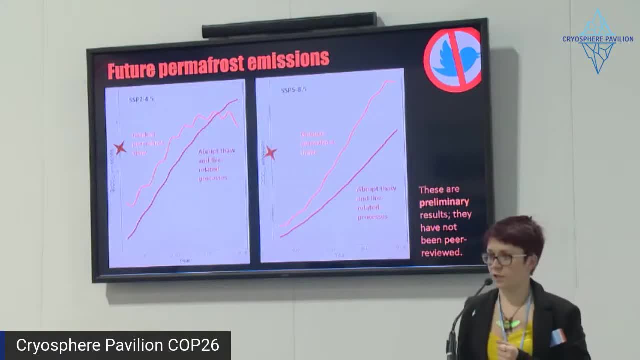 in 2017 um, and these are the emissions from the from the us um in 2017. so really, what this is kind of suggesting is that if we continue to to leave these processes out of climate models, we continue to leave them out of our carbon budgets. 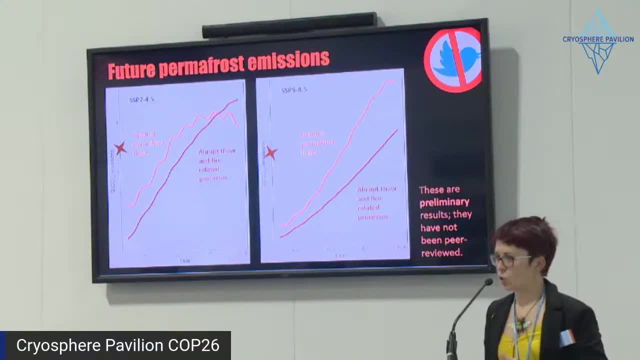 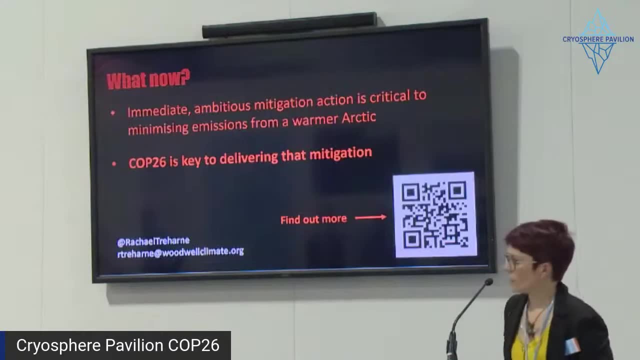 and therefore out of these policy debates, what we're essentially doing is ignoring the contribution of something equivalent to a major economy by the end of this century. so what do we do with this information? of course we're all here at cop and the obvious message really is just to kind of increase that urgency of mitigation. 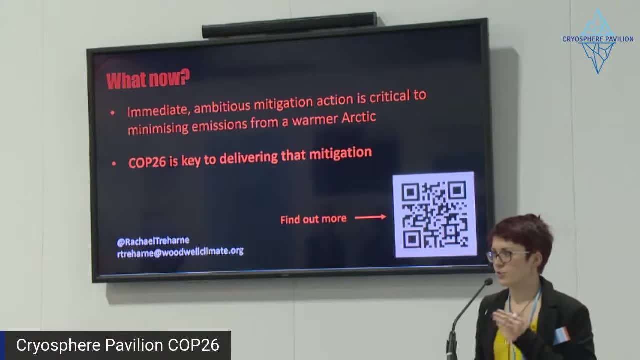 um, we all know that the window of opportunity to reach the paris agreement goals, to reach those goals of one and a half and two degrees is is closing and really what this suggests is that that window is potentially closing even faster than we think, and i think what we all need to 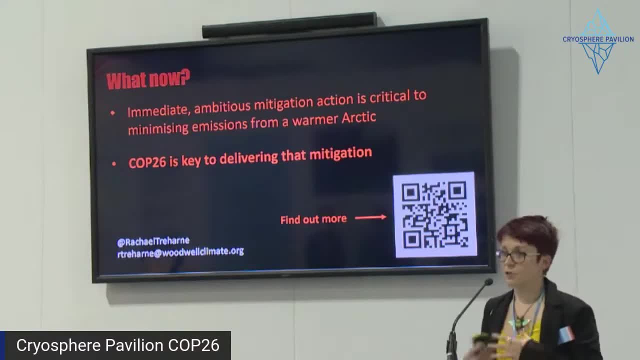 keep in mind is that these numbers that we talk about, our carbon budgets, the future warming we expect in response to different, in response to different scenarios, these things are not safety nets. uh, we know that there are processes out there that are not included in those things and we know 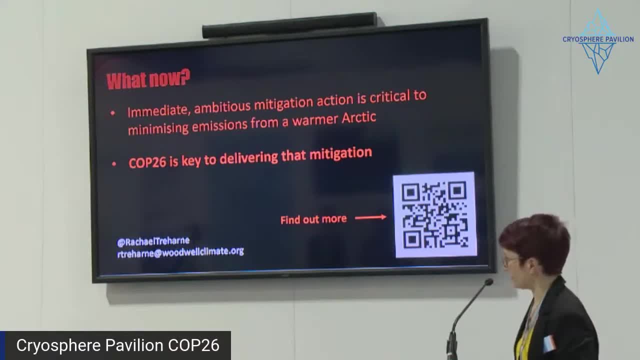 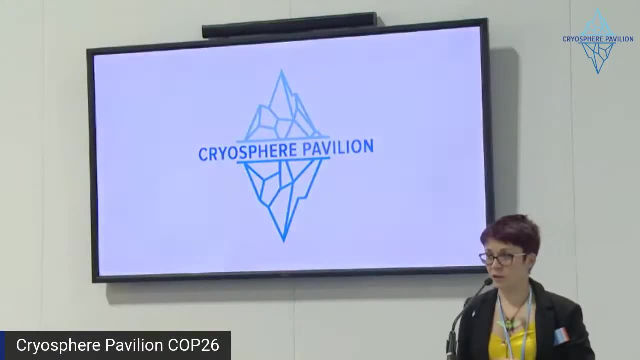 and we've seen here that at least some of those are substantial sources of emissions. um, and so with that, um, i think, uh, we will be moving on to our panel, um, and i'd like to, as we sort of prepare that, give a quick plug. if you're interested in these issues, of course, um, ask. 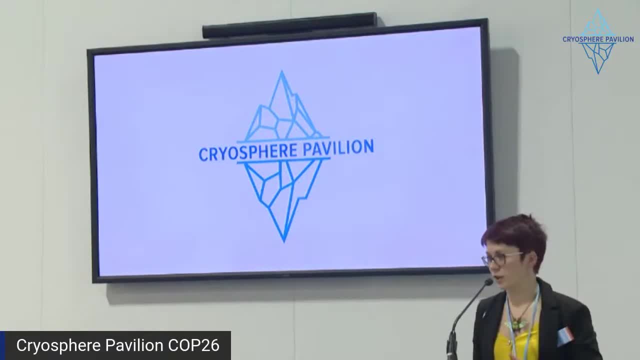 questions and stick around and talk to us, and also on the front desk, we've got a lot more information, um, and some briefings and also some little qr codes, which will take you to a platform where you can look at some of this data and play around with it and find out a lot more background about these. 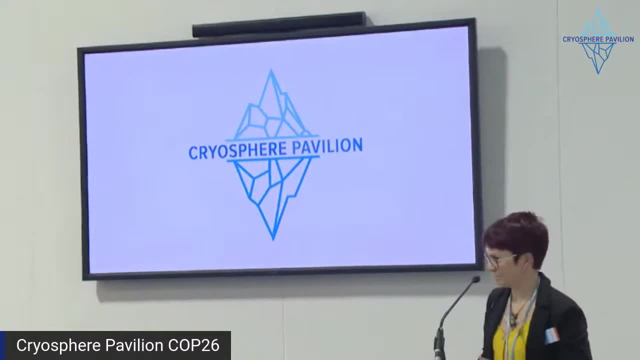 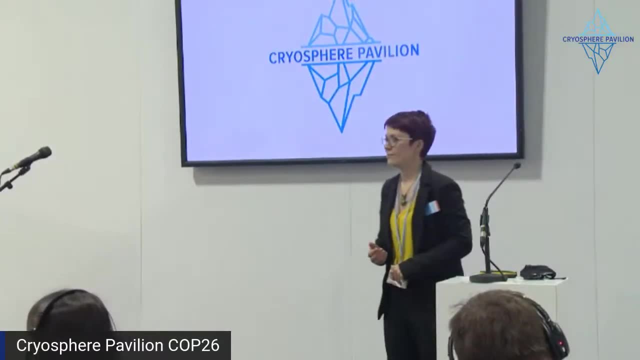 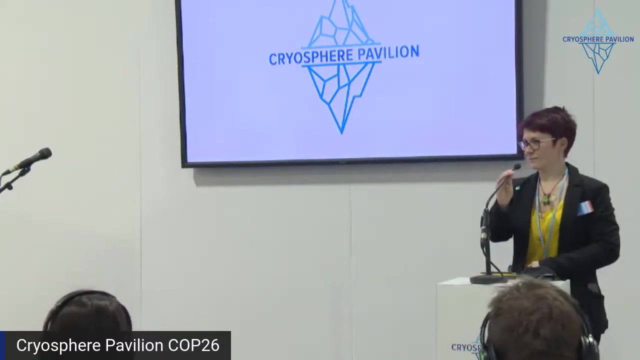 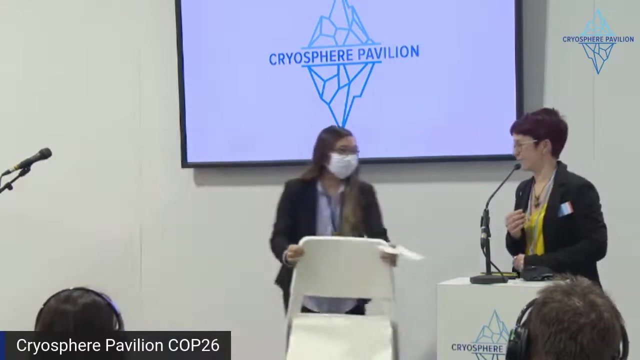 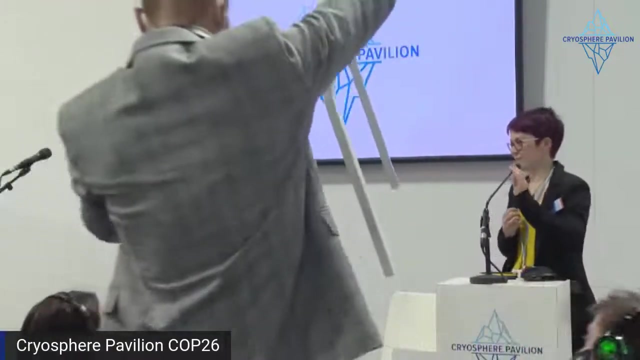 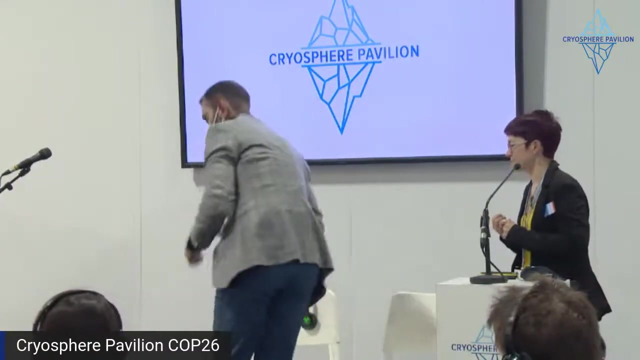 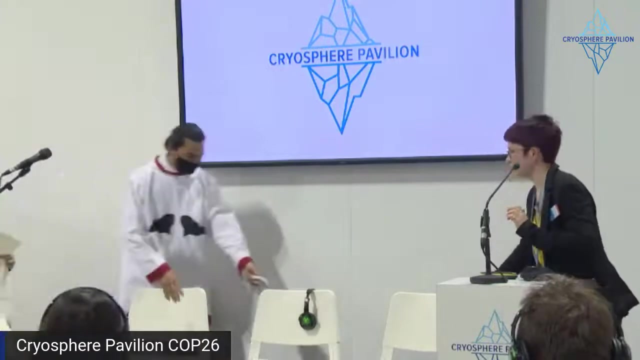 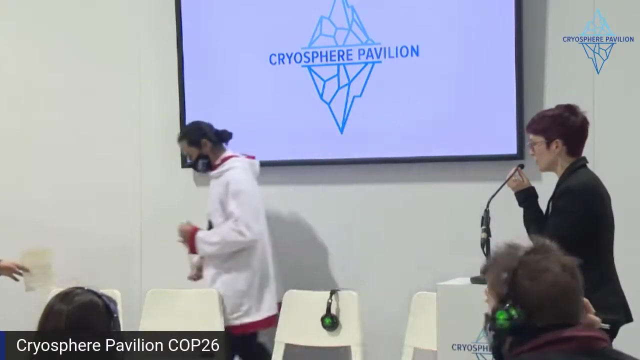 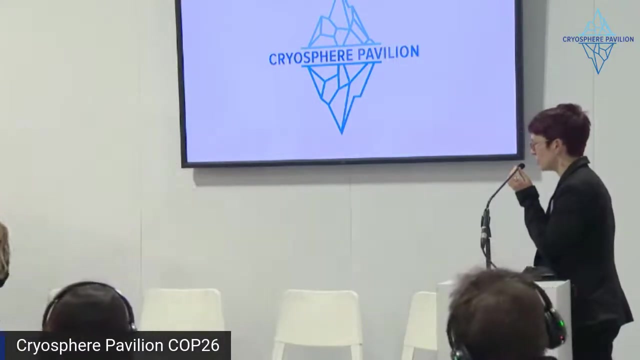 issues. thank you, and i think we'll move on to our panel. you They will introduce themselves in a moment, but we are really lucky to be joined by Darcy Peter, my colleague from Woodwell, and by Jill McClark from Vivo Barefoot, and also. 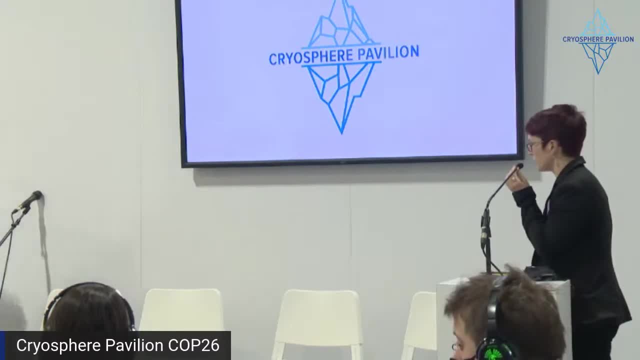 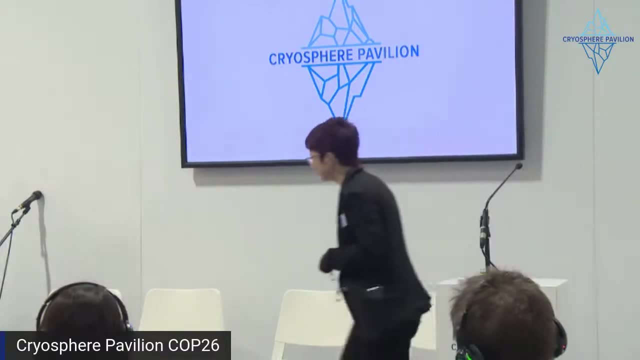 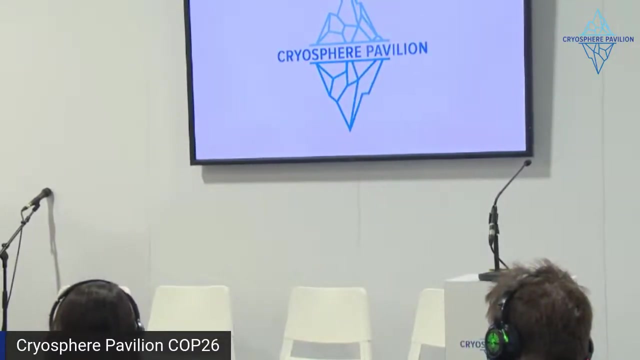 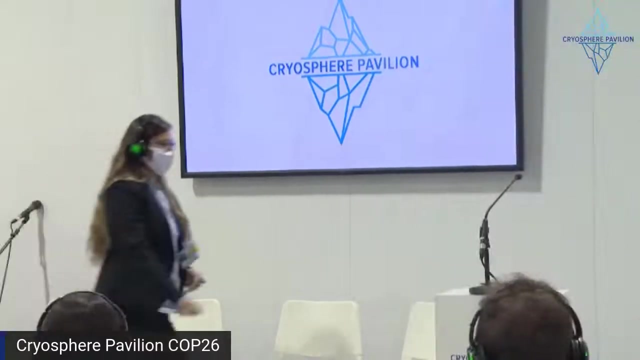 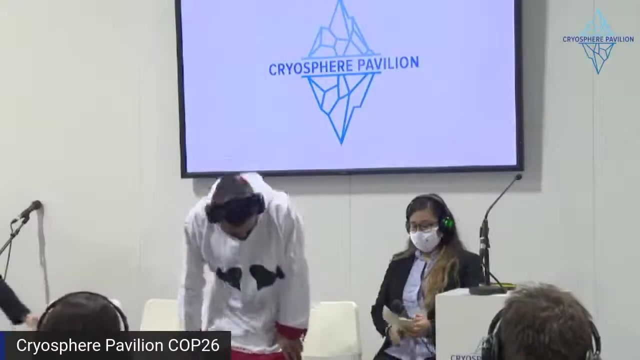 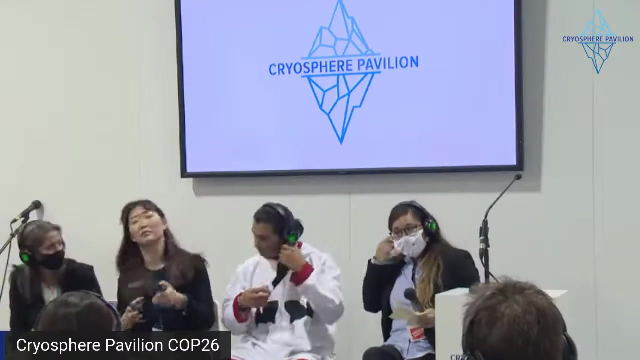 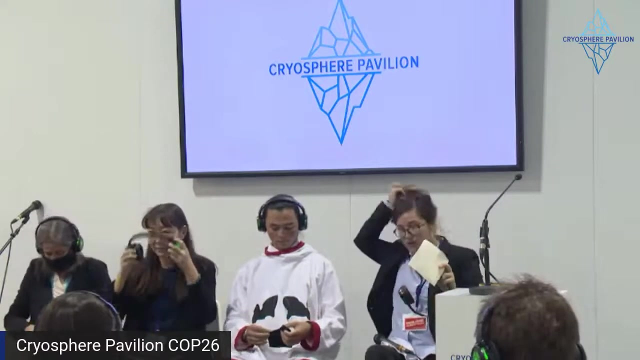 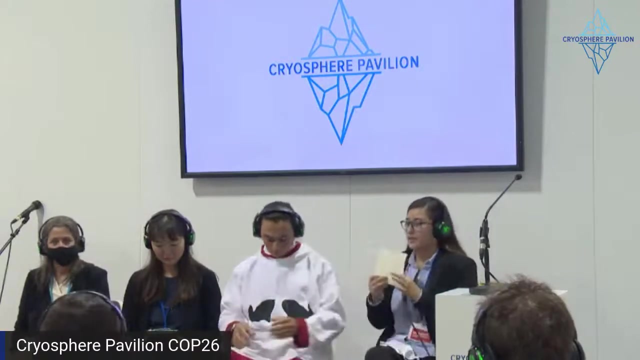 by Sam, who's also going to be telling us about some of the impacts that we're seeing from these processes on the ground, And this panel is going to be moderated by Sue Natale. Yeah, thank you All. right, drink winzy everybody. good afternoon. 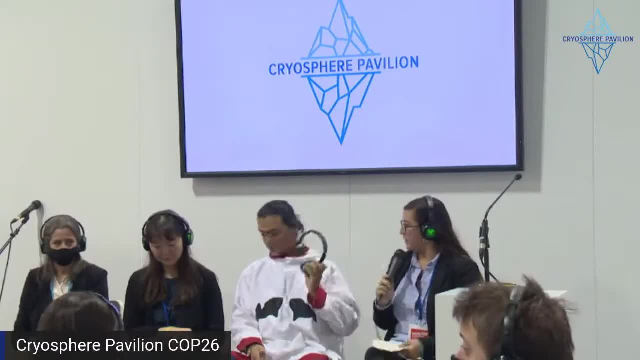 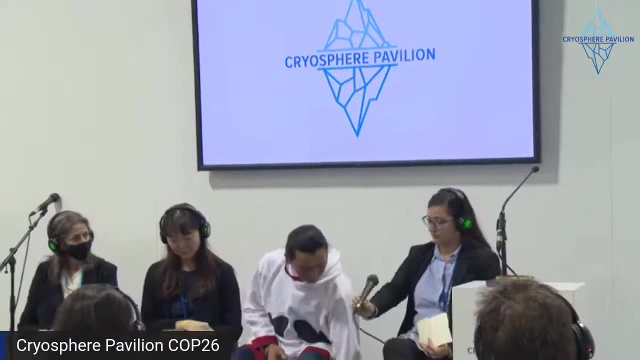 My name is Darcy Peter and I'll be moderating right now, and I just want to open the floor to Dolma. Sam and Sue already introduced herself, so if you two want to introduce yourself, that'd be awesome. My name is Sam Schimmel. 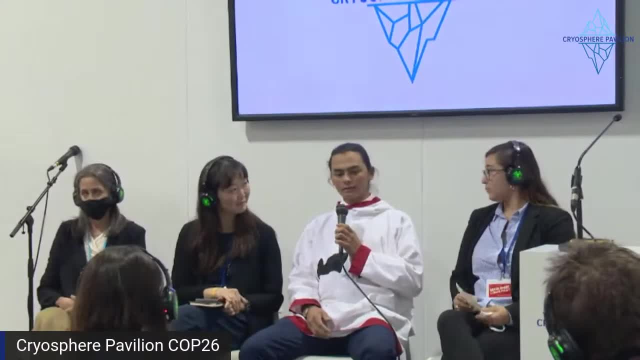 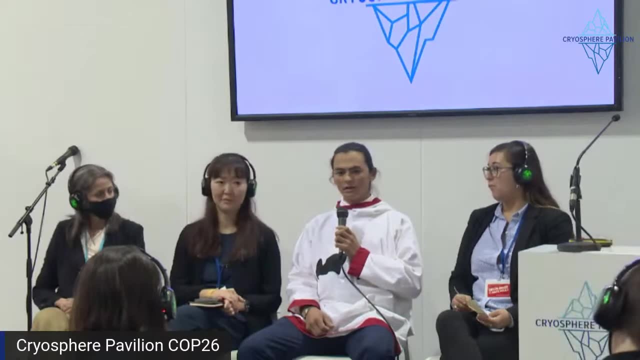 I'm Kenaitse, Indian and Siberian Yupik. I'm from Gamble, Alaska. My community is one that sits in the middle of the Bering Sea, in its northern region, and I come from a subsistence community where all of our food comes from our ocean. 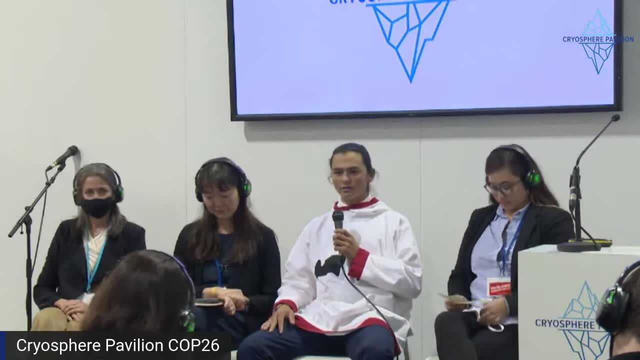 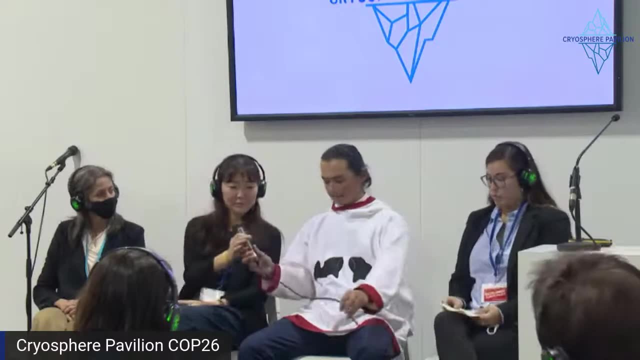 It comes from our land and it comes from the resources that are around us. So I'm really happy to be here with you all today and excited to see what comes out of this panel. Hi, Hi, I'm also good at I can do the greetings in my- yeah. 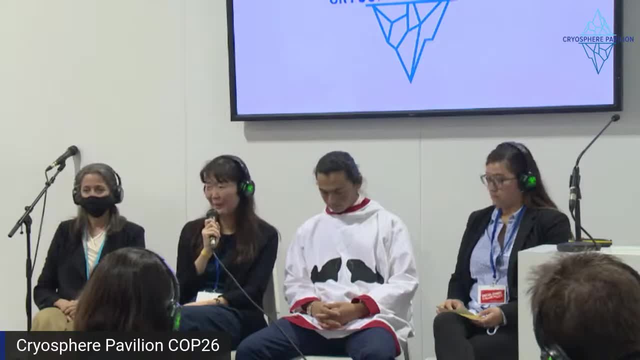 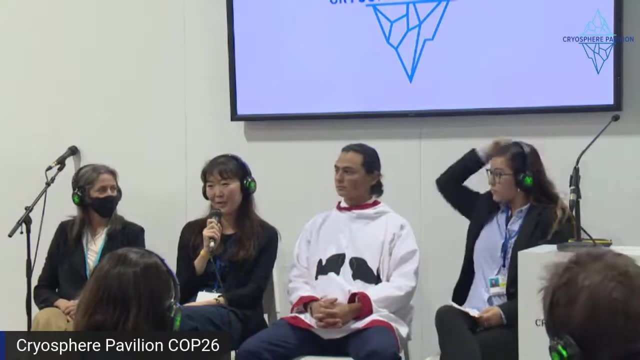 Indigenous language, Sambana. I'm. I'm coming from Siberia, from Lake Baikal. It's not that north or not part of the Arctic region, but my community is already suffering from what you've seen so far, and I'm here to share the story. 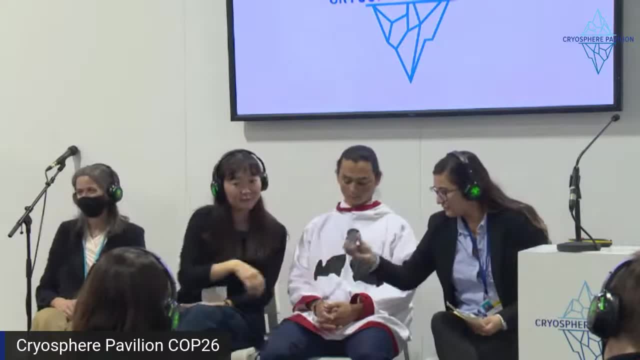 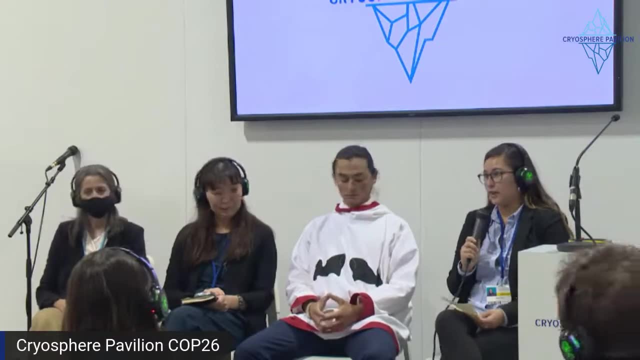 Thank you. Yeah, so I'm Darcy Peter. For those of you who weren't here at the last panel, I am Koyakon and Gwich'in Athabaskan from the remote village of Beaver, Alaska in the US. 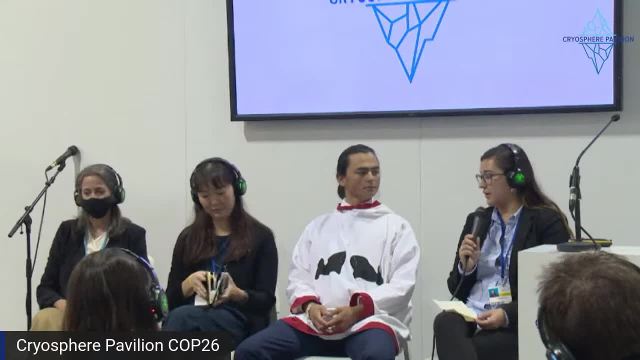 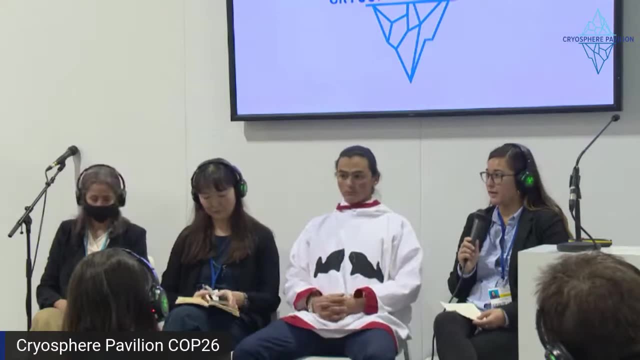 It's located about four miles below the Arctic Circle. There are 30 people who reside there year round, and we also practice a subsistent way of life- hunting, fishing and trapping- and everything that we collect is used and put into our freezers. 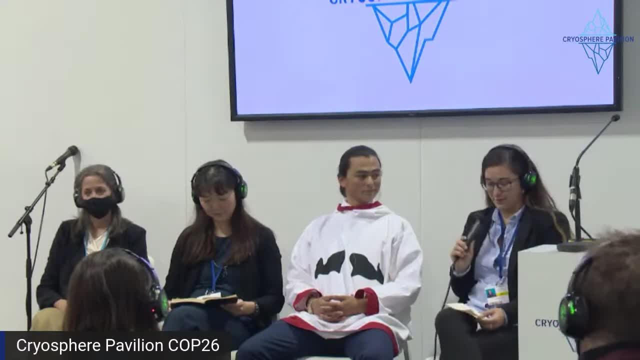 Yeah, so thank you all for being here and thank you, Sue, for your talk. It was awesome. I think I want to kind of shift gears here and ask Sam and Dolma what some of the climate changes you've seen in your communities. 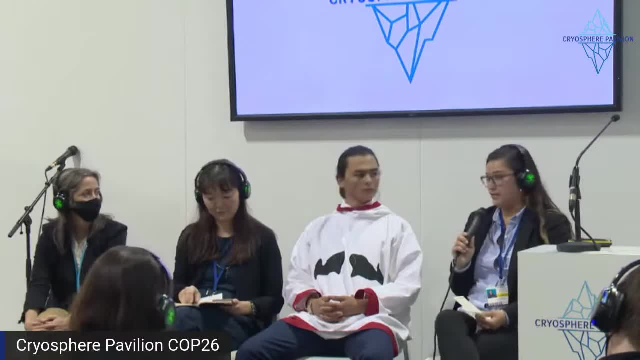 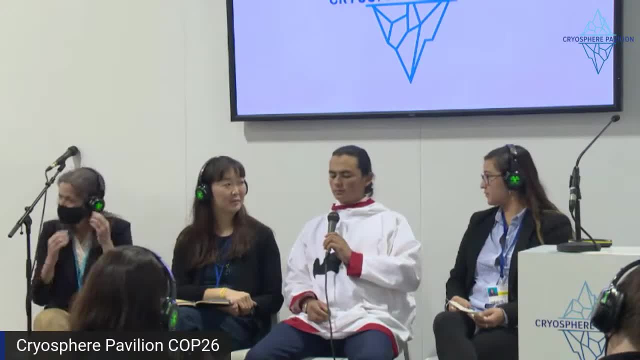 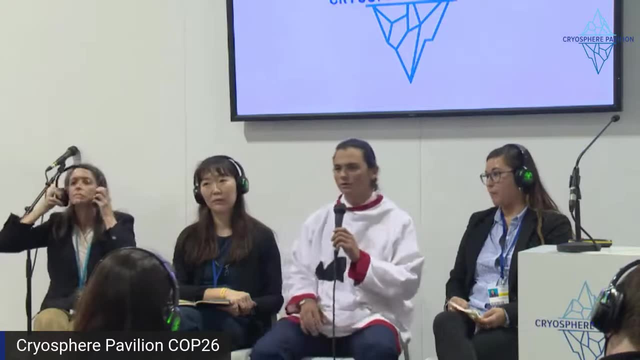 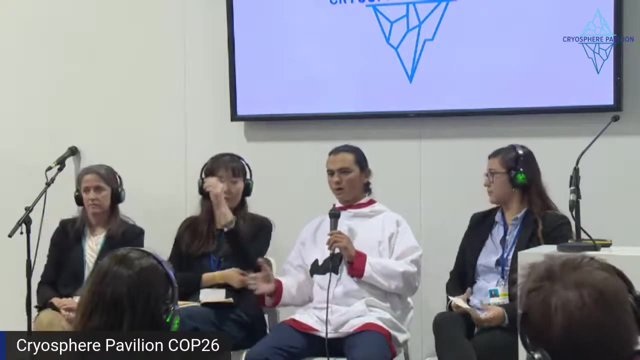 Well, thank you, Darcy. I don't know where all of you here come from, but I would venture that each of you lives in a place where there's a grocery store, that whatever's on your table at the end of the day or at the beginning of the day, is something that you purchased, that you bought. 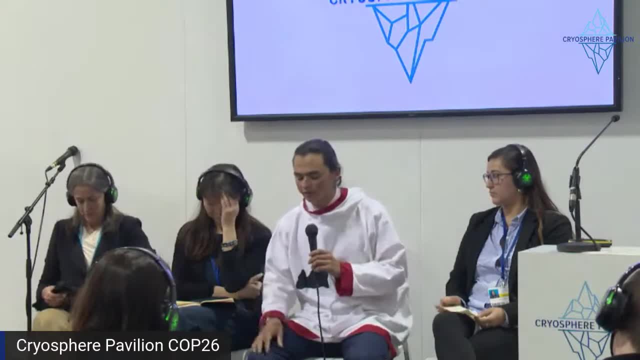 It's not something that was caught or that you had to go catch. It's not something that you bought. It's not something that you know had to go catch. For our subsistence communities in Alaska and around the world it's a very different. 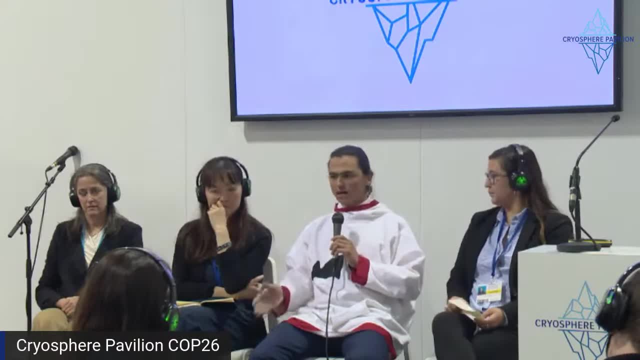 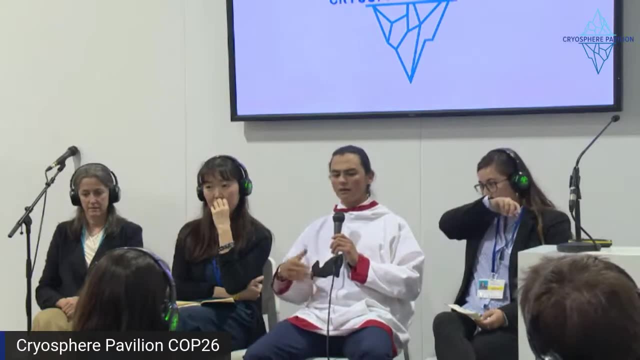 reality. Our food that we eat on a daily basis is not something that we buy from a store. It's something that we go out and we harvest and we catch. This means that our diet of marine mammals- things like whales, seal, walrus- is critical. 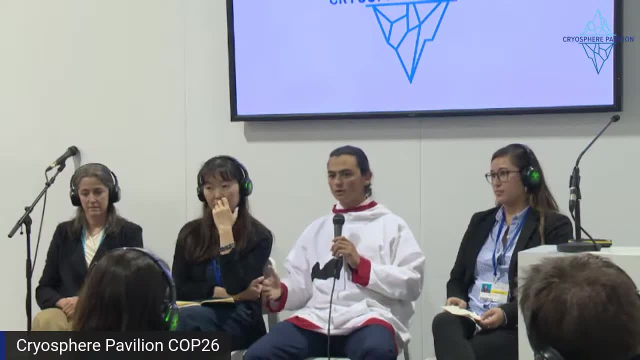 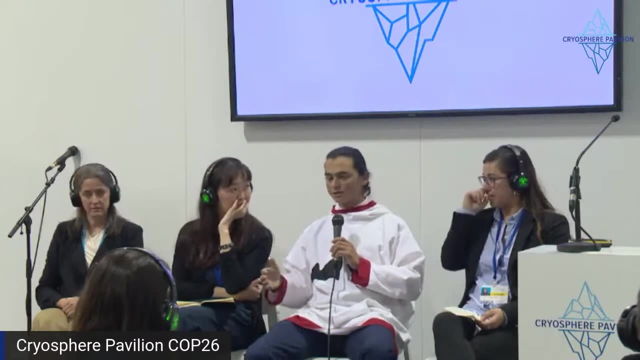 for our communities. In our communities, we don't have grocery stores. We have incredibly high rates of food, We have incredibly high rates of unemployment, and things that you can buy from our village stores, which are very understocked, are incredibly expensive. 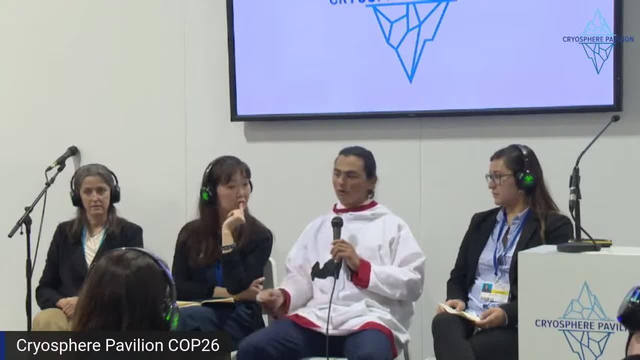 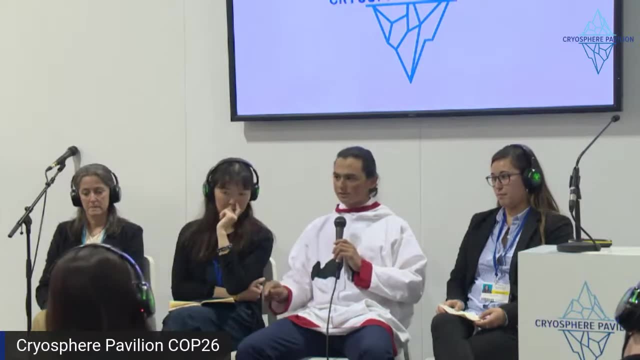 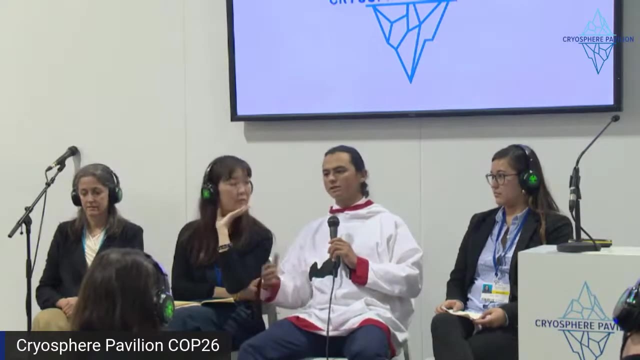 Things like a gallon of milk might cost you $12 there, where it may only cost a dollar or two dollars here. We rely very heavily on our subsistence animals and subsistence foods to survive With climate change. we're watching those subsistence stocks change. 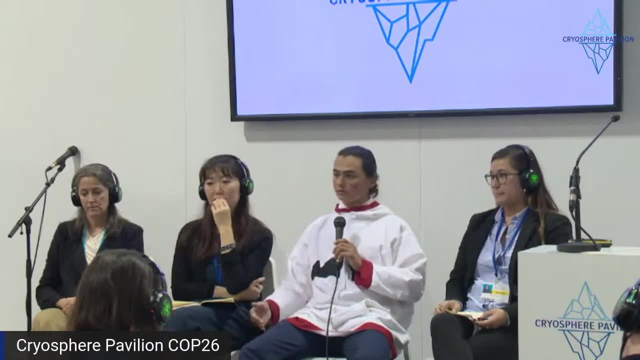 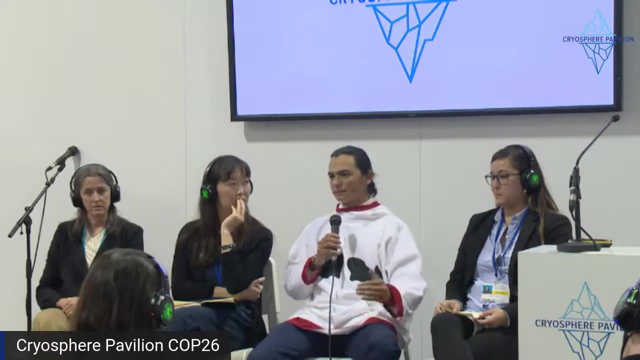 We're seeing our animals come later in the year. We're seeing the reality that where I'm from in the Bering Straits, we're no longer having sea ice in the wintertime. Sea ice is one of the critical things for walrus to be able to calve. 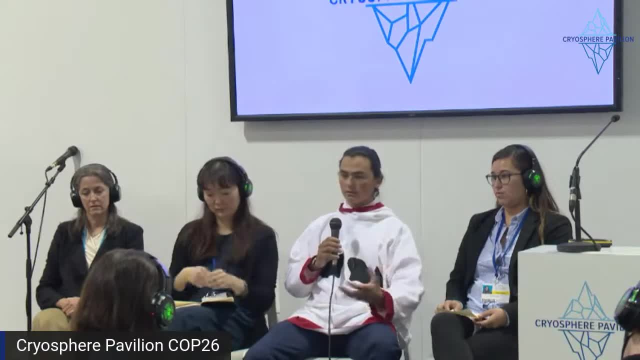 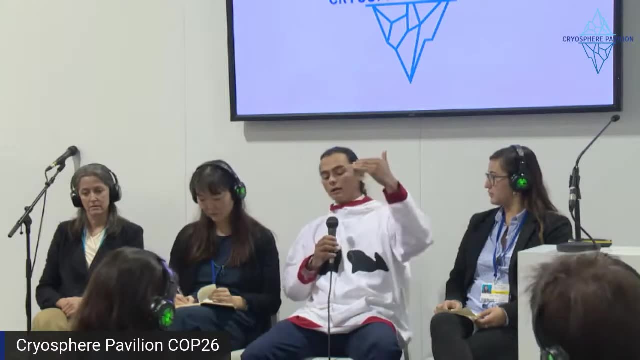 When walrus give birth, they can't do it in the water. They have to do it on ice. They don't like going on the land either. They have to do it on the ice. What's happening is, as that ice is moving further and further north, those walrus aren't. 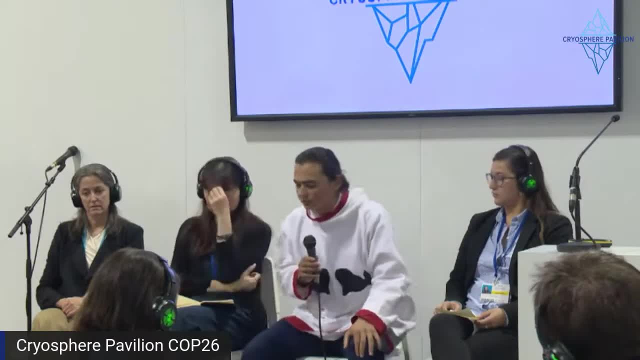 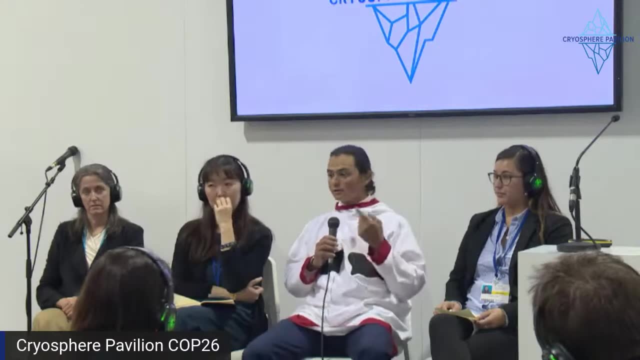 able to stay in those places because the water is too deep for them to dive down and catch their own food. When it comes to climate-related impacts to subsistence, we're watching our subsistence resources that we've relied on since time immemorial are being diminished. 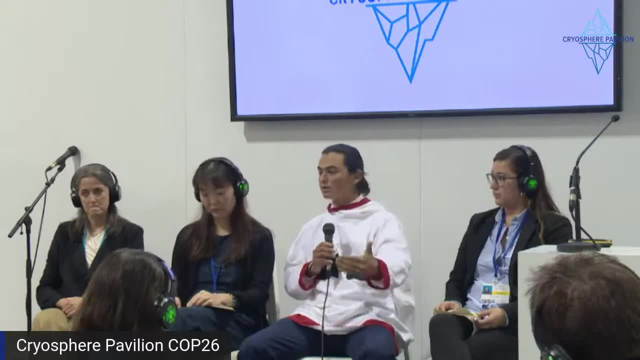 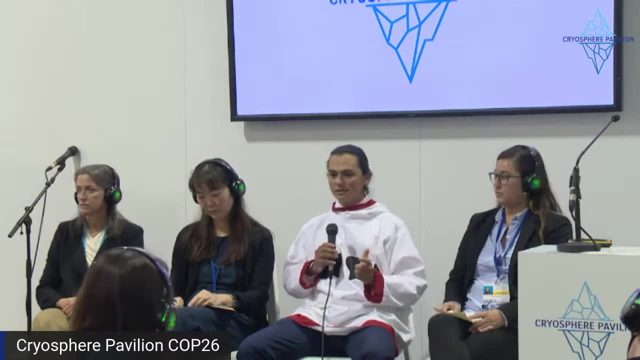 They're slowly- and in some cases very quickly- moving out of our reach. This means that there is immediate food security needs that are being laid to bear by climate change. It means that there's immediate nutritional needs as a result of these animals being malnourished. 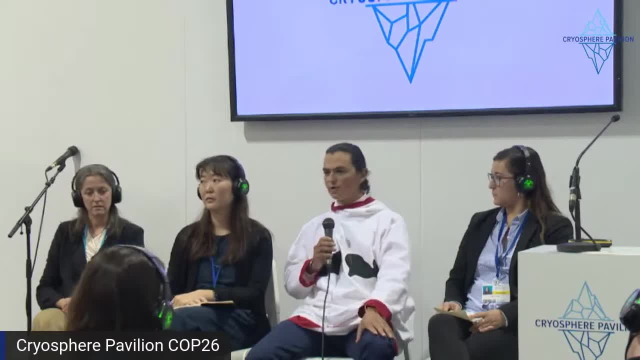 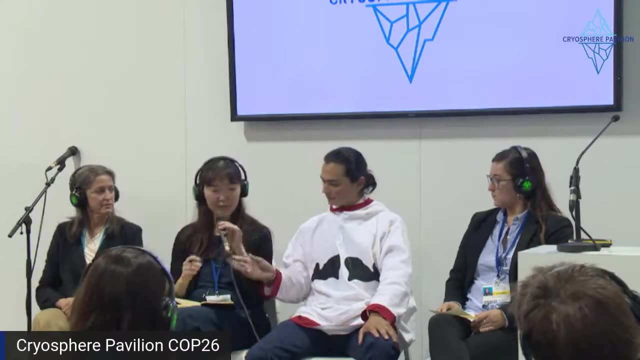 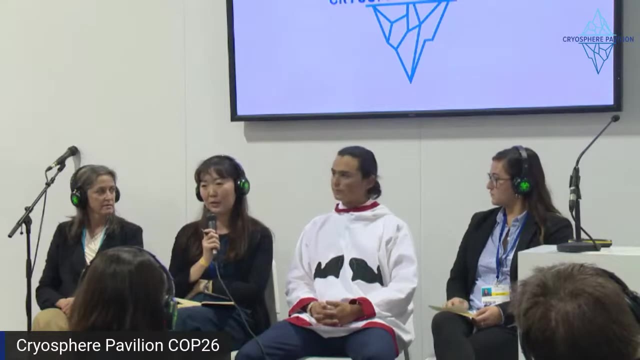 that are present. It means that there is a plethora of issues that are coming our way, Thank you. I come from a really small community, from Lake Baikal. we've been the first indigenous people that basically settled there. Originally, we came from Mongolian side of the border and 800 years ago we got settled. 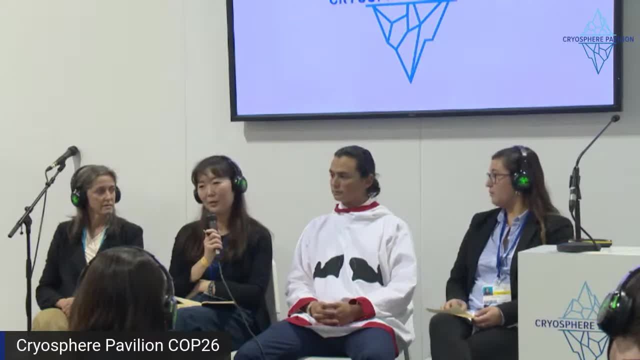 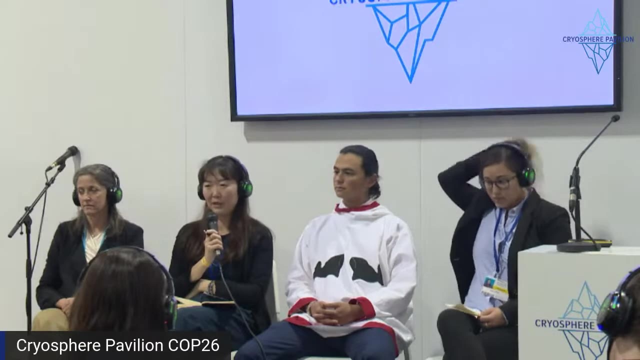 My family was born and raised in the Kesinbara in a tiny community of like 200 people doing subsistence farming all day long and herding, herding the animals and basically watering the plants all entire my childhood and i haven't been since i moved to britain as a human rights lawyer and social business. 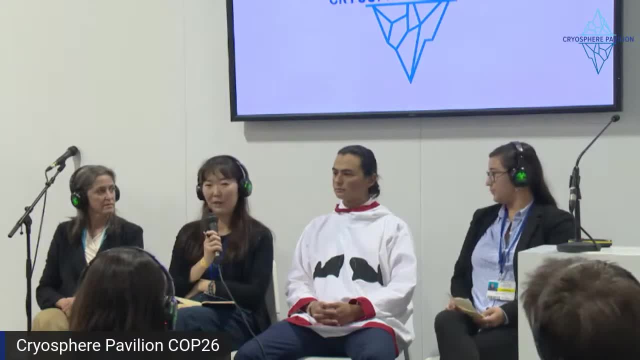 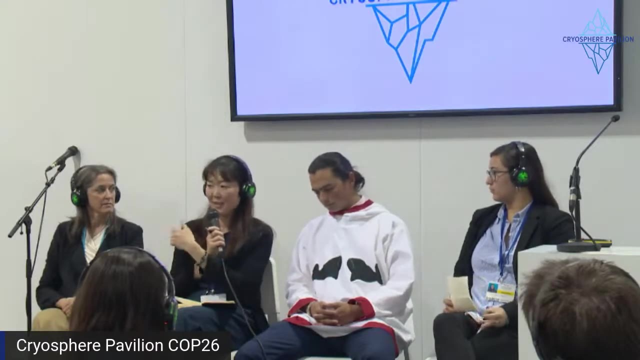 sort of entrepreneur, i suppose. i haven't been home for for a while, so i took my kids for the first time in five years this summer. we arrived in august and we end up in um, basically almost like in the quarantine. when we arrived and we landed, i saw what looks like- looked like a fog. 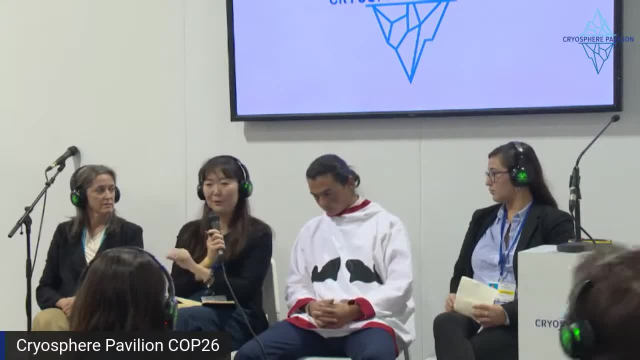 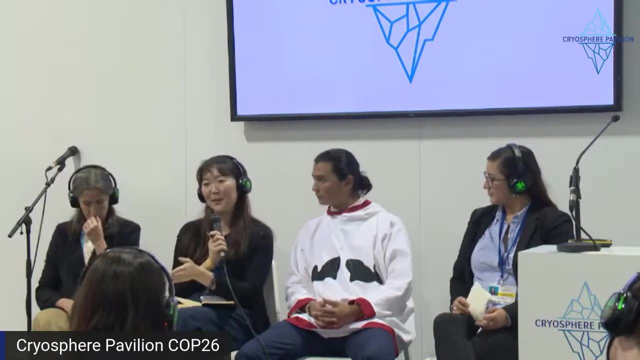 and was so dense and i couldn't work out like- and normally we don't get this kind of fogs like that- i'm thinking, wow, like what the hell? what's going on? and then they open the door. it's actually smoke. smoke that came from the north, even if the epicenter of the fire was like. 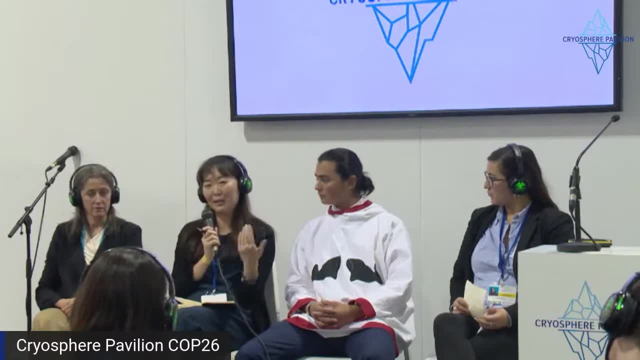 probably 2 000 kilometers away. imagine how shocking it is when you land. you get that. i was reading about it on the news, etc. but i kind of never really um thought it's gonna like you're gonna land in the middle of a environmental emergency. so then, uh, for 10 days we stayed at 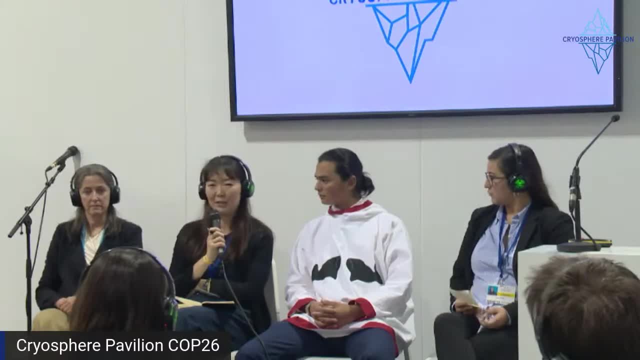 home couldn't get anywhere and it's quite obviously it's devastating. this is my family, it lives there and then for many, many generations, um, everything was super predictive, like everything is super functional. everybody knows when. when do we need to plant? um the plants, and when do we need to. 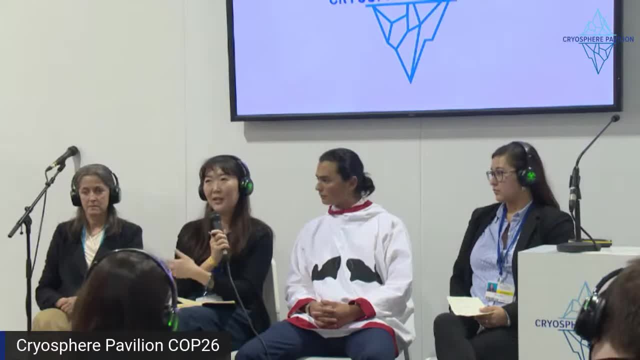 harvest, etc. like all this knowledge has been passed on through many generations was like, so organic and now we get the, the lightnings which we never did that we really had before, like in um. it's very dangerous. like nobody actually trained, nobody knows how, like you know when you're gonna be hit. 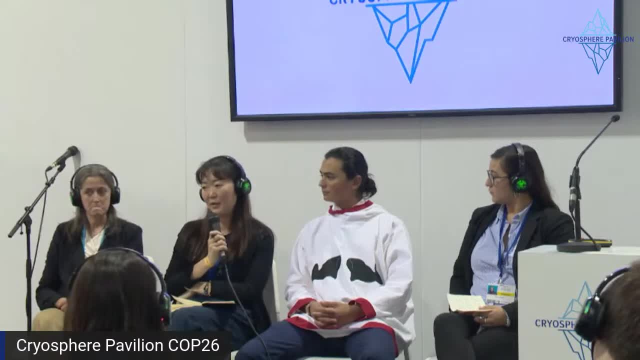 or whatever. so i think there's a whole like awareness that needs to happen. the second thing is around the flash flooding and then the NDTT and the the uh um, i really uh had that like at this uh scale, and then obviously temperatures are changing and it's extremely scary. 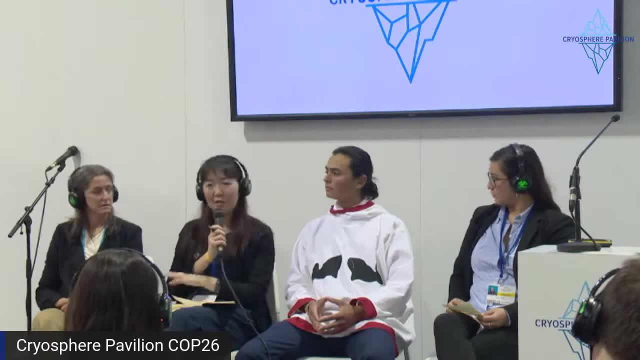 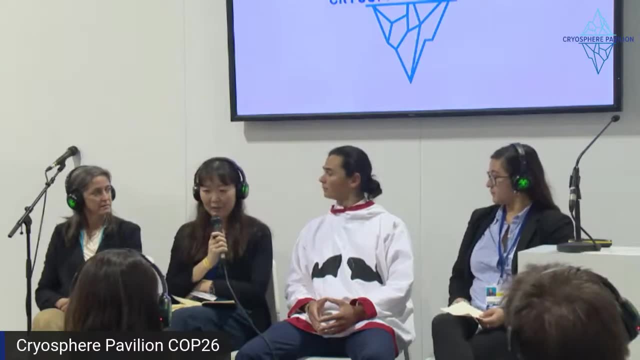 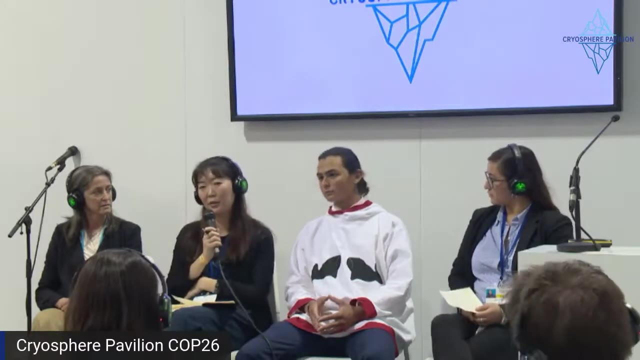 most relevant one for today is the Sami community, and then I can share that project, maybe a bit later. So I'm here with our family company called Vivo Barefoot. we actually have a stand at the UNFCCC pavilion and we're launching this vision of regenerative footwear. So we've been working. 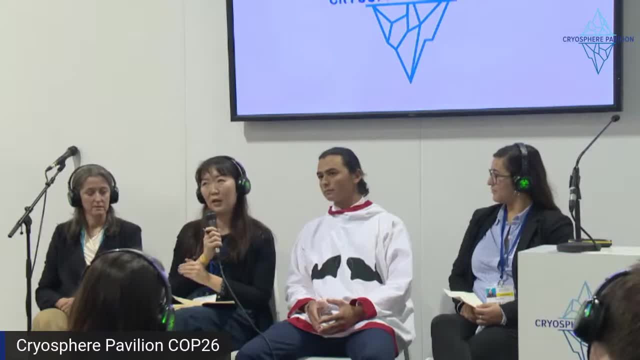 on this project for the past 10 years with scientists, anthropologists, with biomechanic scientists, and the theory is that currently the way how we produce and consume is obviously so disconnected from how we used to do everything foot by foot, from localized materials like 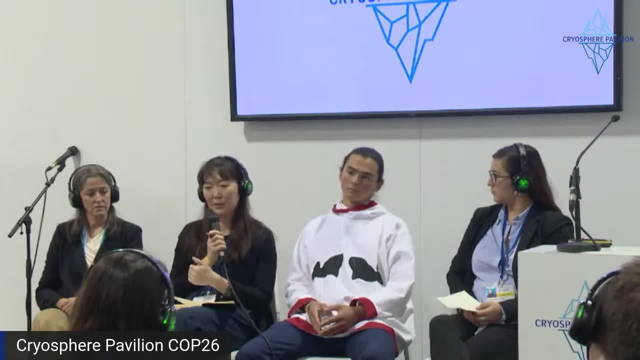 thousands of years ago, when everything was extremely regenerative, localized and sustainable. So we went back to the Sami community, to the San Johansi community in the Kalahari desert, to learn how we can recreate this logic and the way to manufacture and the way to produce things but also make it regenerative. 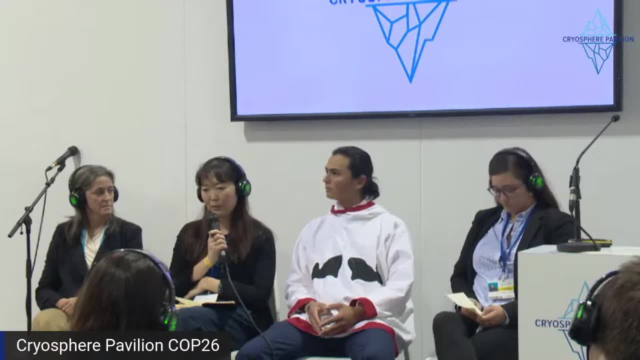 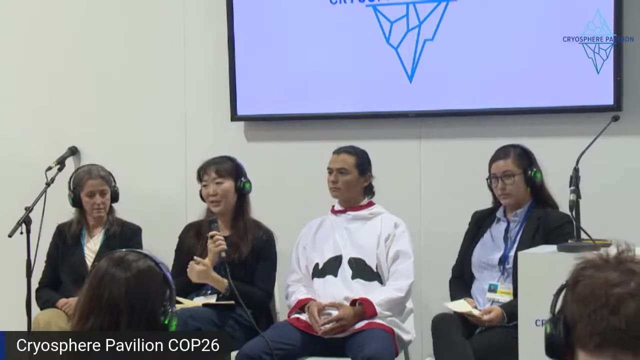 So with the Sami community, they make this probably the only actually like trademarked shoe- footwear that's made out of reindeer and it's the lightest winter boot on the planet. but then now the community is getting affected on, obviously, the of the reindeer and we've basically seen it now firsthand and we're trying to 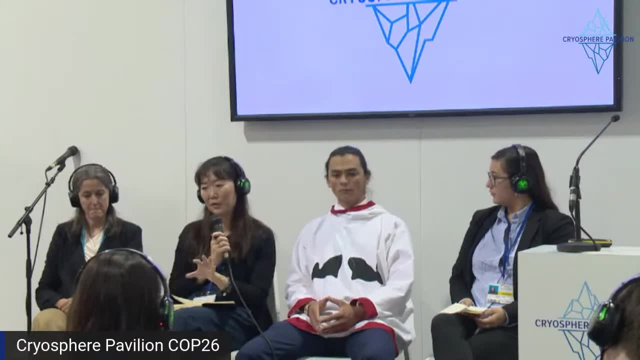 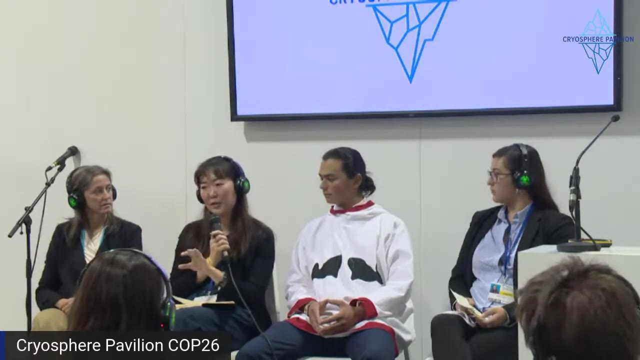 basically collaborate not just with the Sami community but the indigenous communities around the world, like the Navajo, the community in India, in Mongolia, in the Kalahari desert, basically to preserve the cultural coupling techniques, but making sure it's done in a way that it's 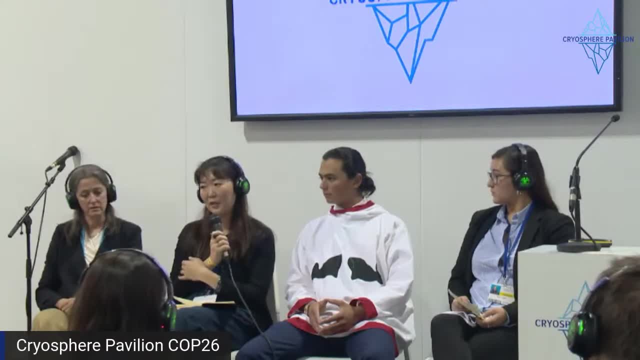 net positive for the localized environment, if that makes sense. So the idea is that to launch regeneration fund. so you all know about like carbon offsetting, but with these community programs we can create fund for regeneration where it's no longer about like offsetting or being like. 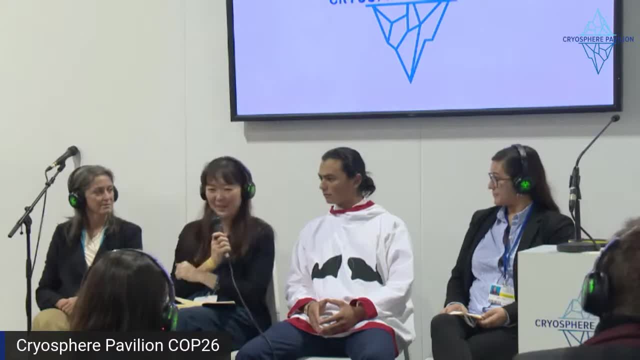 net neutral or net zero, then we need- it's like we're way past beyond that. So yeah, so that's. I hope I didn't wobble too much, but that's basically the idea- and come and visit us and we can tell more. that's at the UNFCCC pavilion stand. Thank you. 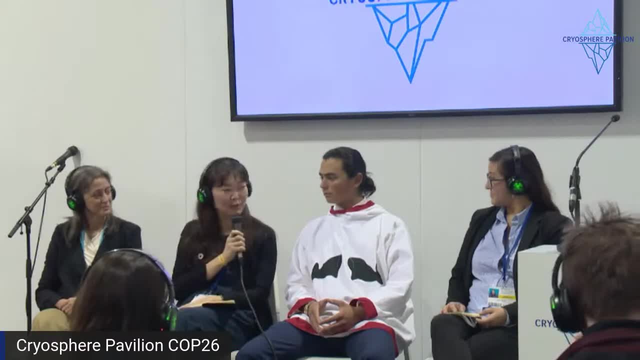 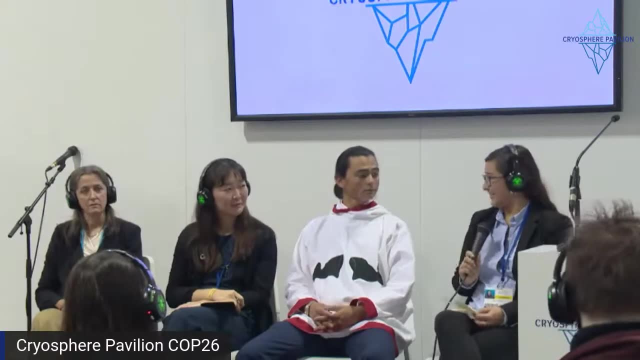 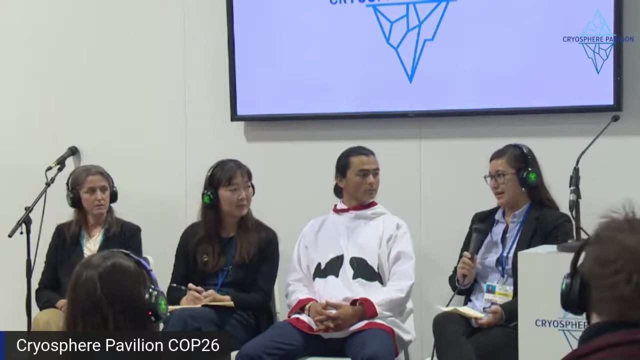 Stand called vivo benefit. So, yeah, that's that's where we're at now. Thank you, No, thank you. yeah, that's super important work and I'm, yeah, thanks for being here and for sharing your experience in your work. it's really meaningful. Yeah, so me I kind of. I come from an interior Alaska perspective, so non-coastal. 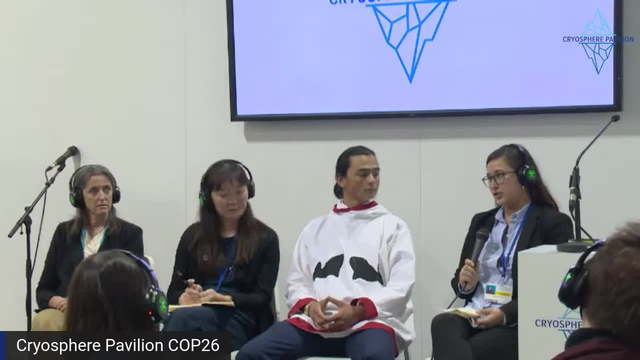 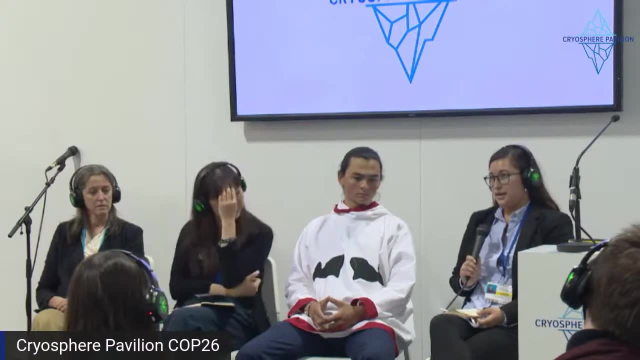 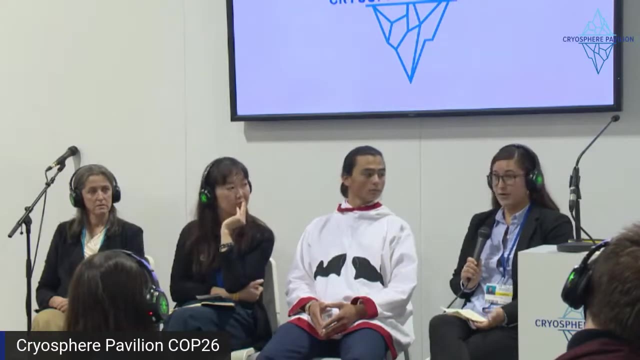 and the changes that we're seeing in terms of climate change are directly tied to our culture, and you can't really have that conversation without talking about policy either. in the US so permafrost is thawing, obviously in Alaska, and that's causing our riverbanks to erode the Yukon. 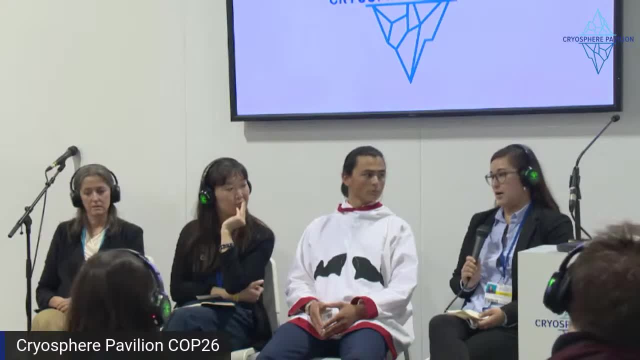 river is a lifeline for many indigenous communities, if not all, along the Yukon river, and it provides food, water, shelter, everything that our people completely rely on as a means of subsistence, so survival. and if the permafrost is thawing, that's changing the way that we're seeing the climate. Is that correct? Yeah, I think that's a great question, So I think I'll take that. I think that's a great question. I think that's a great question. Yeah, I think that's a great question. I think that's a great question. 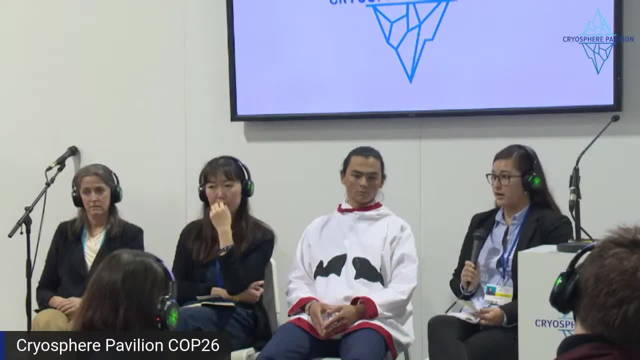 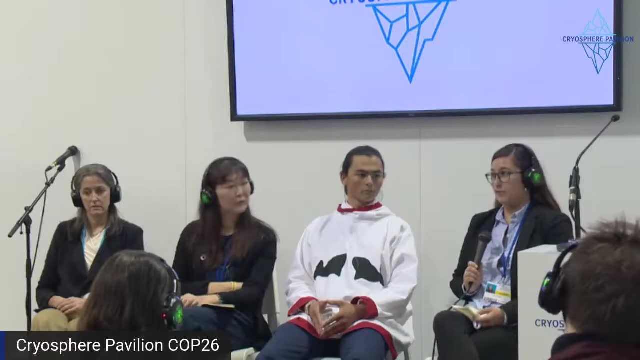 So I think that's a great question. So I think that's a great question. So I think that's a great question. the chemistry of the water: it's changing the spawning grounds for salmon. For me, much like Sam here, climate change is creating incredible food. 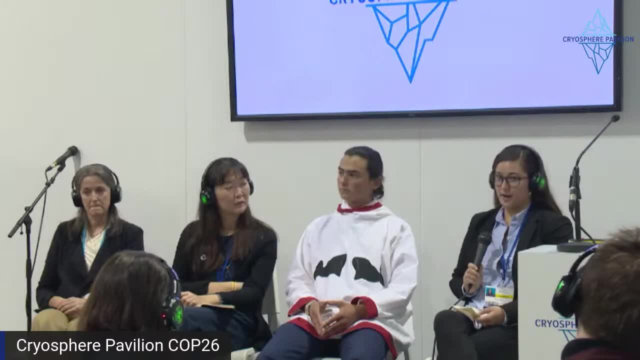 insecurity in terms of what we're able to harvest and hunt and collect and put into our freezers and live off of. There's no grocery store in Beaver. The nearest one is 110 miles away. Freight is very expensive so we rely completely on 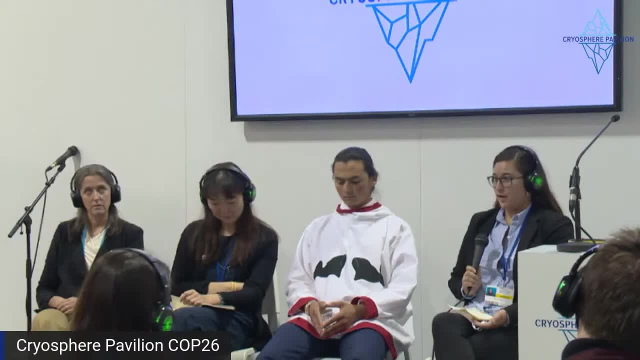 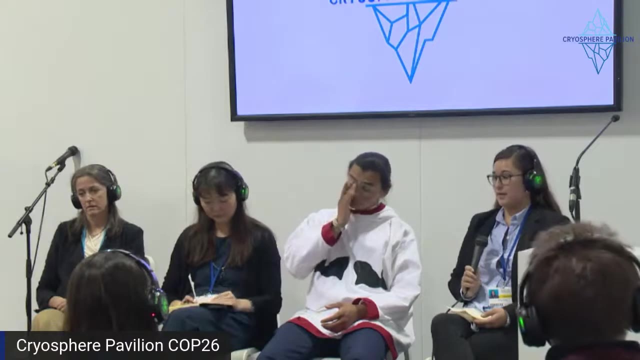 the environment for survival and with the thawing permafrost and the eroding Yukon River, it's changing the salmon spawning grounds, like I said, and that is one of the many contributing factors to the mass decline in king salmon in Alaska. This past year was the first year since I believe ever, that my 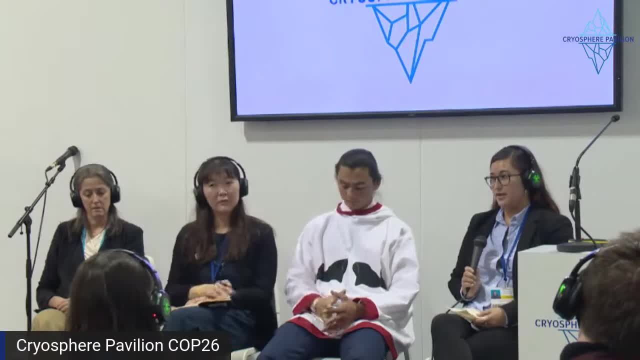 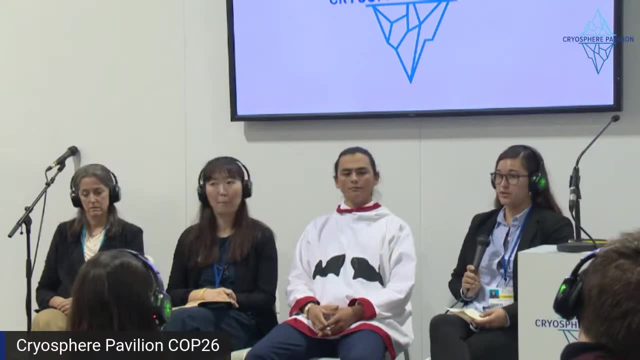 community wasn't able to fish. We were completely shut down by the Alaska Board of Fish because there aren't enough salmon for us to fish. Meanwhile, commercial fishermen in the ocean are by catching hundreds of thousands of king salmon. In terms of policy, it's very unjust. It's not fair at all. Indigenous people. 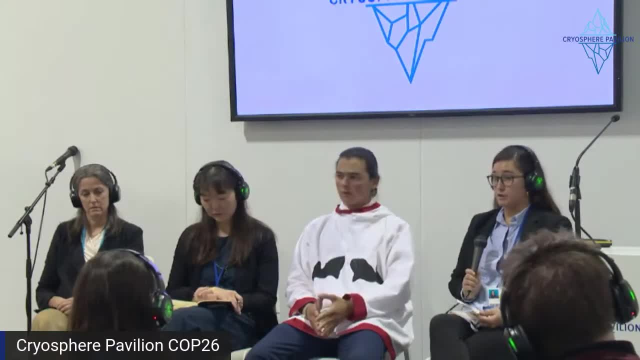 are contributing the least amount to climate change and we're feeling the impacts and the regulations the most. It's a huge conversation and, since we aren't able to fish, a lot of the pressure for food shifts to then moose and to harvest moose. I mean there are regulations in Interior Alaska that also. are unjust. out of the one month that we're allotted to hunt and harvest a moose, two weeks of those. are the moose actually viable and is it easy to hunt and harvest a moose? so that's two weeks out of an entire year to get one moose. each person's allowed one bull moose. 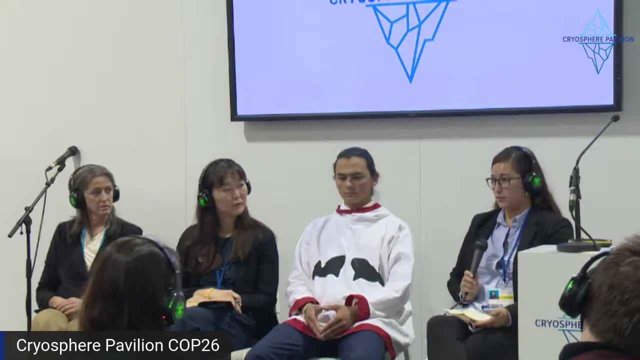 I was fortunate to get a two-year-old this year, but I was with a different family of six people. there are eight people in my family, so that's a lot of people for a two-year-old moose. it's very small. yeah, it's going to be pretty scarce this this winter, but we have meat and that's I mean. 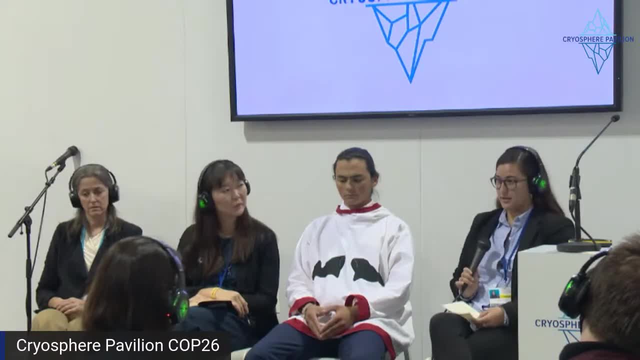 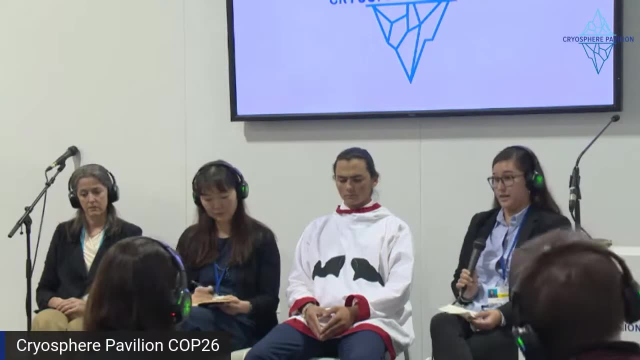 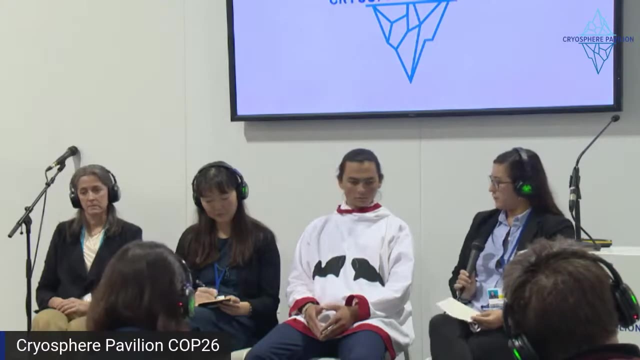 that goes straight into our freezer. none of it's for sport, so that's in. in my perspective, a lot of it is food insecurity and clean drinking water problems. that are the impacts that I'm seeing in beaver, Alaska, where I'm from. so we're obviously really tied and work really closely. 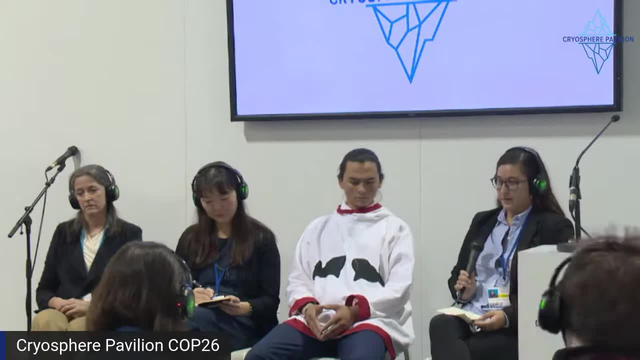 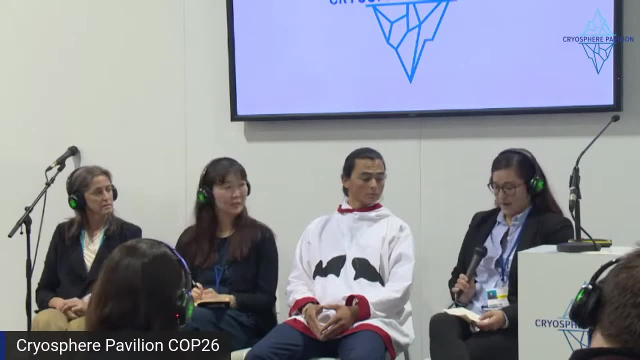 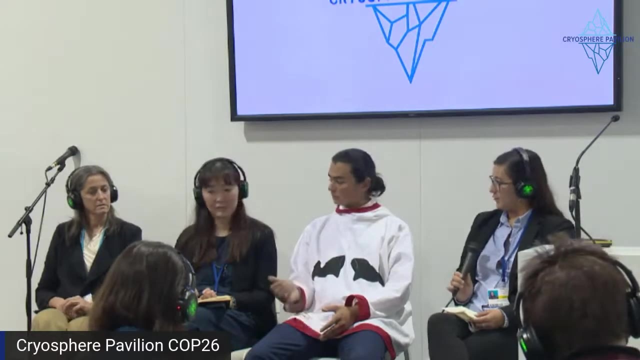 with cultures that rely on the environment, and this is a pretty science-heavy pavilion, and I think that I want to ask each of you, all of us, how do you think scientists and policymakers can better engage with, interact with and learn from arctic indigenous residents, and how would that benefit to the value of the research and or policy? 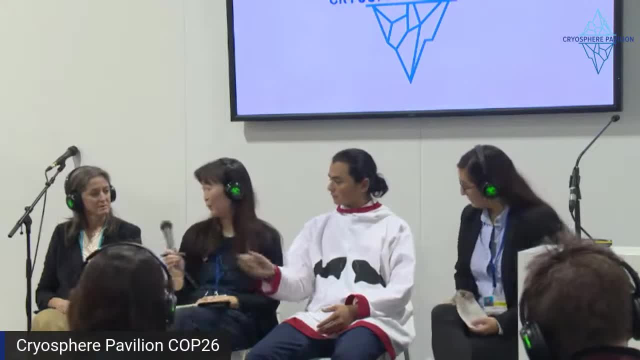 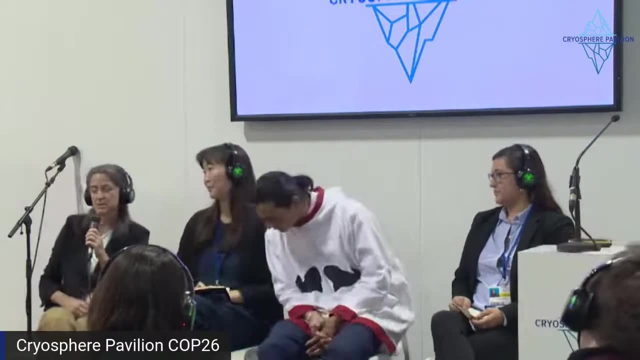 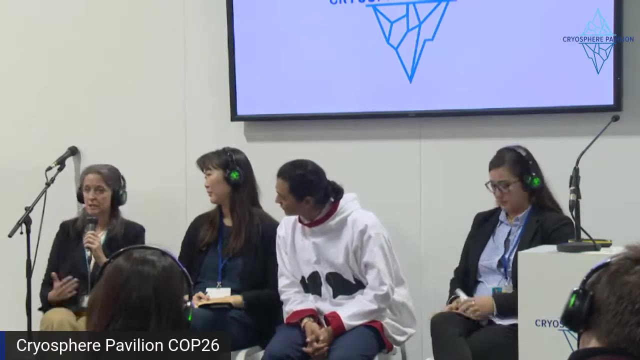 I think this is coming to me. so I'm a scientist, I'm Sue Natale, and I work with D'Arcy at the Woodwell Climate Research Center, and I'm not from the arctic. I live in Cape Cod, Massachusetts, the land of the Wampanoag people, and I shop at a supermarket. so I there's a lot. 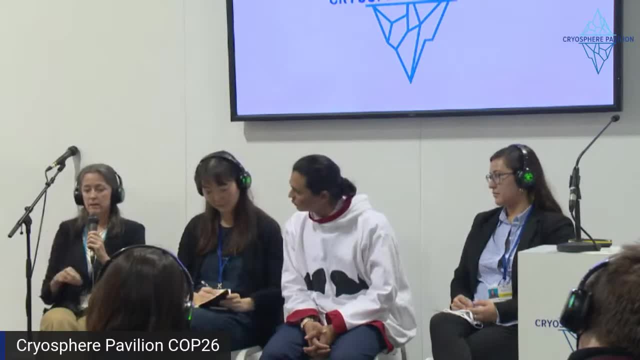 that I do do and I do a lot of research and I do a lot of research and I do a lot of research that I do not know. and, as a western scientist, the way that we get trained is to be very, very focused and to you know, be an expert in a certain area. but we know, and then we try to do interdisciplinary. 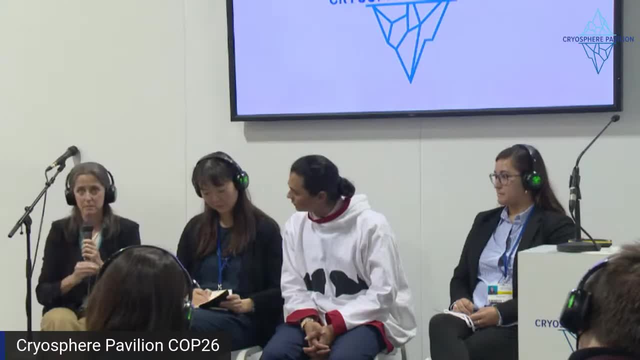 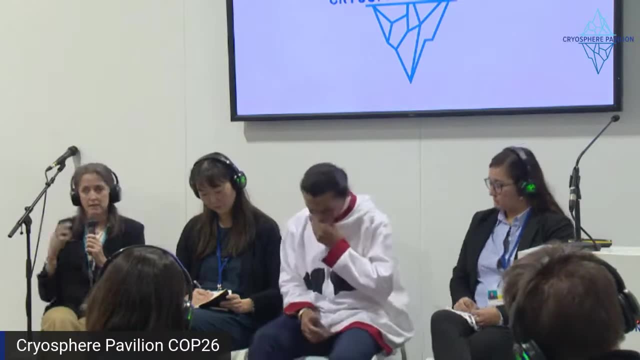 work and sort of connect with other scientists who are really, really focused. but if you've listened to this panel in the previous panel- people who are relying on the environment and living in the environment. they don't need to sort of take the world apart and put it back together because the 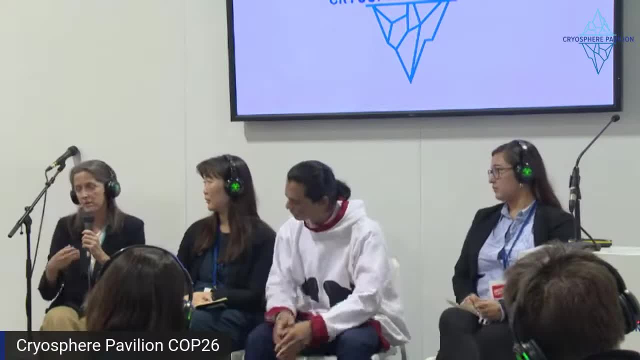 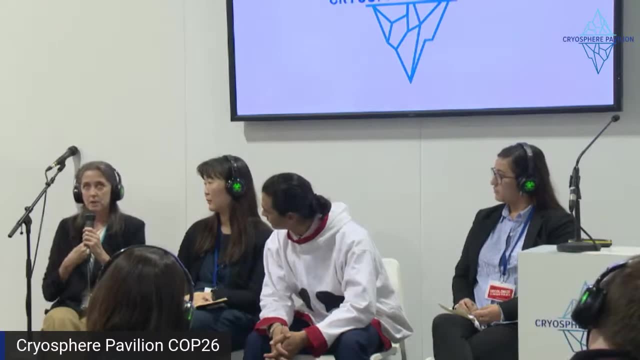 world's together, right. I mean, you're talking about food security, you're talking about health, you're talking about you know how you, how you move around the landscape, you know what the habitats are for animals, and so I guess the best way- I think the question was how- the best way to 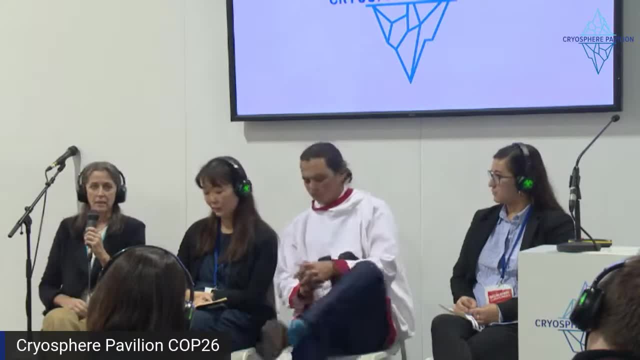 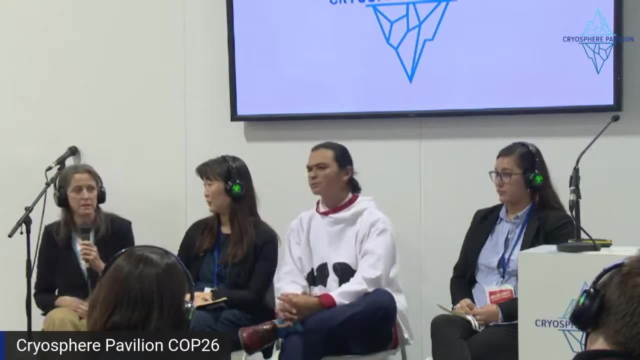 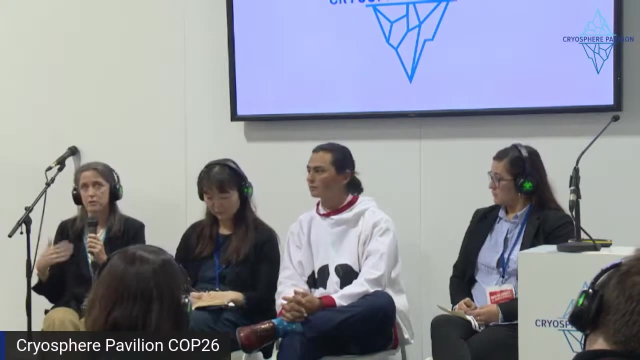 learn. I think the best way to learn is to listen and yeah, like I have to tell that message to myself a lot like just shut up and listen, because I learn a lot when I shut up and listen and some, and also making the time to do that, I think that we often are very have this urgency of having 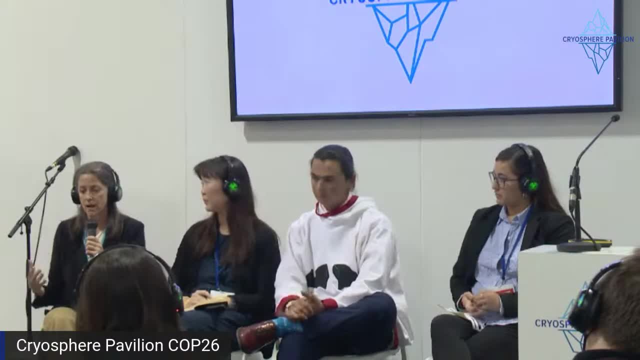 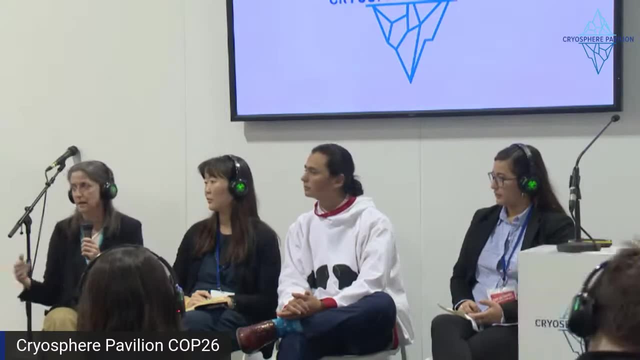 to get things done and having to get things done and having to get things done and having to get things published, and so building in that time. if that's important- which it is important because, honestly, in the long run, we will get much farther, much more efficiently if we take the time to sit. 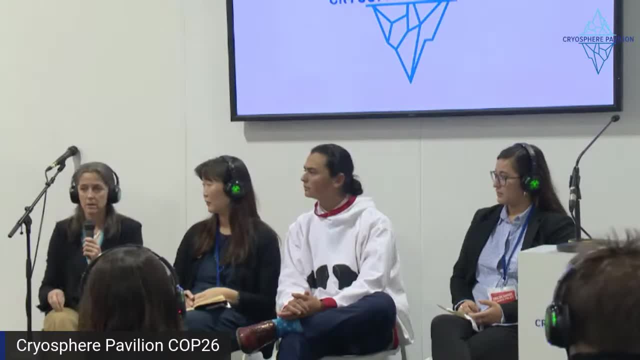 and listen from these experts in the way that we do the science and I and I just have to say the same thing goes for policymakers, I mean. I think again it's. it should be a conversation and not just me doing my science and putting it out there and saying here it is on a platter and it's not. 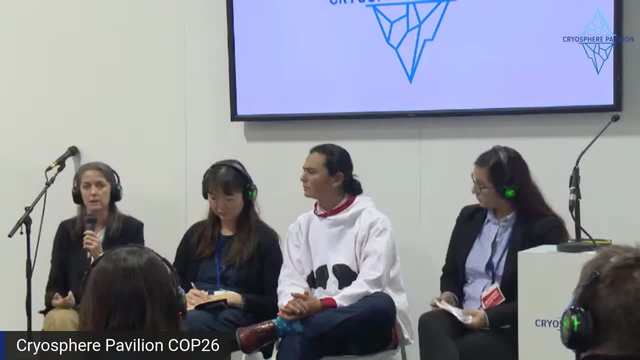 really useful for anyone. so I think the same thing goes for policymakers sitting and having to having the conversation and spending that time and having the conversation and thinking about and listening and asking what is, what is the science and how is it that you want it to be done? like 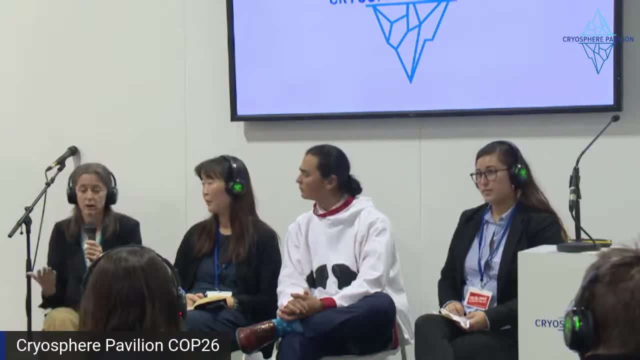 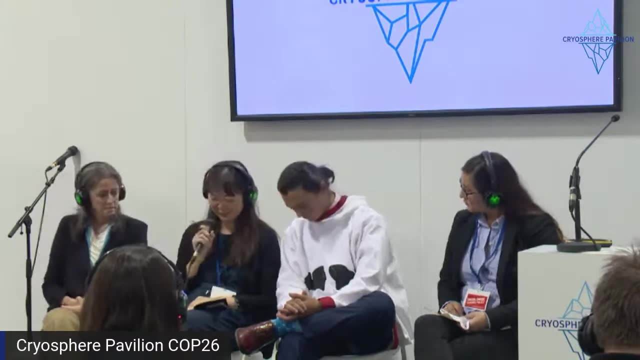 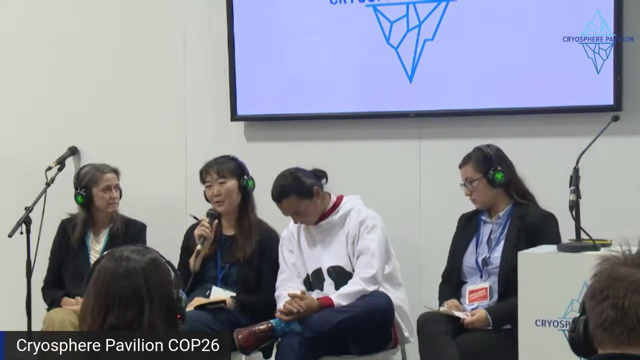 what is useful, you know if that's a priority, if it's not a, you know. yeah, so I'll stop there. so I've done quite a lot of activism when I was growing up, where, at the age of 16, with a crew of my university classmates, we started an NGO to clean up the shores of 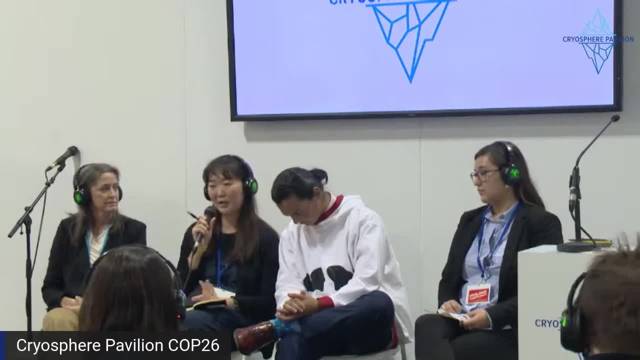 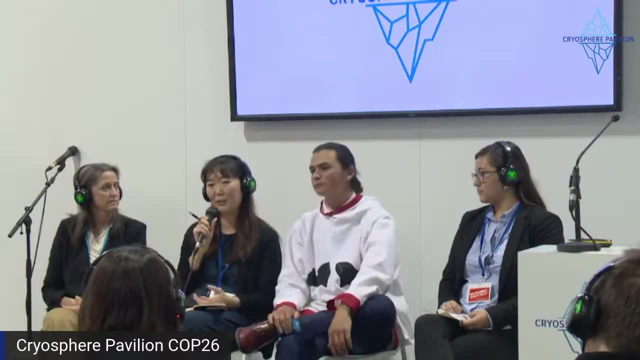 Lake Baikal from rubbish because there is no like social infrastructure. like you know, government didn't put basically enough bins and there is no like system behind to keep the territory clean. however, Lake Baikal is the deepest lake in the world, contains 20 plus percent of the fresh world. 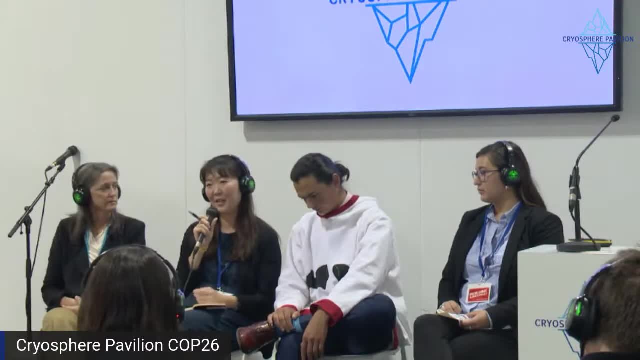 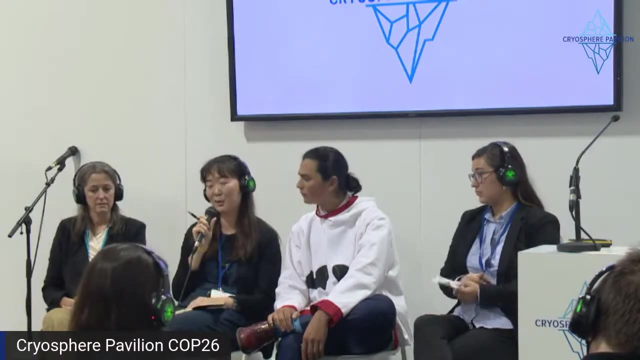 water is UNESCO heritage site and then this is how it's treated. it's like, I mean, like I mean, everybody knows that Russian government is all over the place and it was like, yeah, a bit helpless, so with the students we did that and then when I moved to Europe, I started raising funds and sending to Russia to support. 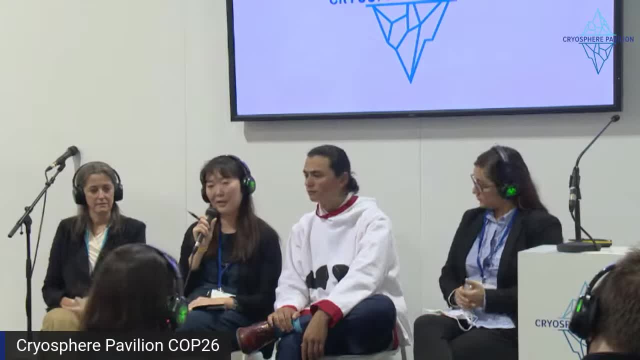 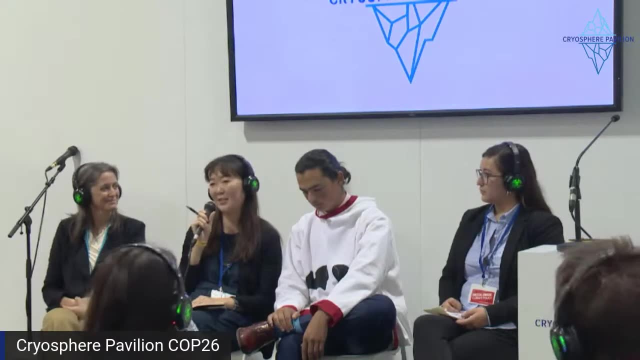 the program because it's still going on. and then they did this law about international agents- if you receive funding from overseas or like outside of Russia- that basically our accounts got blocked and we didn't have access to any of the finances that were raised here for like two years. so we had 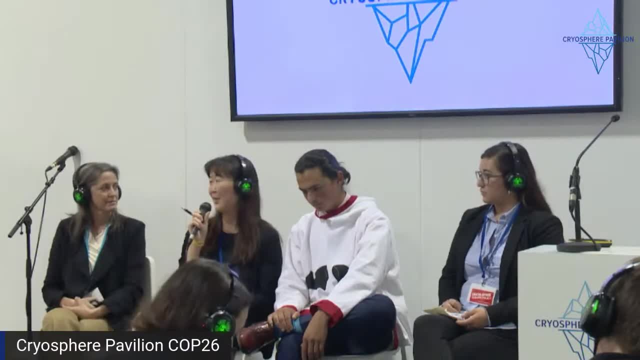 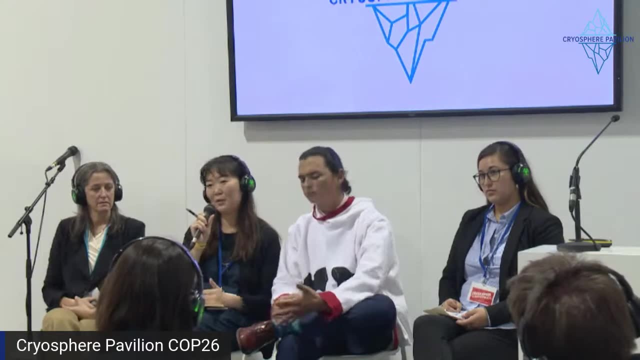 to do like tons of paperwork. so there's kind of like practical examples how you know, terrible the system is in the first place. the second thing is like how do you amplify voices through whatever work you do like? we're an example of a, like you know, baseline sort of. 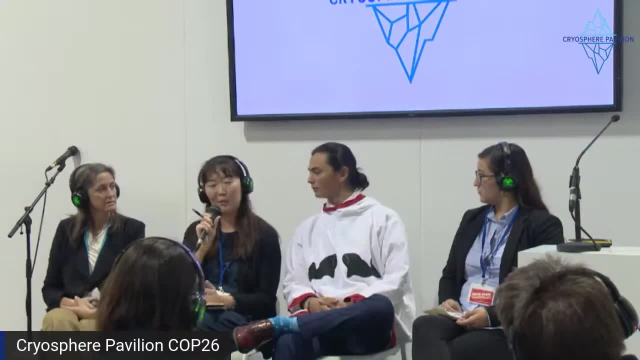 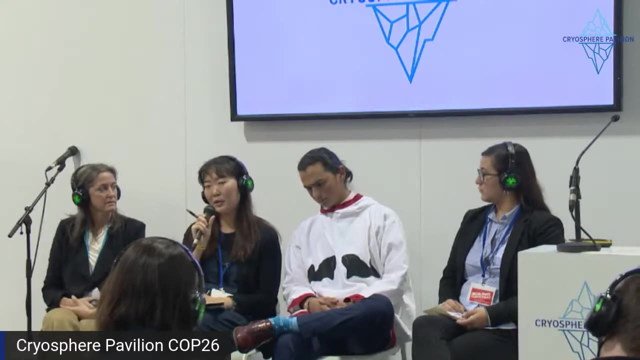 footwear business, but you can still utilize your product as a medium for storytelling. so, as an example, this year this spring we collaborated with a US-based NGO called Oxygen. it's like almost like an advocacy media NGO, and we did an open letter to UNESCO on stopping harmful 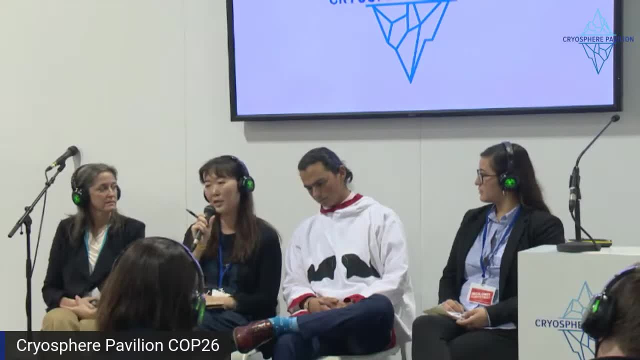 algae blooms and there was also related back to Lake Baikal, because it's all getting algae blooms and they can be also toxic, depending like what. what caused the blooms? because, like the industrial agriculture, the water runoffs and then it, basically this balances the system and then the 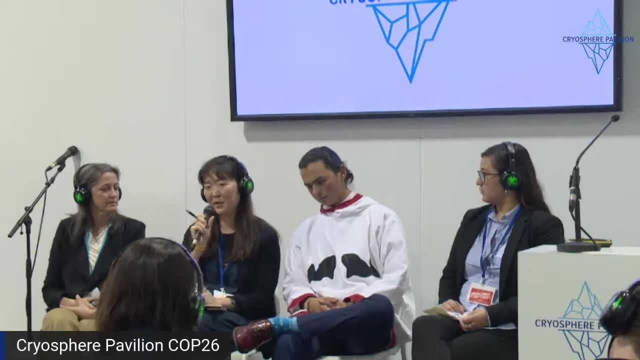 water that was pristine. they clean. you know, even like six, seven years ago now, where you get like all this green. I don't even know how to describe it. sorry, English is not my first language, but you know we used to just drink the water from the lake. basically, let's put it that way, and now we don't do. 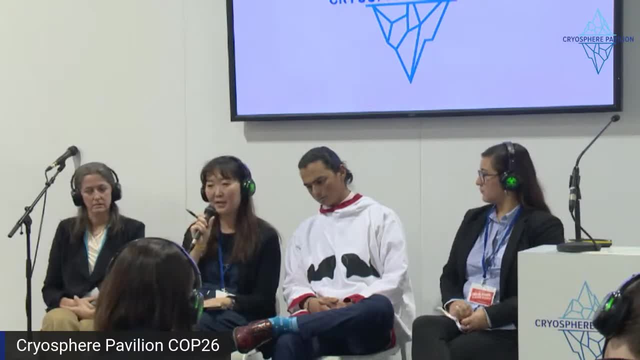 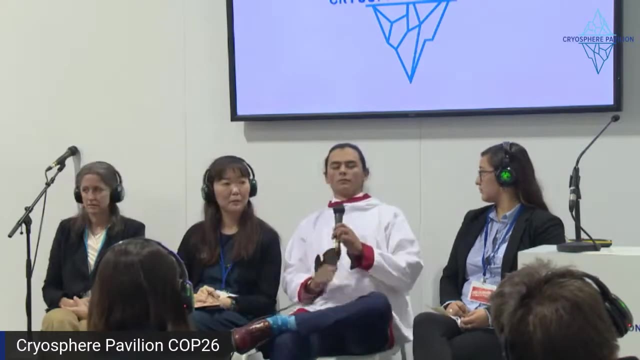 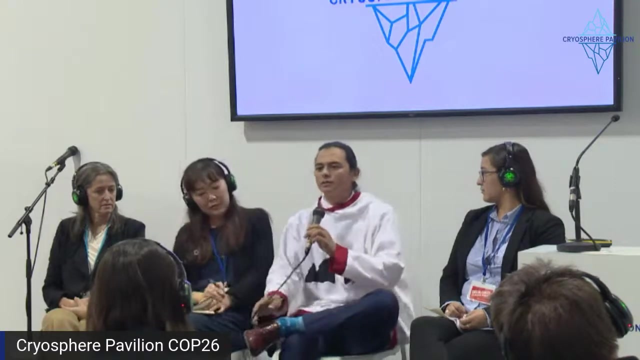 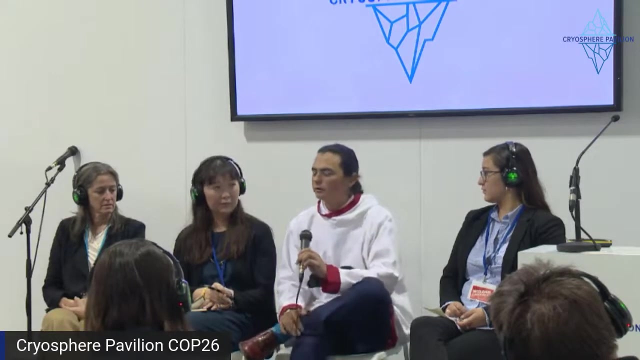 it because it's like we never know what's inside now. so yeah, so I guess there's two things: co-create and then somehow make sure the government listens. but it's a tough, especially in my home country. um, I I guess my thoughts on this are are rooted in in one of the formative experiences that I've had. 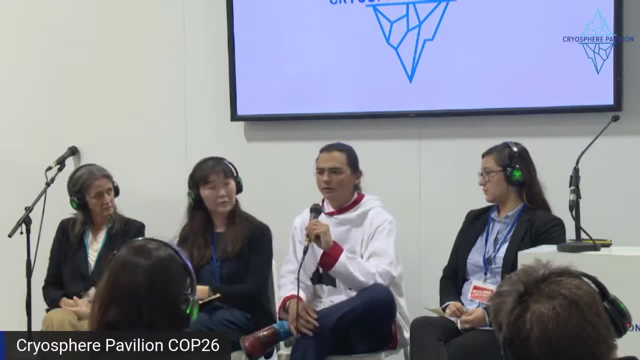 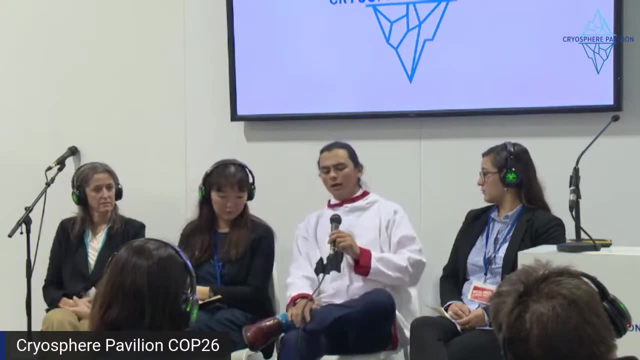 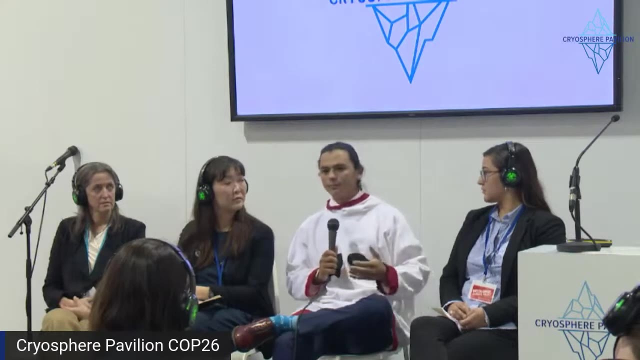 um, at the age of 16, I had the honor of sitting on our governor's climate action leadership team, which was led by the first Alaska native Lieutenant Governor of our state, and in those meetings it was uh, a team that was 26 people, one of which was a. 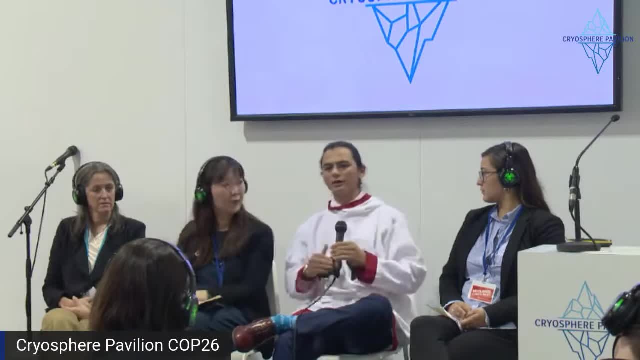 youth, and the rest were scientists, industry leaders, oil and gas executives, forestry people, fisheries people, native communities that were all coming together to try and formulate a comprehensive plan with regards to climate change for Alaska, And I remember very specifically a meeting between myself, our lieutenant governor and the chairman of research for the University. 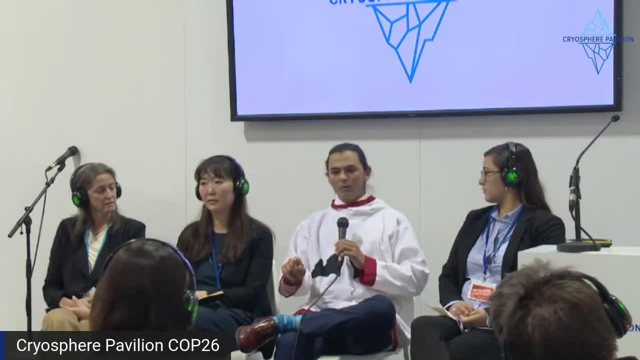 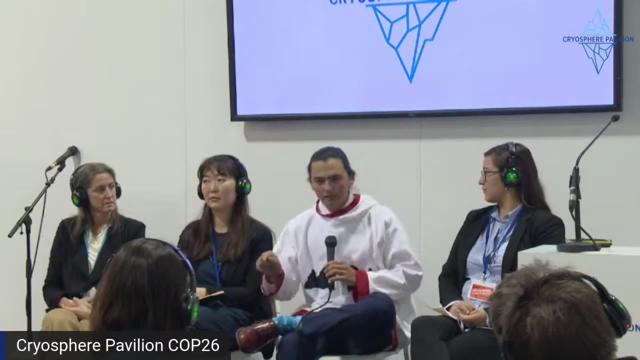 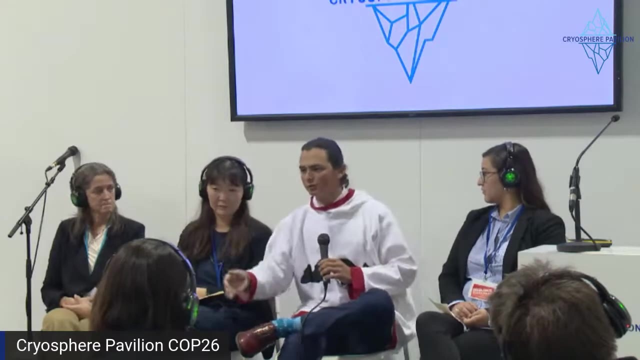 of Alaska And in that meeting, the chair of research for the university was saying that we need to study the things that our native partners in this room are saying, because we can't prove them right now. There isn't scientific proof of what our communities. 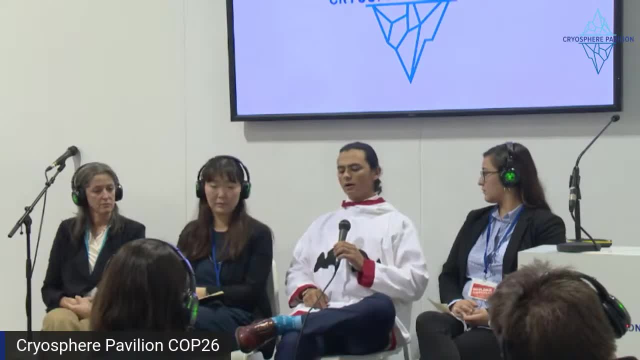 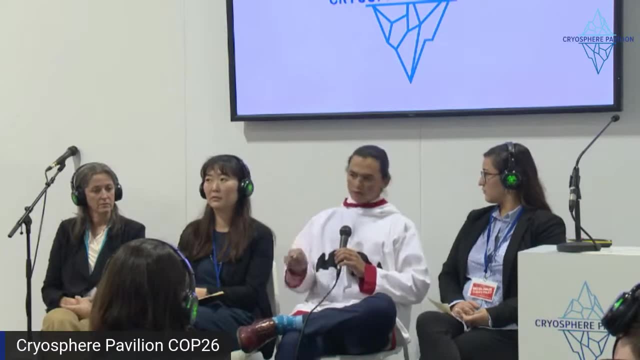 are seeing what they're saying, And so what our lieutenant governor said is: our communities have been living in these places For thousands and thousands of years. Their observations in a single day measure far past what Western science can see in an entire year, because it's built on our traditions. 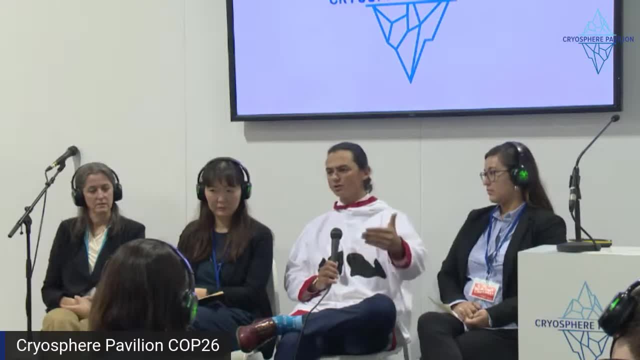 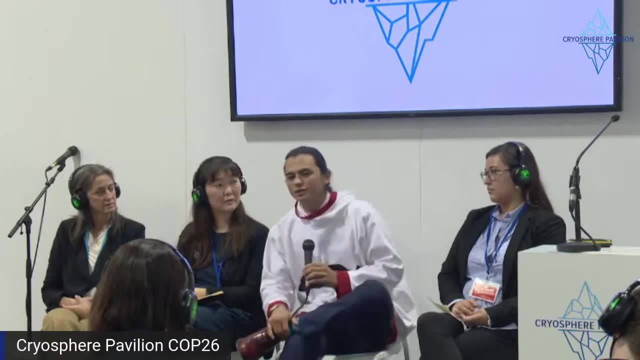 it's built on our historic knowledge and it's built on the stories that we pass from generation to generation. Long before we were seeing currents changing, or Western science was seeing currents changing in the Bering Straits, my uncles were talking about how it was different- Our tides- 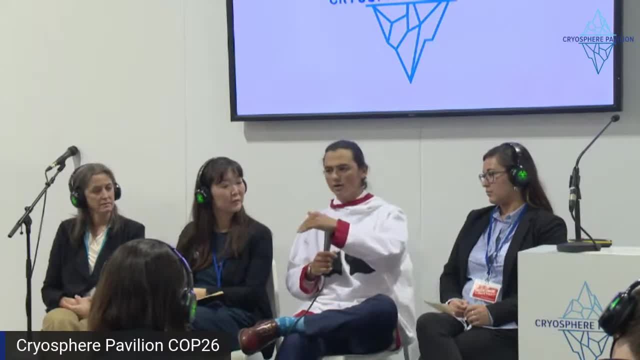 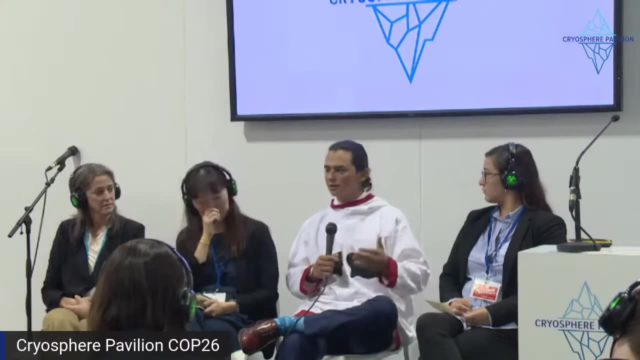 were changing. The waves were changing, The waves that are changing, The waves that are changing. Our water came in, The nutrients that was coming up in the way that our whales were feeding. We were seeing those change in the 1990s. You didn't hear Western science start talking about. 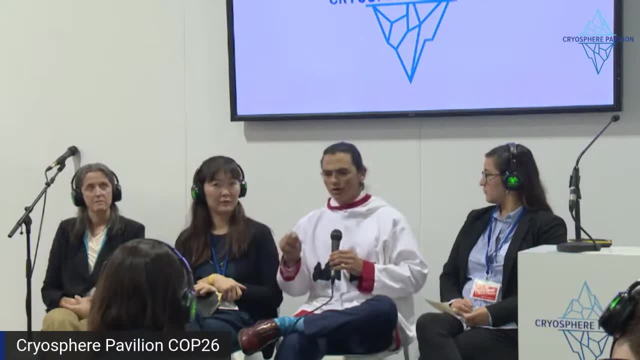 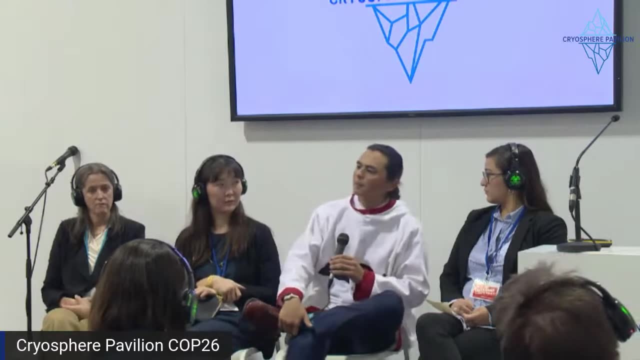 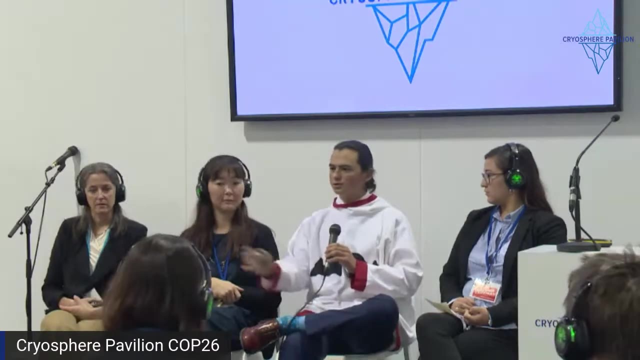 this until the mid-2000s. Our communities are, in a sense, from an observation standpoint, a canary in a coal mine. We're the first ones to see it because we're the ones that feel it, And so, while we can embark on large research projects that take 10, 15 years, 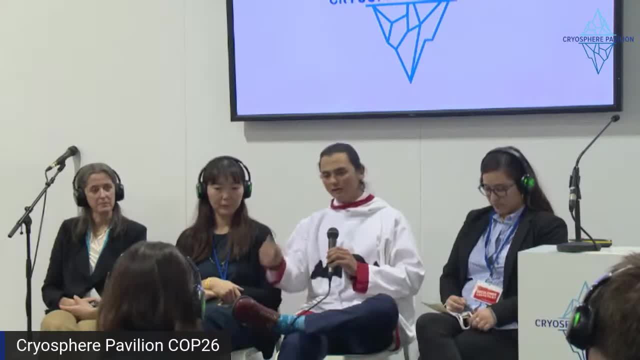 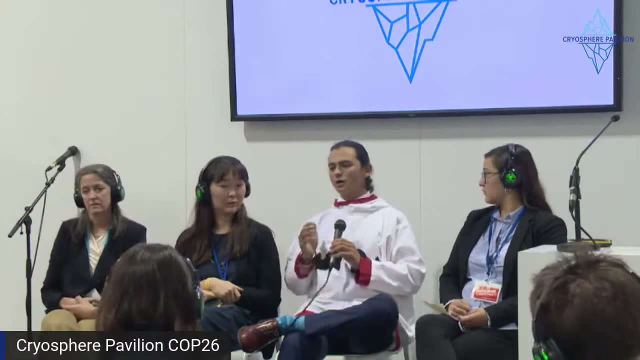 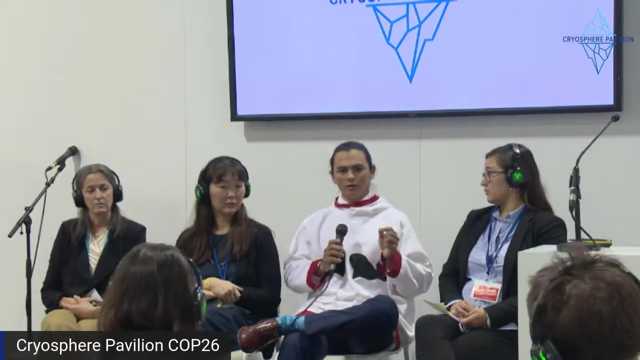 to come up with conclusive results. our indigenous communities living in these places see these changes day to day, And so I think good policy and good research are done in such a way where there's collaboration and not consultation. I think a lot of times you hear consultation. 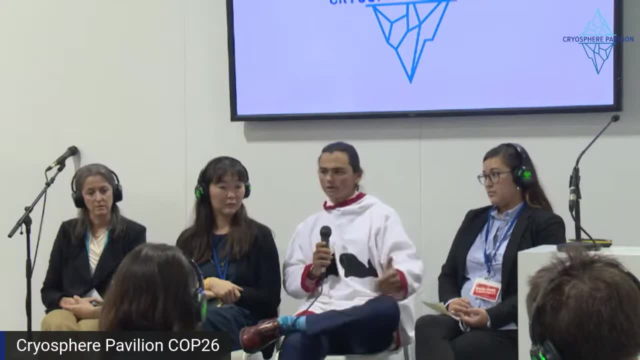 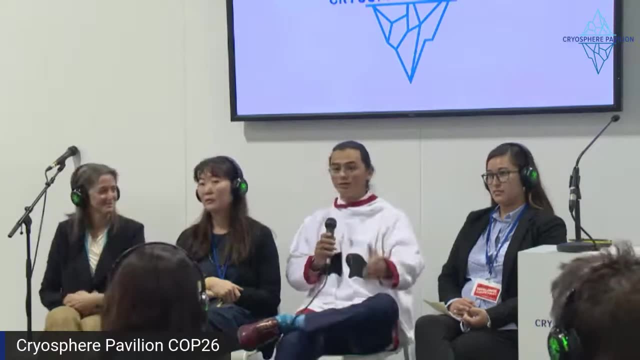 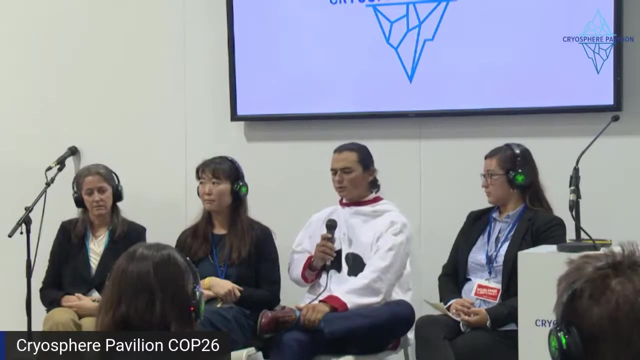 consultation, consultation. And, at the end of the day, what consultation means is that? well, actually, how many of you guys are researchers here? That would actually probably be more. Oh, actually a lot of you. And are the others affiliated with NGOs or stuff like that? Yes, So in consultation, I think what? 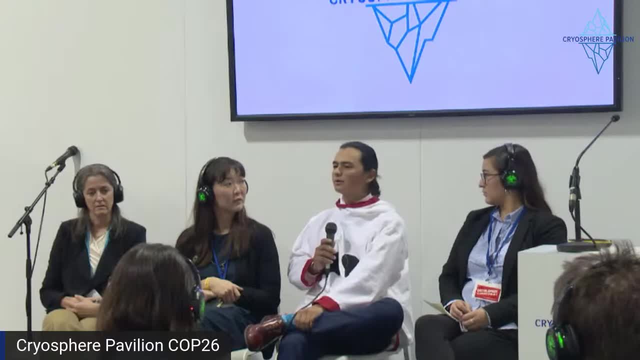 happens, or what it really means, is that you can sit down with the indigenous community. We talk about what we want to talk about. You tell us what you want to tell us, And then you don't have to, you're not obligated- to include anything that you've heard. You just have to listen to us. 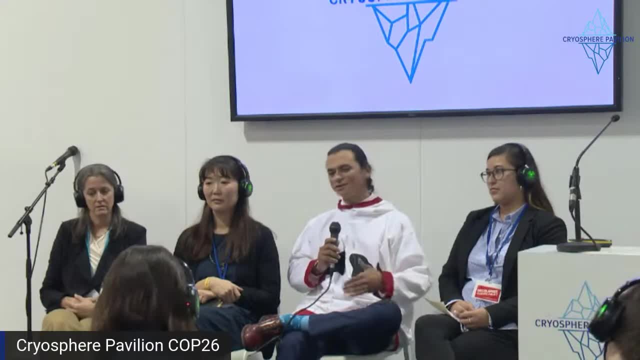 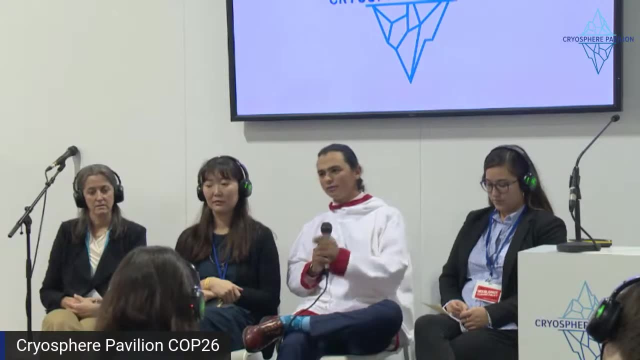 say it. This is our relationship with the federal government in the United States. We say things, they disregard it, They do what they want, Whereas collaboration means that you're working together with a community. It means that you're going to a community and saying: all right, what do we want? 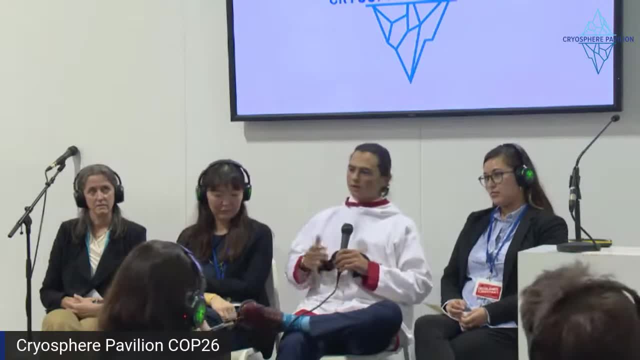 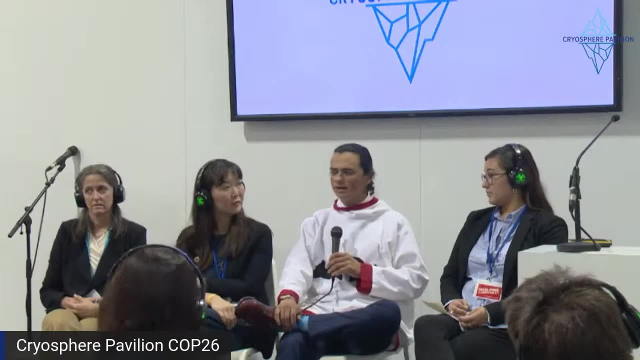 to study Because we have people come to our island, oftentimes spend hundreds of thousands of dollars on studies that have very little applicability to the actual needs of a community, And so the scientists are alienated. The researchers are alienated from being able to gather. 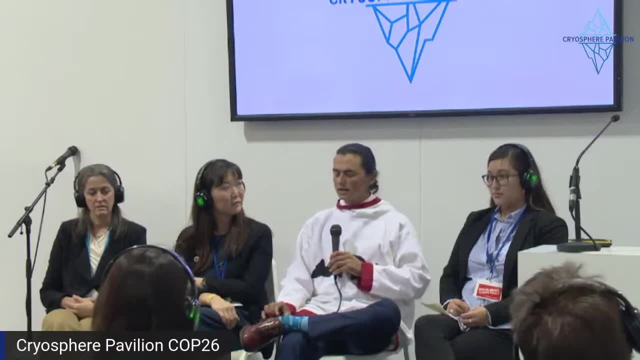 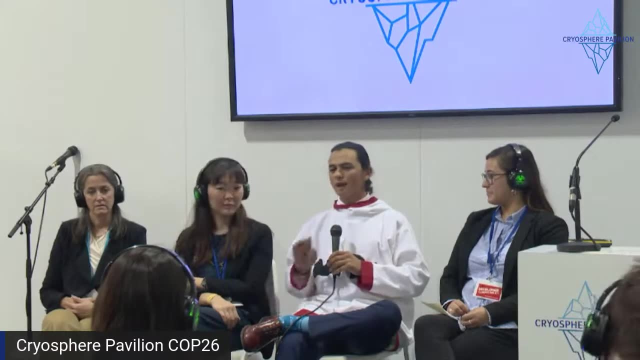 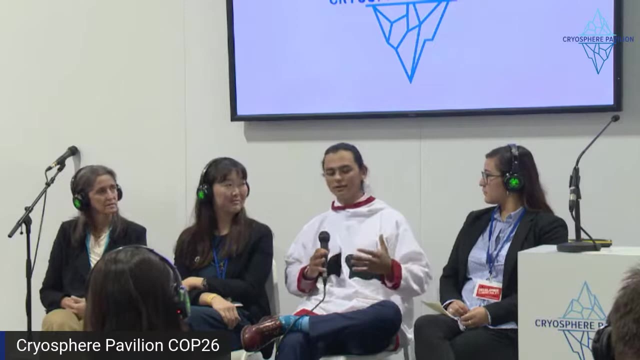 any information from our people because we don't see its relevancy. And so in research there needs to be clear and understandable communication about what is actually being researched, how that relates to a community, And I know that you have to submit abstracts to get funding and submit things. 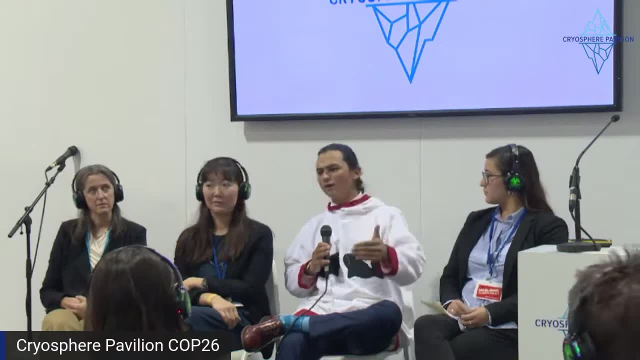 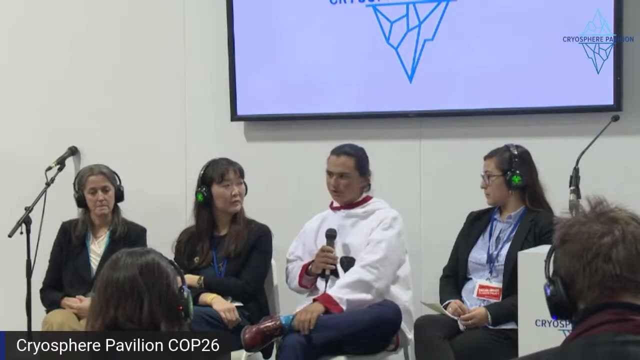 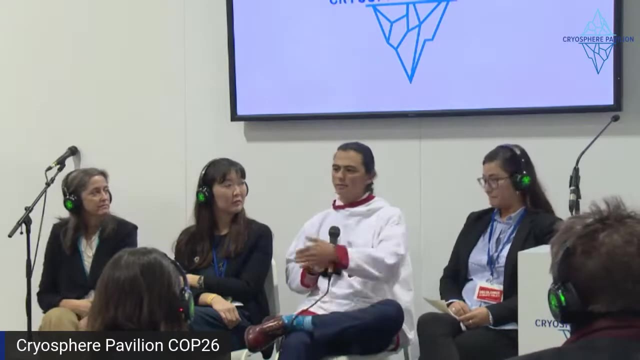 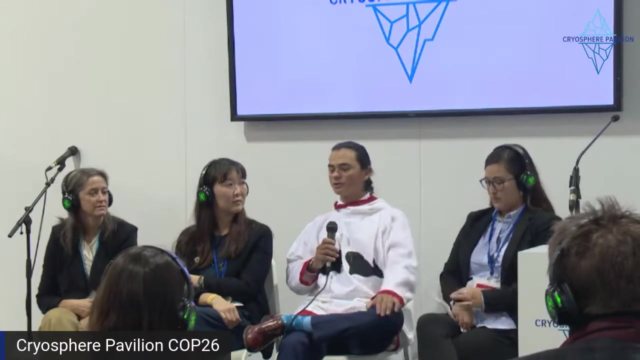 like this, But trying to co-develop research goals is really critical. I remember at our island there was a group that was trying to study sea ice And they spent two years observing our ocean ice And they came to our school to present their findings And we had our Yupik language teacher. 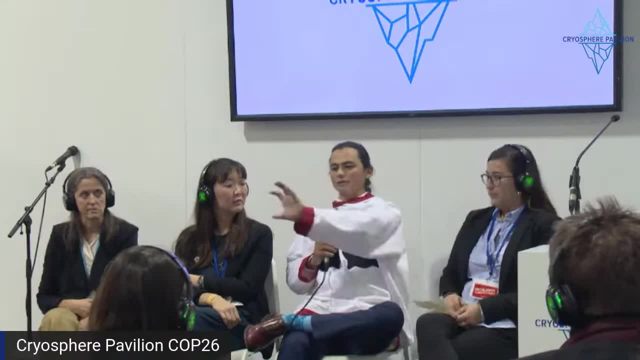 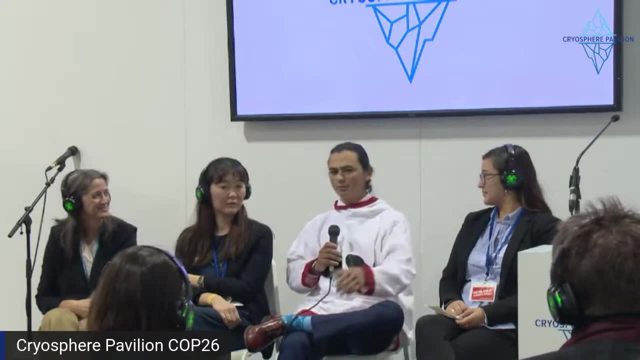 one of our elders in the school and he saw their title slide and he saw the first two slides and he stood up and he told them their conclusion before they even got through all of their research, Not because he'd been paying attention to their research, but because he knew our ice And so 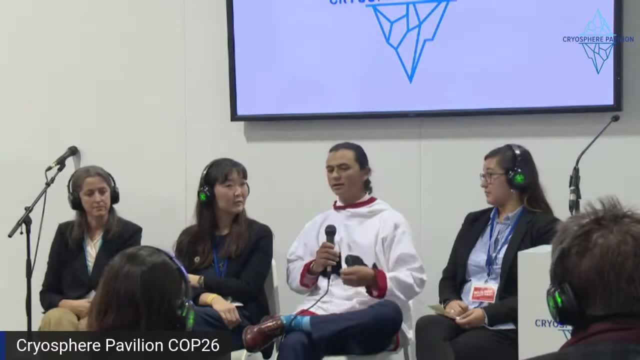 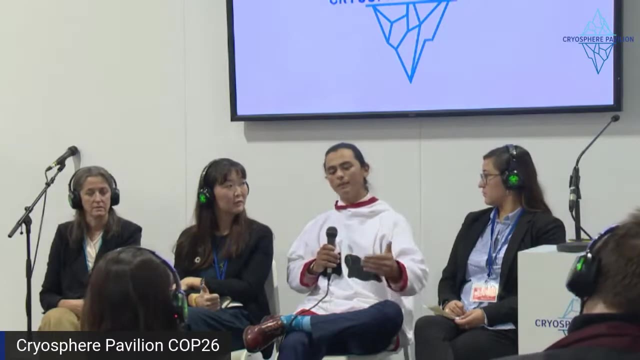 sometimes there's simple answers to the complex questions that are being asked And really a lot of time can be saved and a lot of direction can be saved Just by asking the indigenous community: what are key things that we could look at, What are key things that you're observing and how can we help to prove the things that you're seeing? 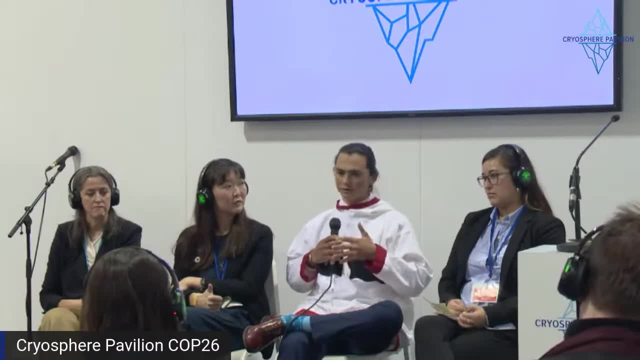 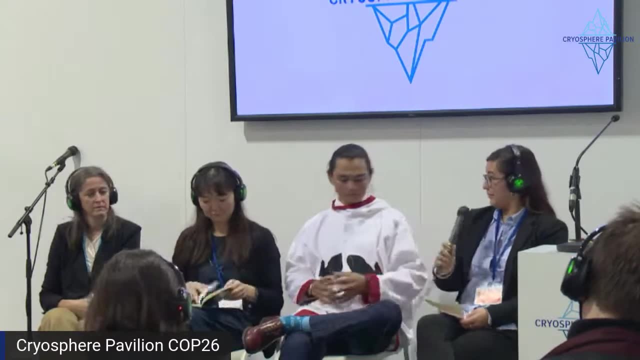 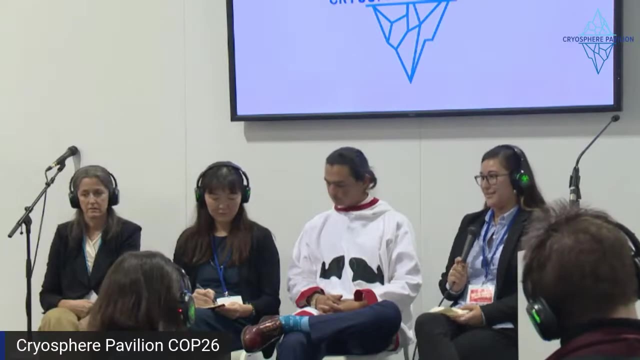 Because when Western science and indigenous knowledge come together, you actually see good policy coming out of that. So those are just my thoughts, though. Yeah, I mean, I don't know how much more I can say than that. Yeah, I think as a scientist and as an 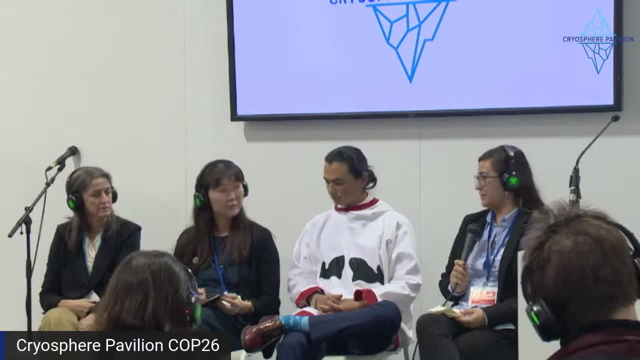 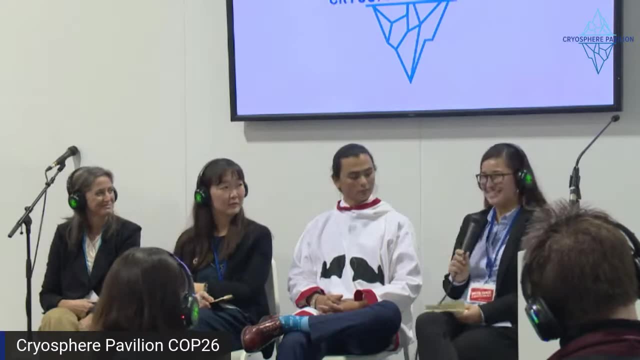 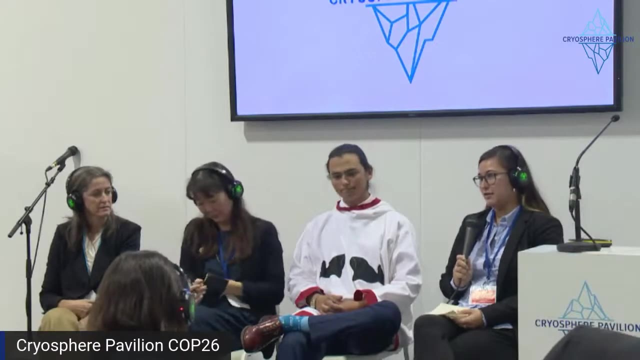 indigenous person, I have a really unique perspective just because I have one foot kind of on each side, maybe like a foot and a half on the indigenous side and half a foot on the science side. Yeah, I think one thing that researchers and policymakers can do better. 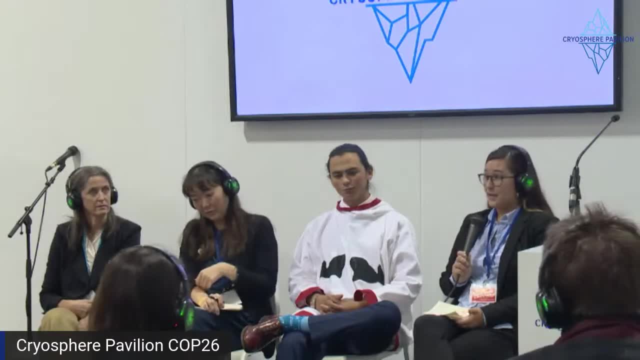 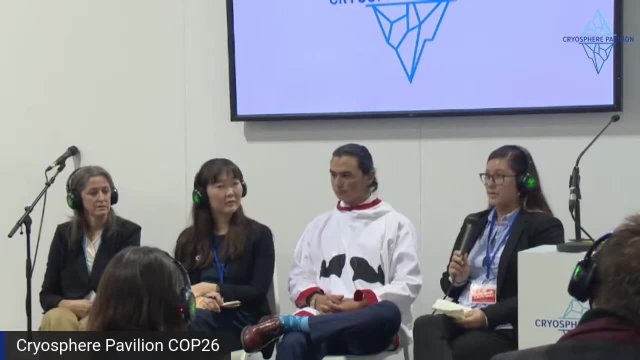 echoes a lot of what Sam's already said, that you can spend time with the community, You can co-develop a project with an indigenous community. that's going to be beneficial for both indigenous people and researchers. I don't see the value in research for the sake of research when it comes to climate change, because 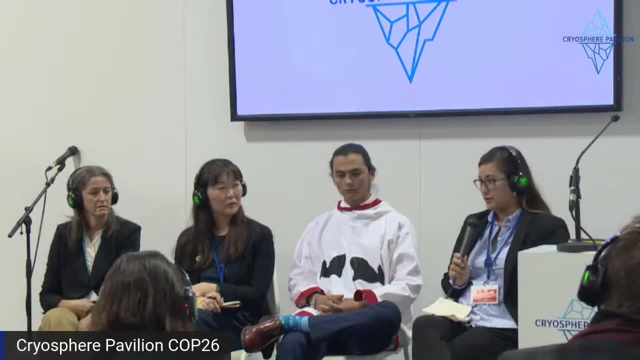 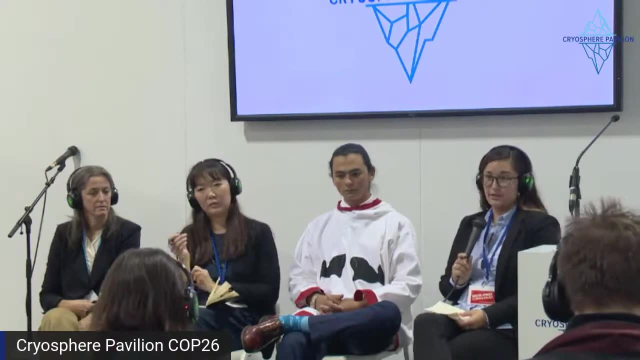 what good is research if it only benefits other researchers And it never works its way down to indigenous people who are living on the land and who are seeing these changes? It's really hard to be based in Texas researching Alaska. when you're based in Texas, You're really disconnected from. 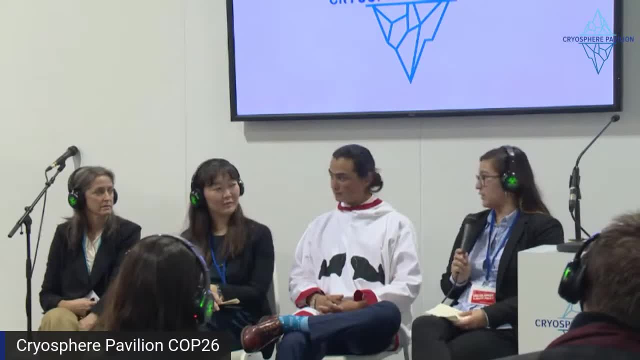 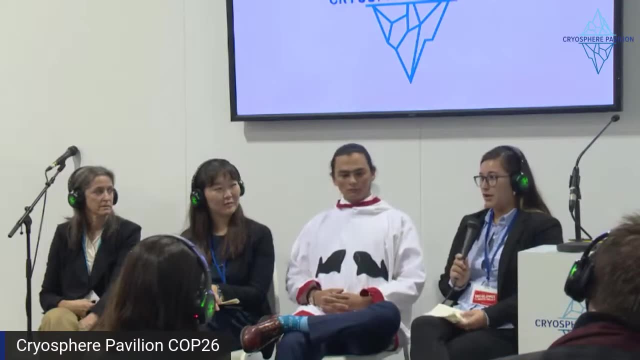 policy. You're really disconnected from the people. You're disconnected from the land. You spend maybe two weeks out of the year there, versus working with people who've lived there since time immemorial and have a plethora of knowledge to offer if you so choose And if you're, if that's a. 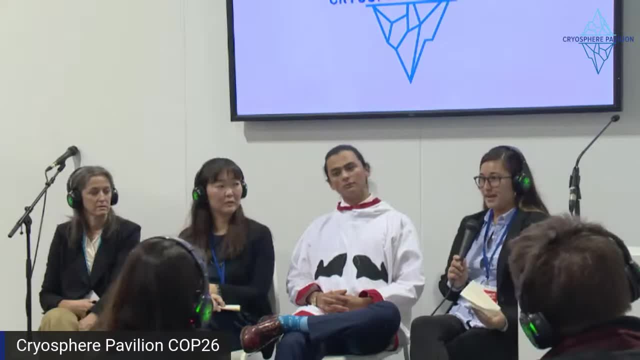 priority of yours, which it should be, because it can only benefit and add to the quality of the research itself. I don't think anybody would be opposed to having like thousands of years of research added. It can only add so much value to it, And that's something I think is really. 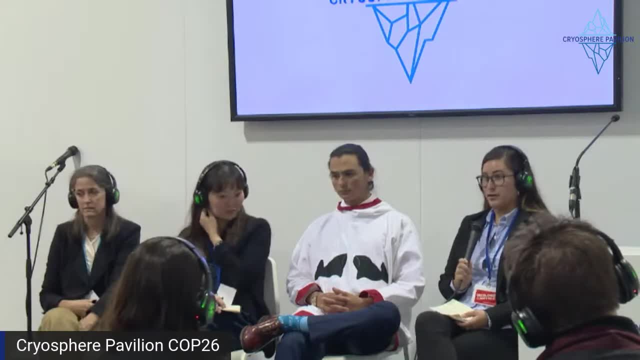 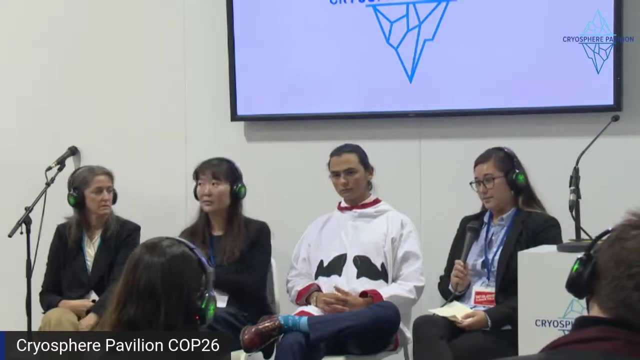 important. I think another thing researchers can do a lot better is to be able to do a lot better with a lot better besides co-producing projects- is they can communicate their science better. It's so easy and there are requirements. I know that people have to fill. they have to publish. 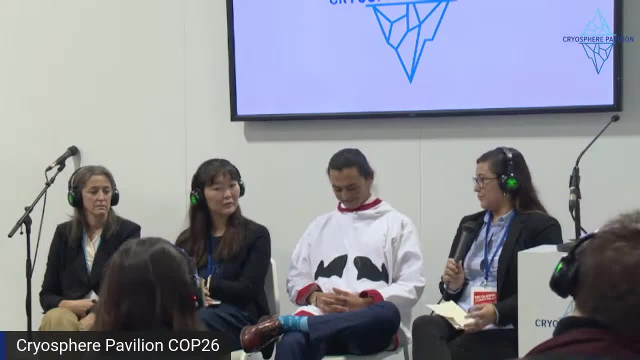 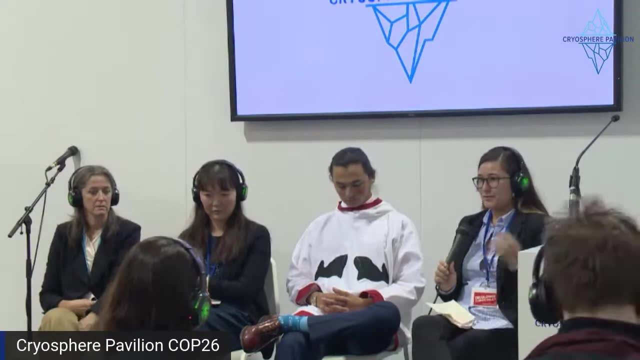 or perish. And then they consult an indigenous community. They don't, you know, work with one. They consult with one, They slap the tribe's name on the paper at the end and they send it off to the tribe in a language that's completely foreign to them. 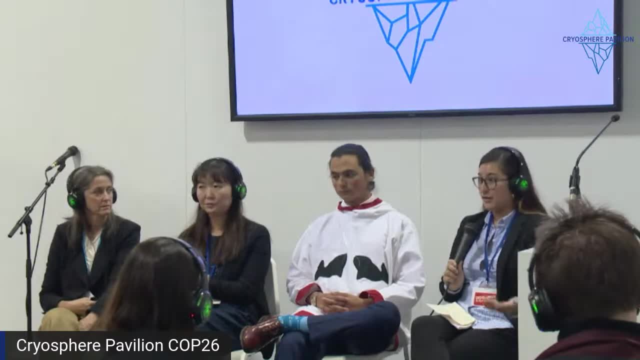 Um, there's graphs, there's tables that they don't understand. No one's communicated with them what this means for them on the ground And they've just, uh, exhausted a bunch of resources indigenous people have by sharing this very sacred knowledge. um, that's been passed down. 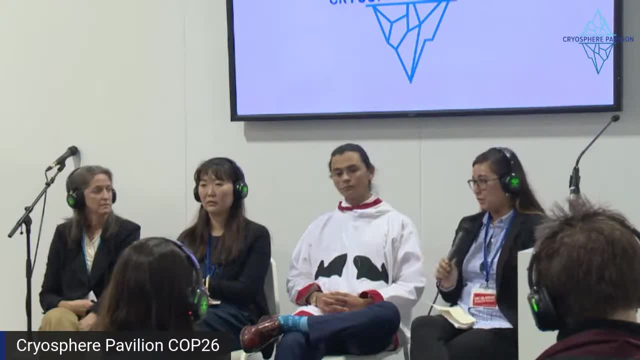 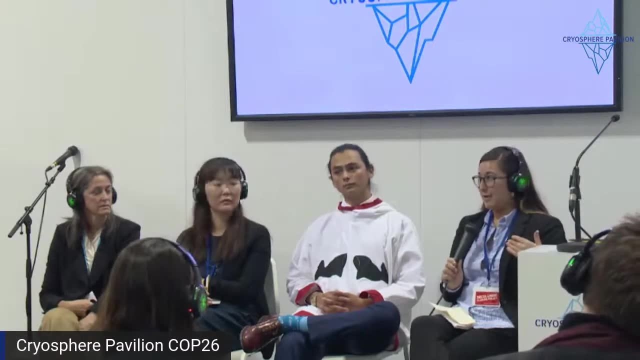 from generation to generation to get a paper that's maybe 20 pages long and that they don't understand, Um that where they saw so much hope and like, oh my gosh, like I'm going to go into policy and I'm going to induce change, like for food insecurity or for clean drinking water or for 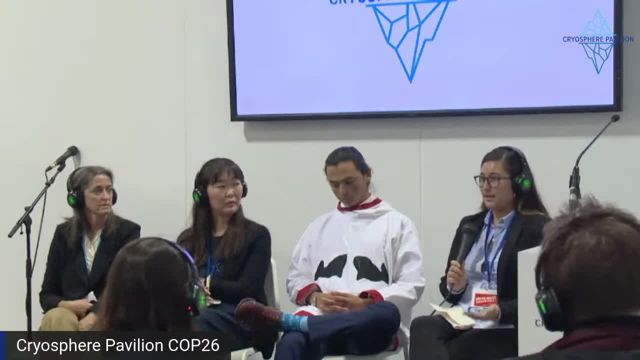 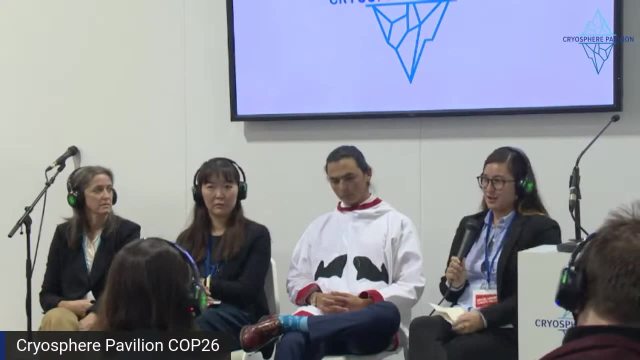 you know, jobs, anything that the indigenous community might need Uh, and they saw this outlet to maybe get something done- is now just a paper that they don't understand. So I think something uh researchers and policymakers can do better uh is just to communicate with 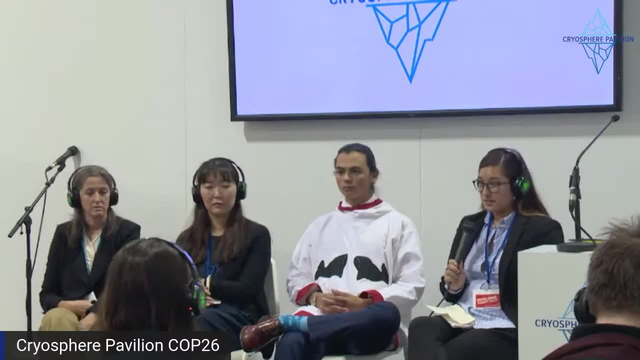 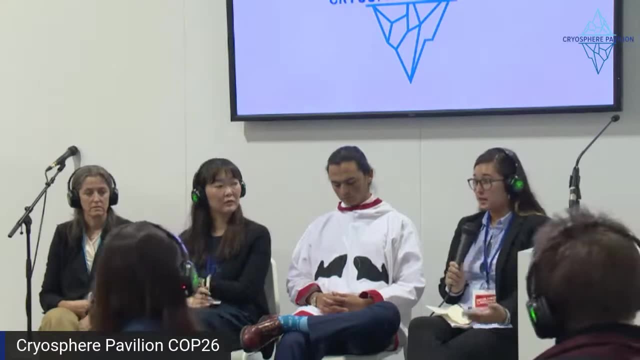 indigenous communities to have uh, a newsletter that's full of pictures that uh is. that exemplifies what your research means in a way that people are going to understand. It's spending extra days in the community during the field research season there. 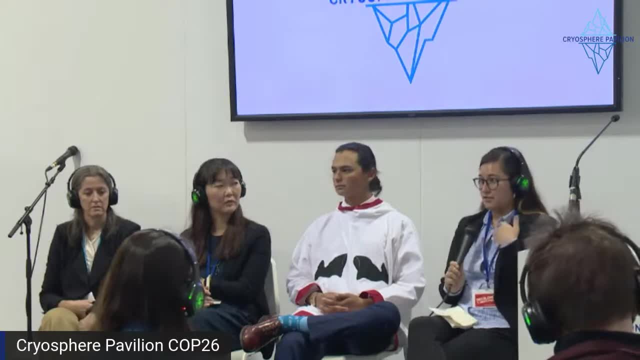 To have a community meeting. get locals in the room and listen instead of just talk and project your own project out onto people. Um, yeah, it's just listening, Like Sue said. uh, it's sharing your research in a way that people are going to understand. Uh, you can go on local radio stations. 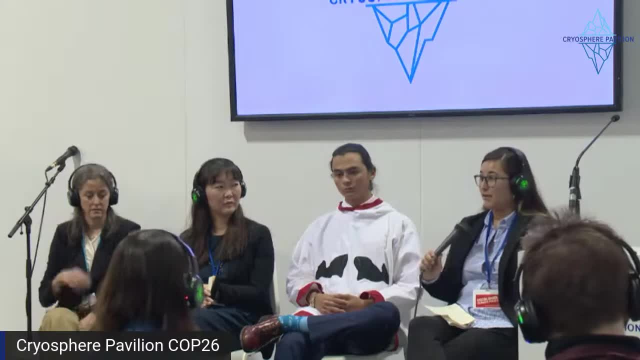 and be like: Hey, this is who I am. This is how long I'm going to be here. We have a community meeting. please, Like I have no agenda here. I'm just here to listen to you guys, uh, and give you. 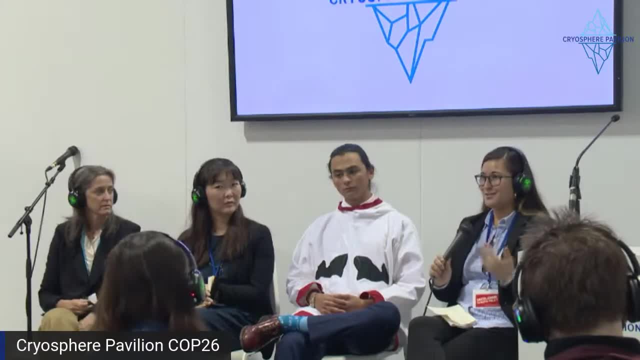 some food and snacks. Um, it's. it seems so simple, but it's so uncomfortable, And I think it's uncomfortable for so many researchers to actually follow through because it's so different than what they're taught in academia. Uh, that's my experience in the U? S and I'm not sure if anybody 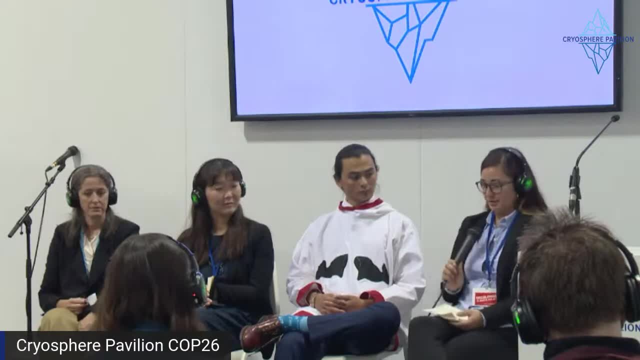 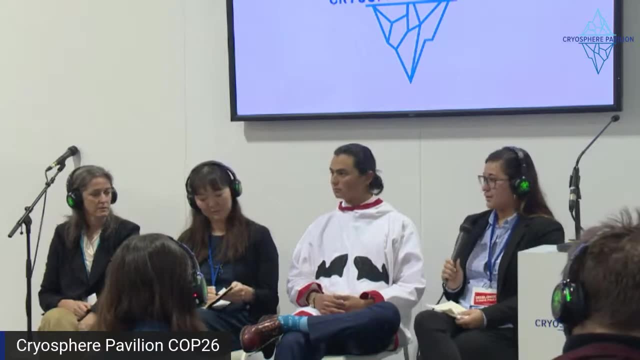 else has anything more to add to that? Um yeah, so we still have quite a bit of time, but I think, uh, we might take some questions from the audience, if anybody has any. but, uh, before I do, I kind. 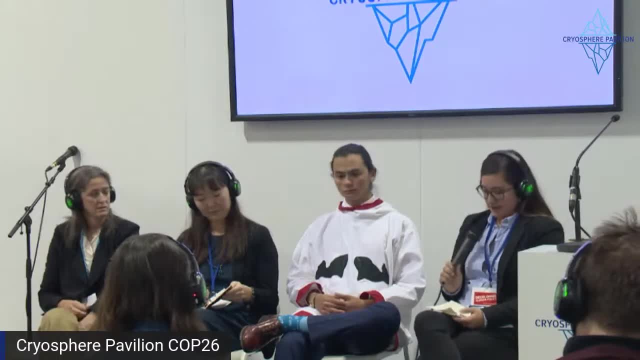 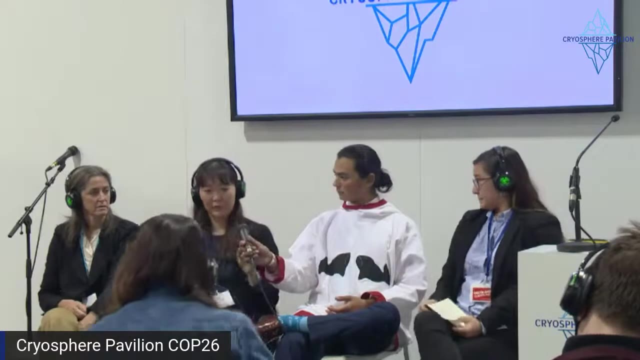 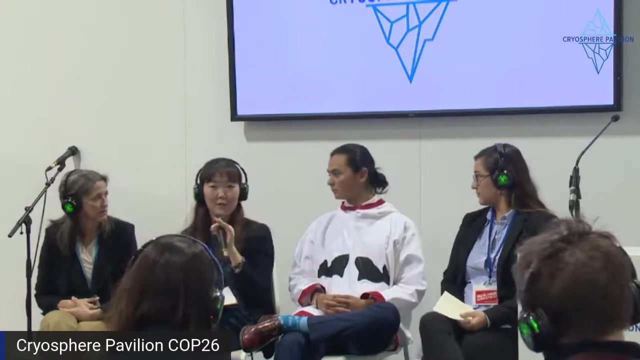 of just want to ask anybody uh about their last remarks and um what the key message is that you would like to give to international policy makers and people in the community. I can just do a quick remark. Um, one thing that wasn't mentioned is about uh also empowering. 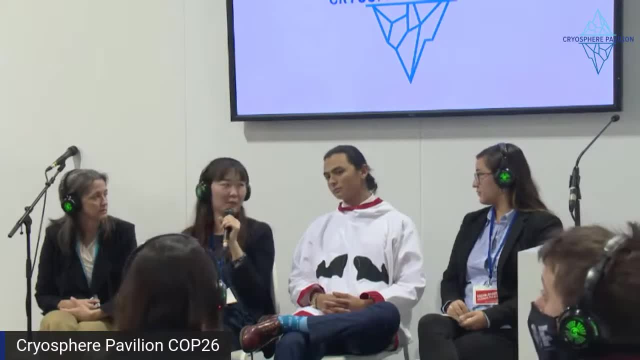 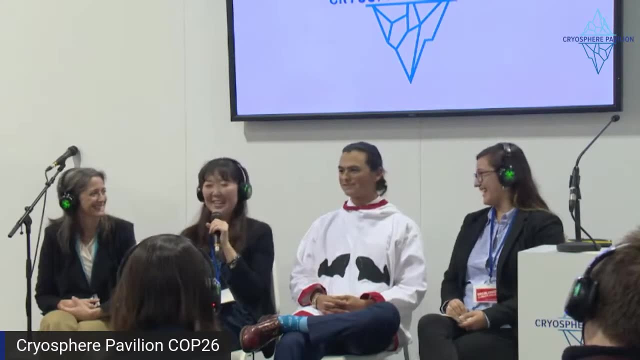 the community, scientists, Like now. at the end of the day, we're living in 21st century. Pretty much everyone has internet, Even my parents. my mom just signed up for Facebook, like a month ago, Um, but she has no idea what I do. 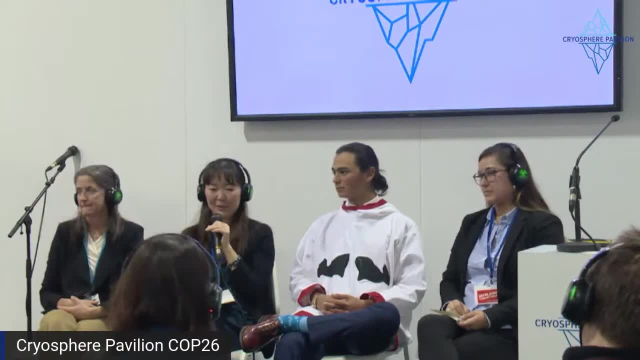 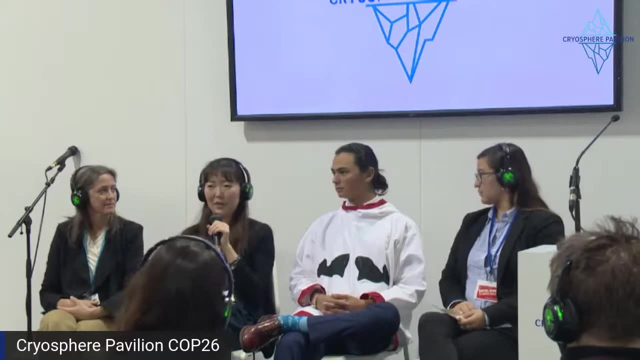 Um, but what I'm trying to say is like: uh, I think we should uh come up with a system. at least I don't really know if it works in our community, but I'm sure there's all this like next gen, uh, young kids thirsty to be. I mean, obviously they care about the community environment. 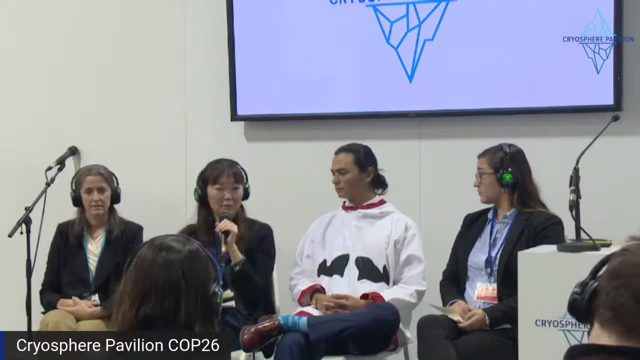 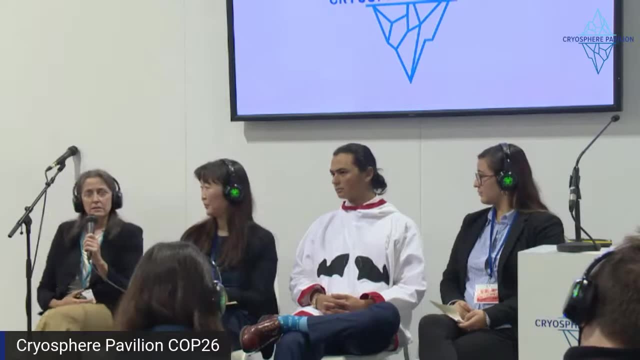 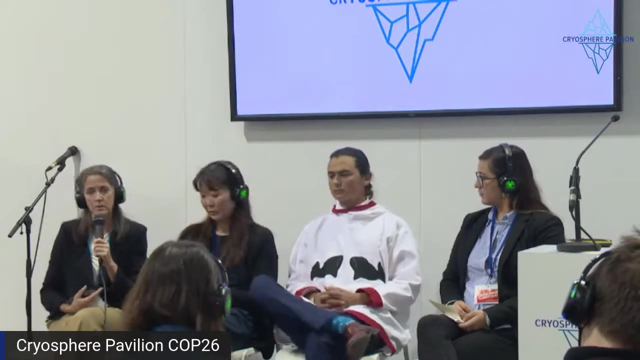 that grew up in it, et cetera, And I think we just need to empower it and like, make them the scientists And uh, yeah, I think in terms of Arctic policy, I think, um, I guess, for people who are decision makers, I think listening more to the voices of the folks here and recognizing 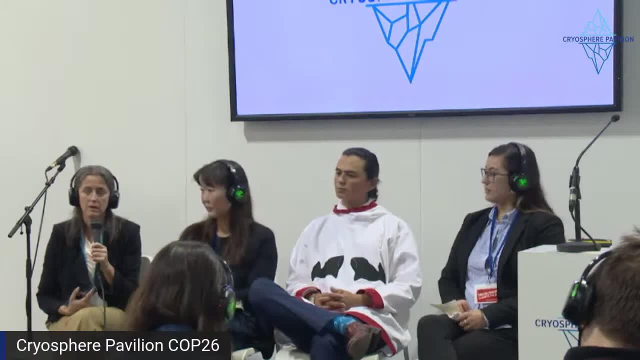 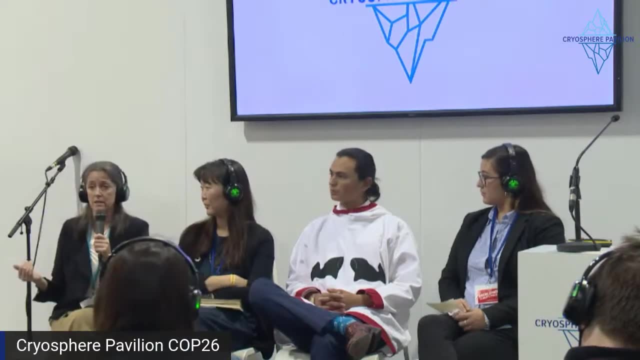 um, you know, when we think about climate loss of land as a result of climate change, the Arctic often is not a part of that conversation. Um, we think about island nations, and that's critically important And I'm glad that those voices are starting to be heard. but um, communities in 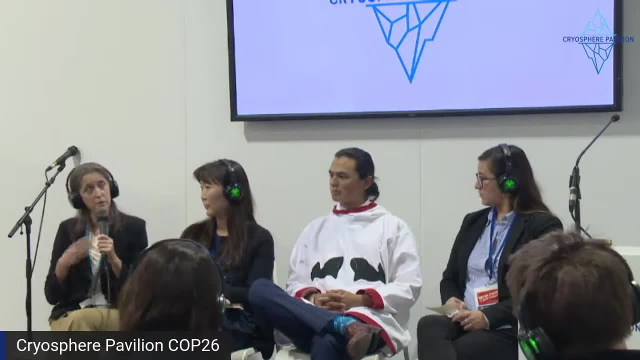 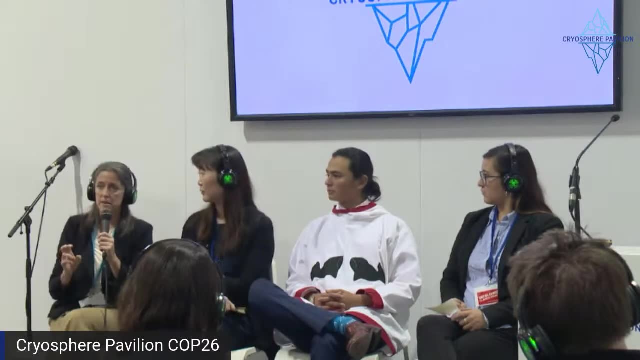 the Arctic are losing their land as a result of permafrost thaw, as a result of erosion, as a result of fires, and all of these things are connected. And so I think getting this, these um sort of slow onset events um in Northern regions, into the conversation about loss and 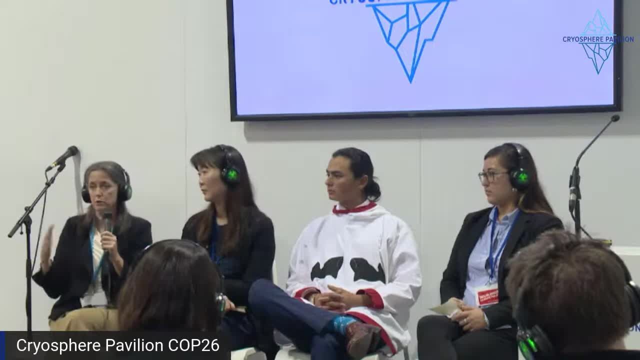 damage is is critically important Um in the U S w. there's also right now these erosion. permafrost thaw is also. there's zero climate change adaptation planning um in our country And so there's just sort of no, no leadership at all and no guidance at all. So I think hearing 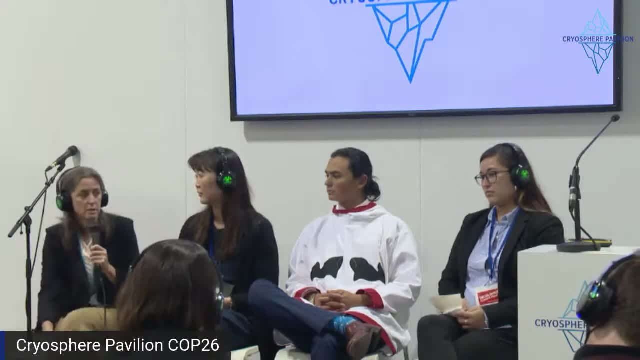 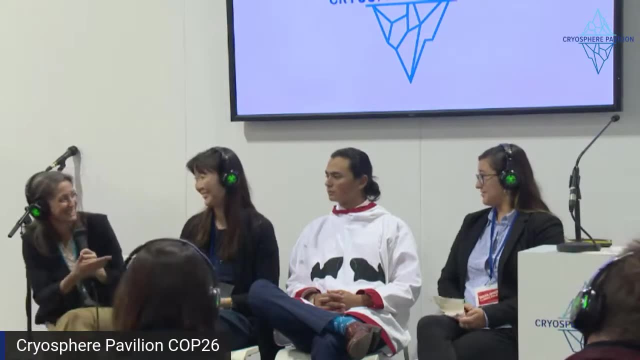 these voices getting a better understanding of what's happening right now on the ground. I think is really important. And then I think, as a scientist, um, yeah, I guess I'll say I'll stop there, I'll shut up and listen now and pass this on to. 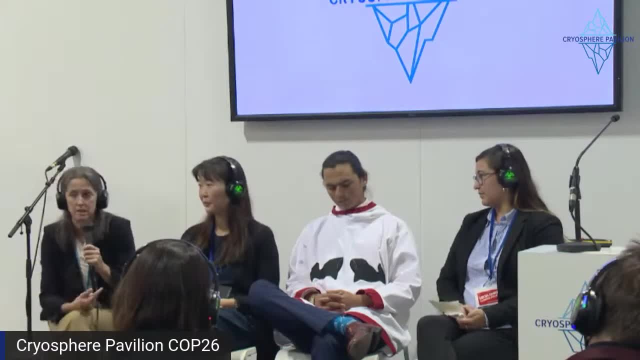 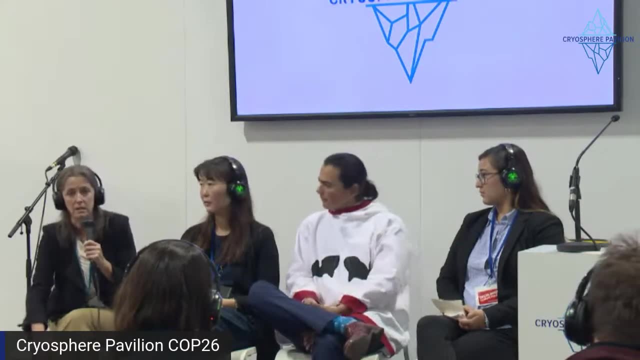 others, because I really, um am fortunate to have this opportunity to be on this stage, but also to learn from um. you know, Darcy and I have worked together for a long time, but just to taking that time to listen and to learn, and being humble and being uncomfortable. 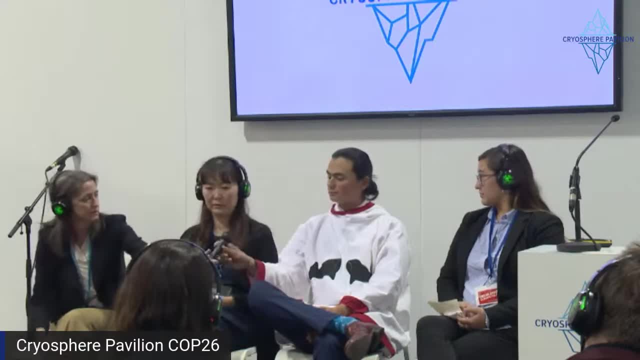 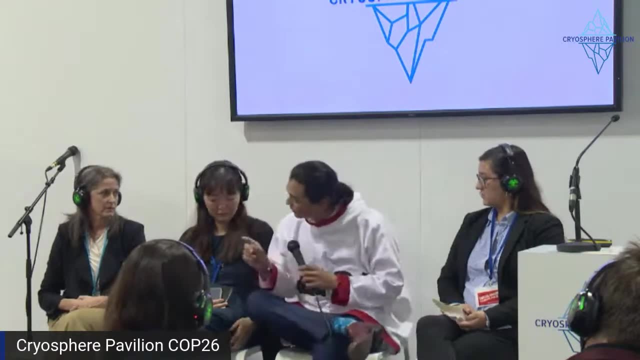 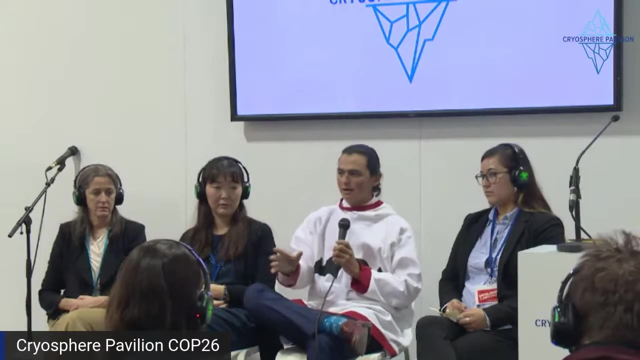 at times, um, I think is really important. I think that what you said is really important, Um, in terms of um, ensuring that there's listening happening, ensuring that there's communication happening between indigenous communities and research. I mean, I I understand. 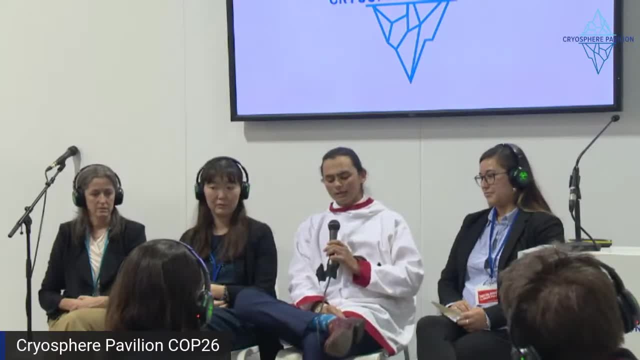 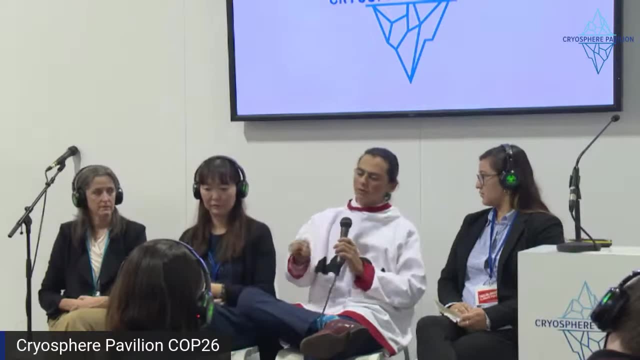 I'm talking to a majority of researchers here And, um, I think really what's, what's critically important on the research side is that co-development is making sure that when it comes time to publish a paper, when it comes time to write a paper, when it comes time to 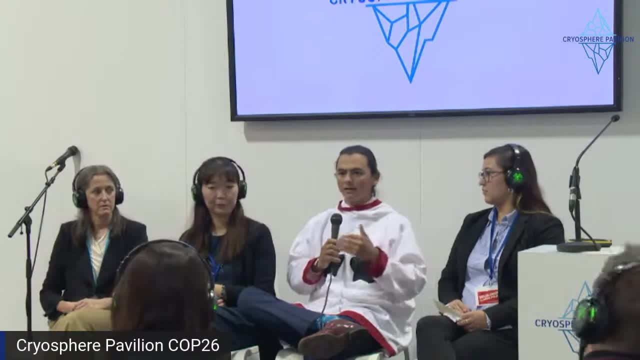 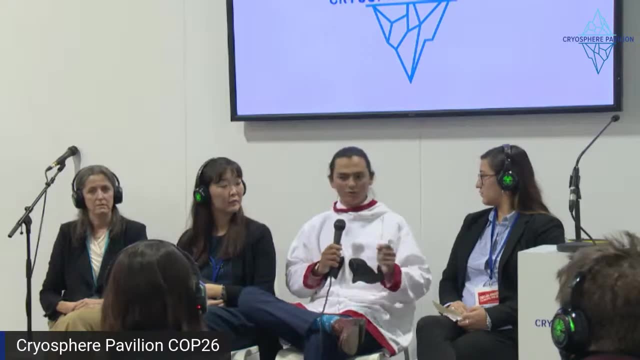 research, a topic. that topic is informed by indigenous views. I understand that sometimes this won't be the case, but in the majority of the things that you write, I ask you to reach out to the community before you submit an abstract or before you submit a proposal and you say: 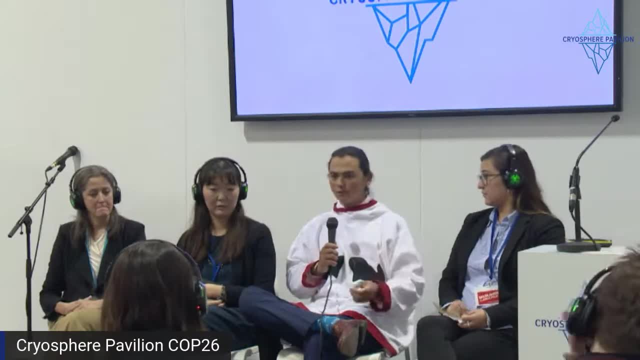 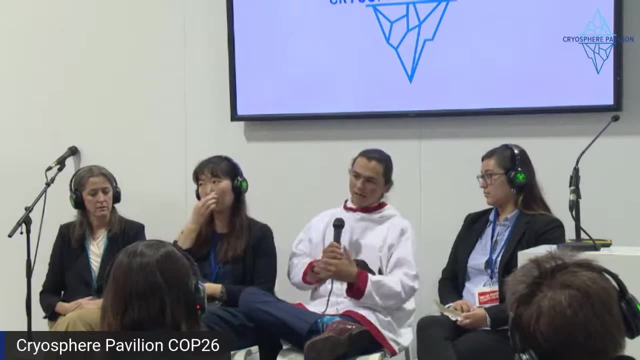 what? these are some ideas that I have. What do you think? Foster those relationships with communities, foster those relationships with individuals, so that they're in a position to be able to help direct research towards the issues that are present on the ground. Um. 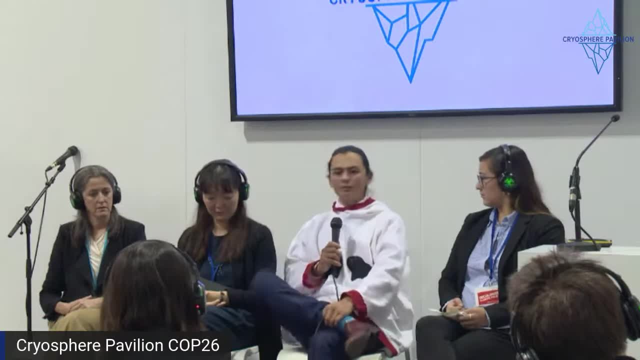 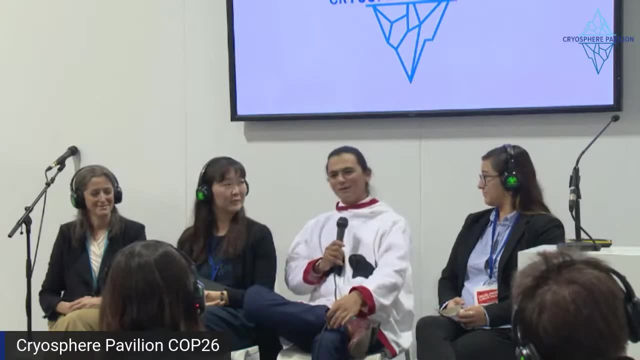 there's. there's a saying that's in our community, which is that indigenous peoples used to not trust researchers. Uh, but now we just can't tolerate them. Um, and that that's. that's partly because sometimes research can get a little bit. 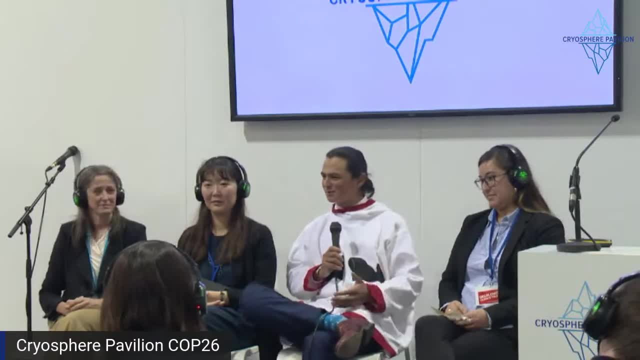 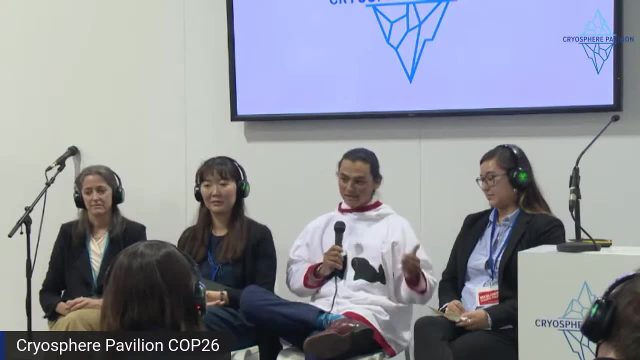 esoteric. Uh, I'm sure anybody who's spent more than five hours in front of Google scholar uh knows that sometimes it can get a bit into the weeds, Um, and so that is important: to get down to the bottom level, but it's also important to have broader applicability. So making sure that 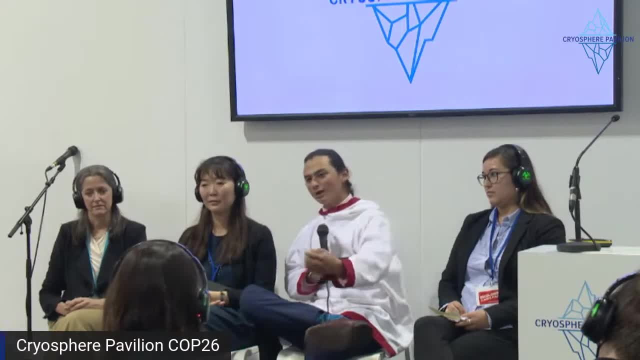 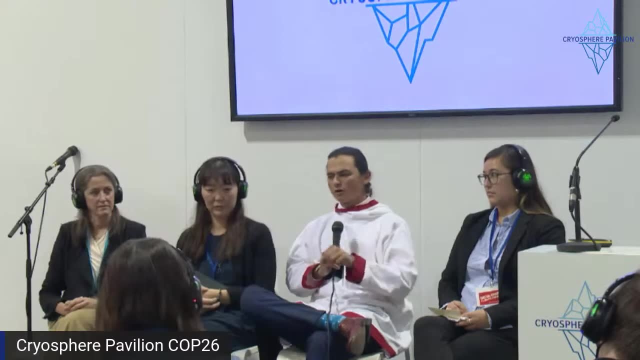 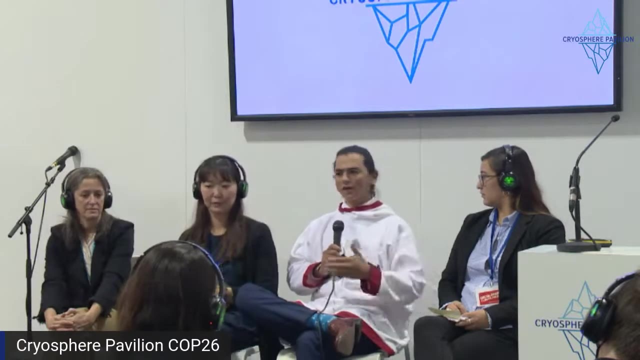 when working with indigenous communities, there's a clear applicability to that community, Um, in terms of policies. right now, you're watching as carbon markets are emerging. We're seeing the commodification of carbon. before it was um oil, before that it was gold, Now it's carbon, Uh, and in order to ensure that there's protection, 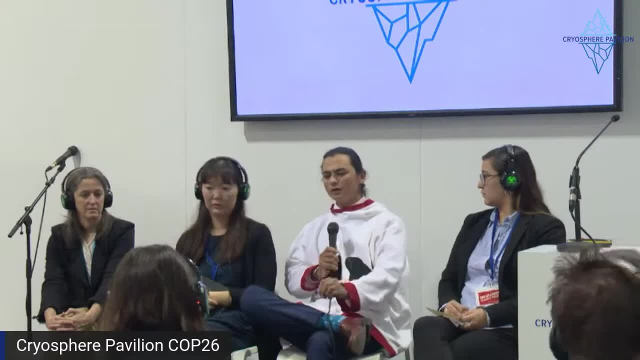 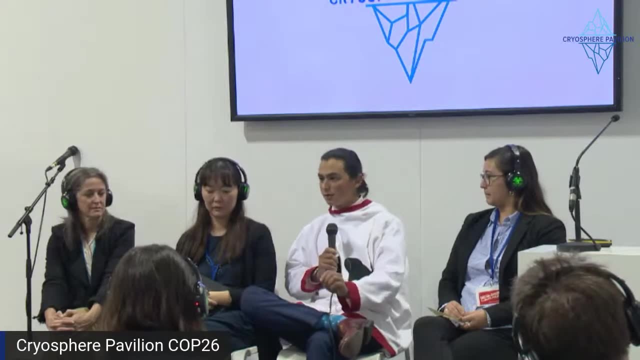 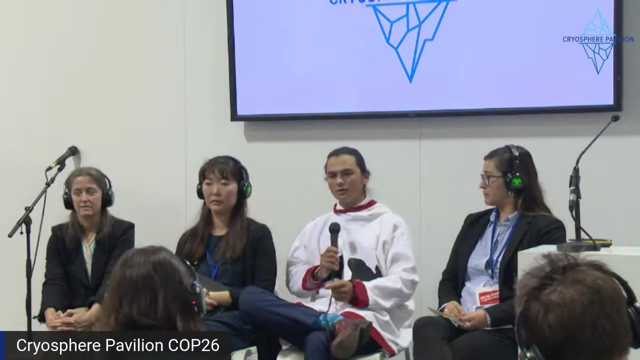 for indigenous peoples and our environment. um. we need to really focus on what's being talked about in article six. Um, that means Ensuring that there's human rights protections and environmental rights protections. That means ensuring that there is full and effective participation for indigenous communities when 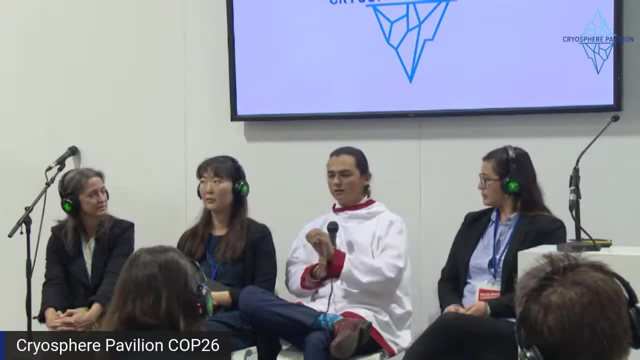 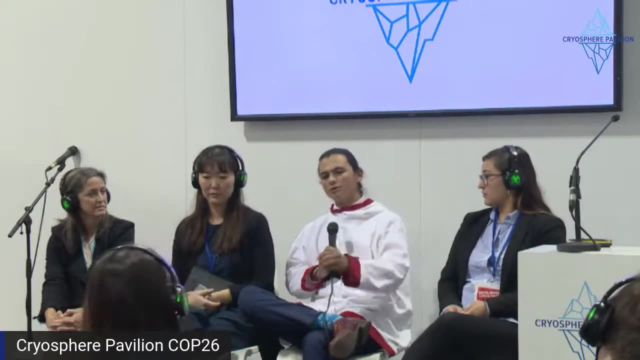 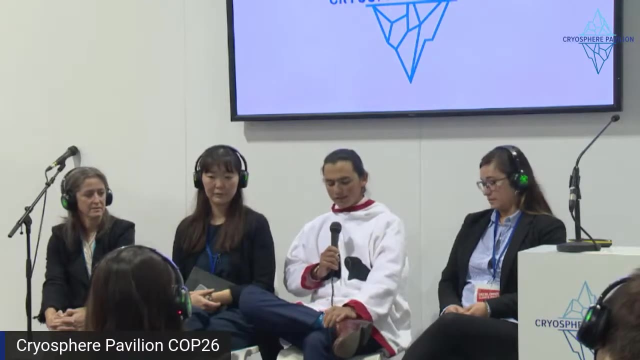 it comes time to designate these sites, And it means making sure and and participation is not consultation, again, it it is a right of refusal on a policy, Um- and then also making sure that there's redress mechanisms in the event that such policies fail. So I I guess in in closing um. 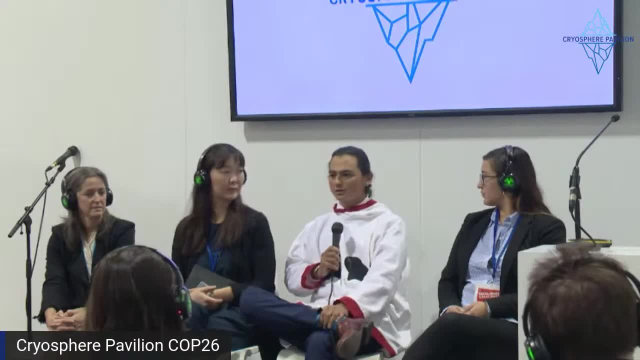 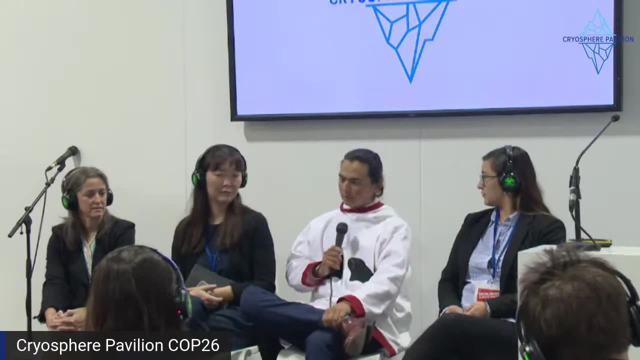 I, I ask all of you to to go about your research and to to just ask the simple question, one of how can I help? And then to explain how this relates to me, uh, in our indigenous communities. explain those, those relevancies, and ask those questions And I think you'll be surprised by by your results. 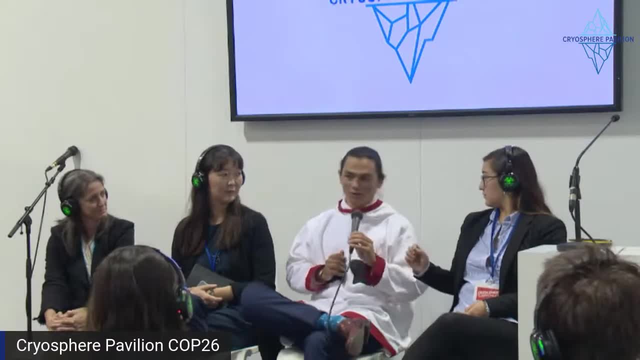 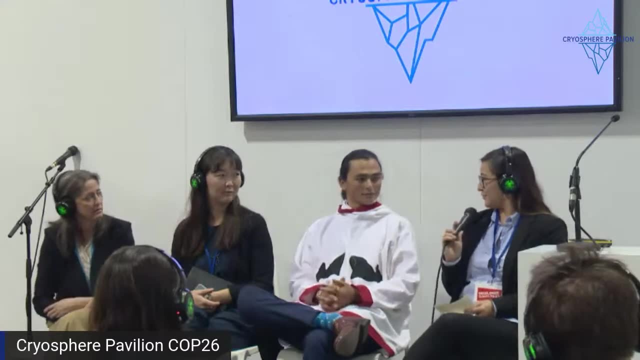 So thank you all for um for coming, and I'm going to give it to Darcy, Yeah. So uh, before I give my short answer, um, do you want to explain what article six is for people who don't know? 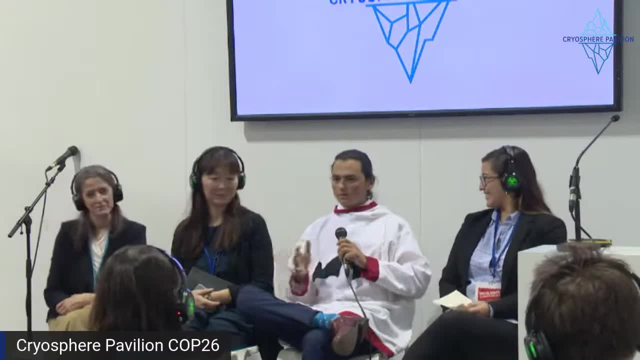 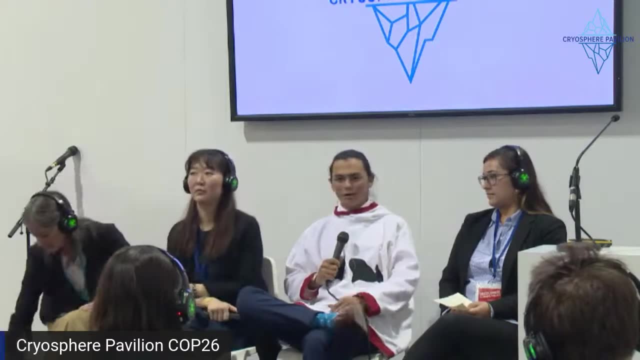 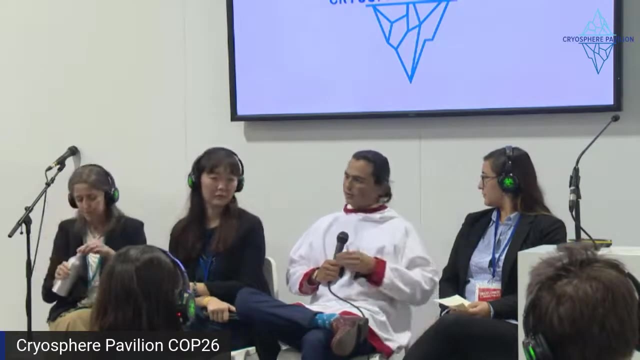 So article six is the part of the convention here that is regarding carbon markets, um, figuring out. So I'm sure all of you have heard about cap and trade or carbon markets or things like this. Essentially, what it's saying is that I'm going to run my car here or my oil. well, 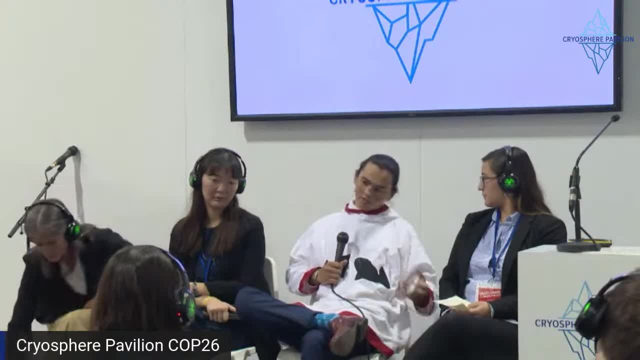 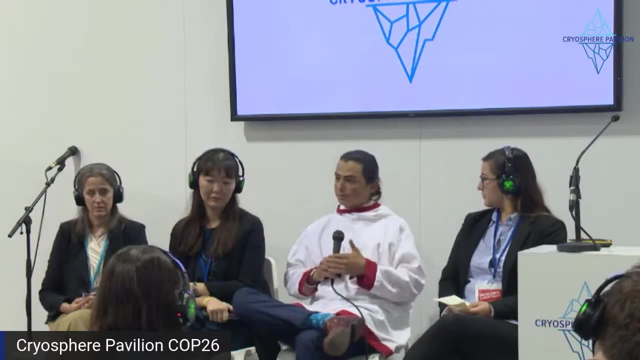 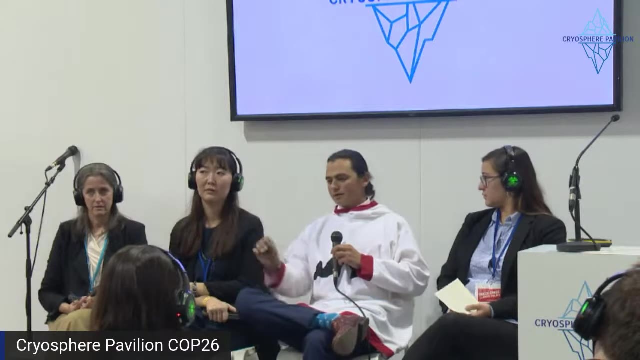 here, And then, in order to offset the carbon that's going to be emitted as a result of this production, I'm going to set aside this land over here, And there's concern for this for indigenous peoples and environmentalists alike. Uh, in the sense that land that set aside, um, to be considered a carbon reserve can be very 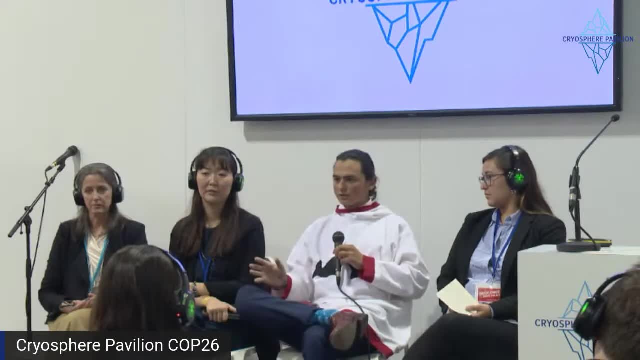 restrictive on what happens. uh, in the United States we have something called the park service And what they do is they set aside line land and they call it a preserve And the mandate is to preserve the land And under a lot of doctrines of land management we don't see people as part. 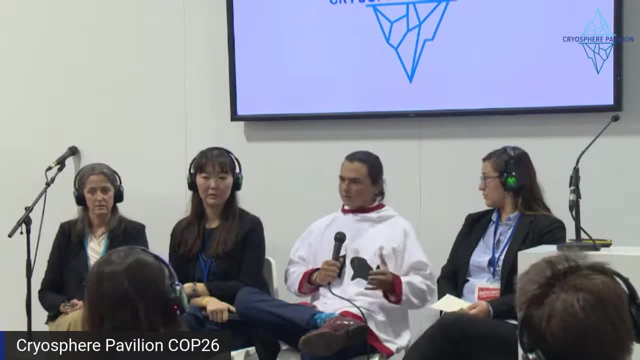 of an ecosystem, And that's- that's a fickle thing. Yes, Western civilization really isn't part of an ecosystem. Indigenous communities are We're. we're the stewards of our environment. We're really the only ones that can call the forest. 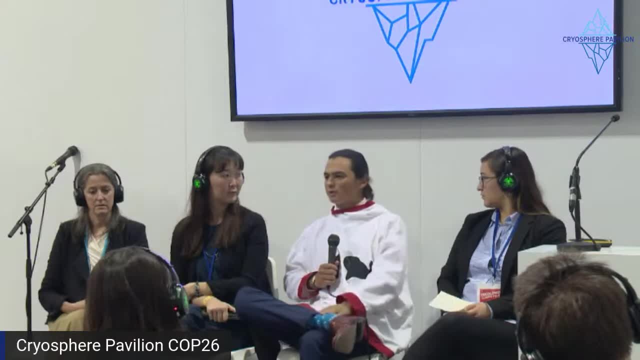 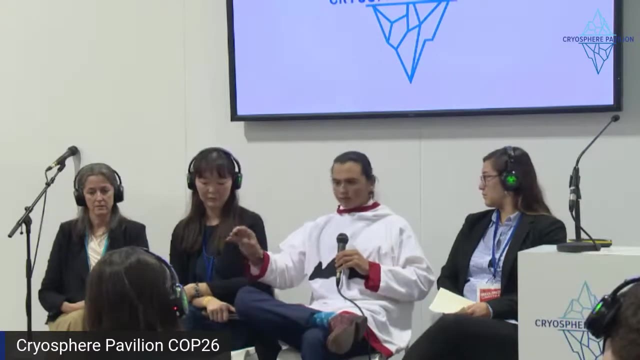 our home And we are the ones who do population management, clean up our forests, make sure that there's controlled burns in certain communities and in certain areas, And so when you pull us out of an environment, you, you can see the changes to the ecosystem. And so, uh, in set asides we want. 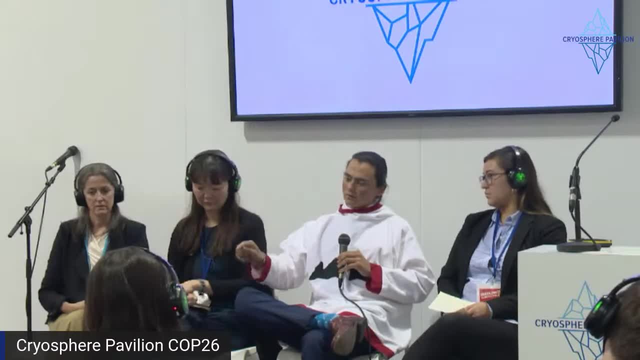 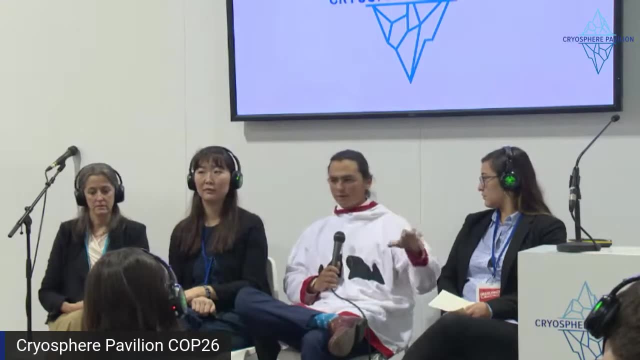 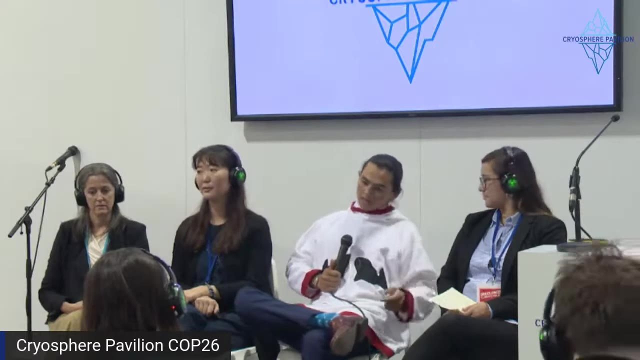 to make sure that subsistence is able to continue. We want to make sure that our rights to our way of life are not infringed, And then, in terms of development, we also want to make sure that we are equals at that table. we're able to say no, this can't happen here, or no, this can't happen this. 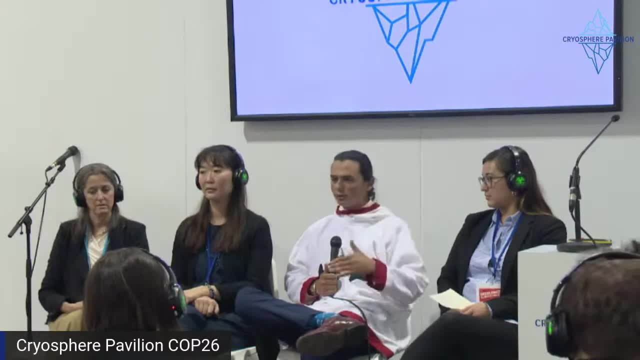 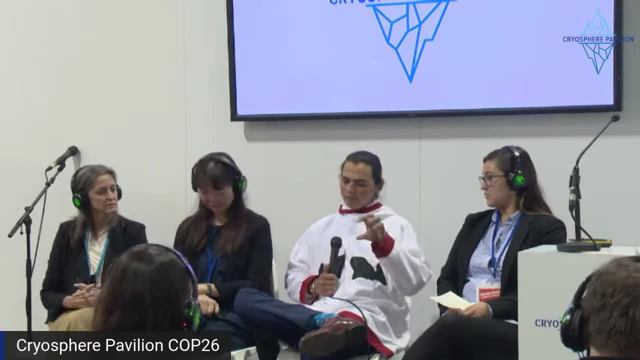 way. This has to happen according to these set, these uh terms that we lay out, or this happens with a profit sharing agreement or something of that nature. Uh, so we want to make sure that these are safeguards that protect our rights and protect our lands, uh, and. 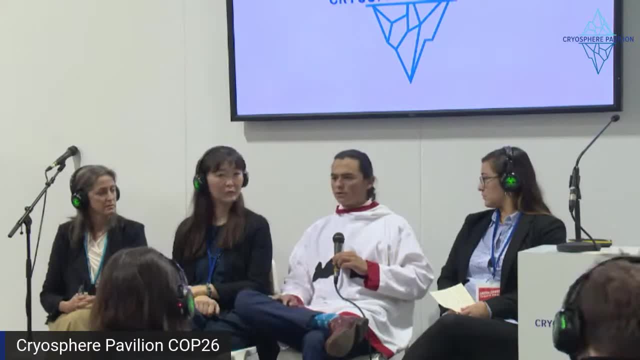 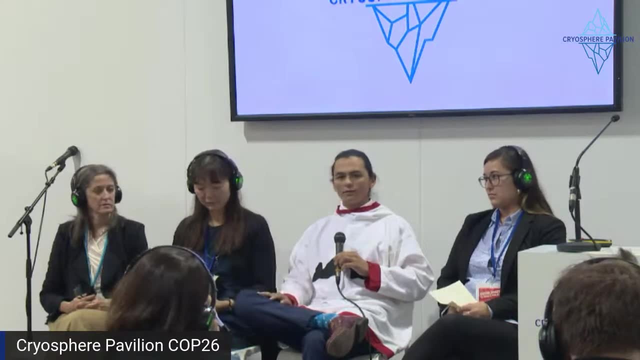 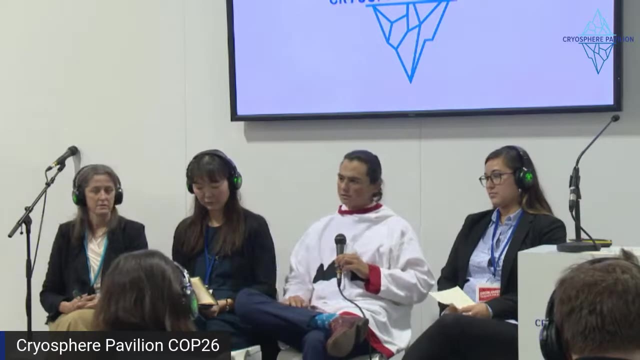 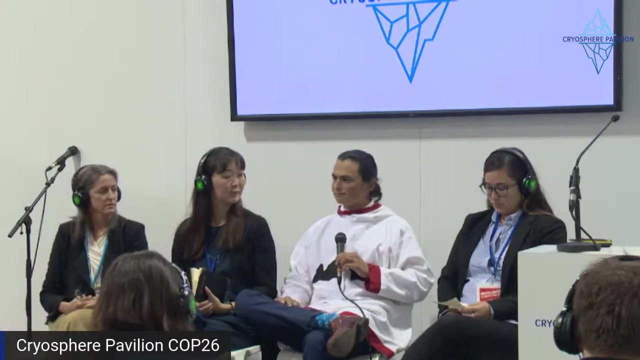 And really, at the end of the day I think, enforce indigenous sovereignty, the idea that we have the power of decision over our lands, over our ways of life and over our peoples, And so that's really where those concerns come about, with Article 6 and kind of how that fits into this larger picture of trying to build a new world that's based in clean and green energy. 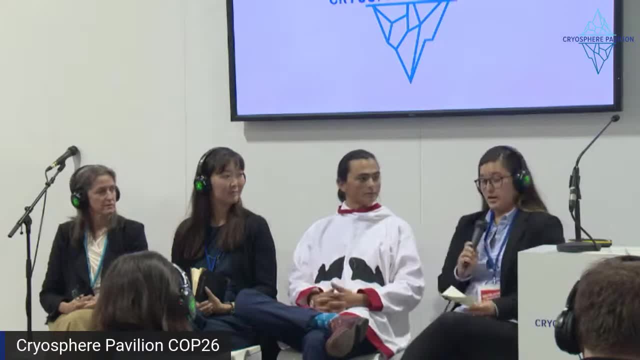 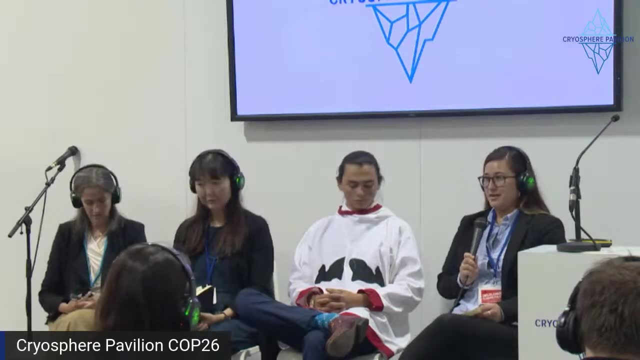 Yeah, Yeah. so Article 6 is a huge topic of conversation, or it should be here at COP. So if you don't know too much about it, I'd encourage you to delve into it. Yeah, it's a big issue. 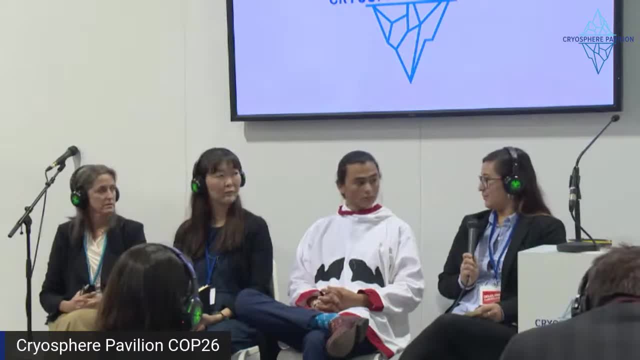 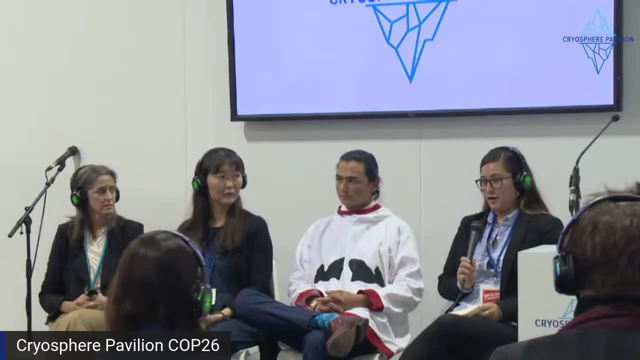 I think my takeaway message wouldn't be too different than everybody else's. It's: yeah, do ethical research. Care about people before you care about research. At the end of the day, we're all human beings. We're not all scientists. 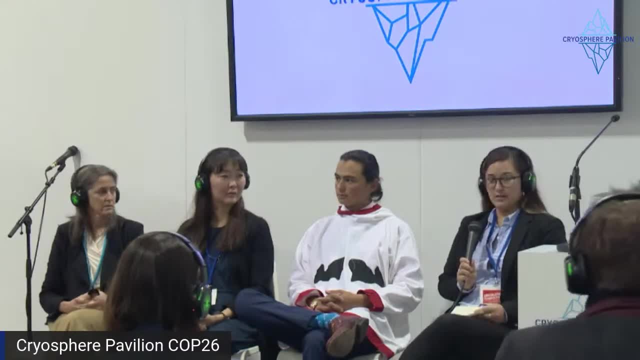 Scientists and indigenous people are living on the land and we have been for many generations. We are very in touch with place. We know our resources and the land that are on, the resources or the resources that are on the land, excuse me- insanely well. 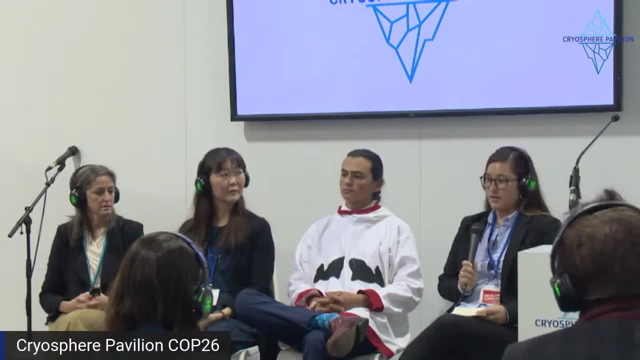 We're very in tune with what's happening. We have a lot of knowledge and we're again the ones feeling the impacts, I'd say, the most heavily. So make sure it's ethical, Make sure your research is applicable. 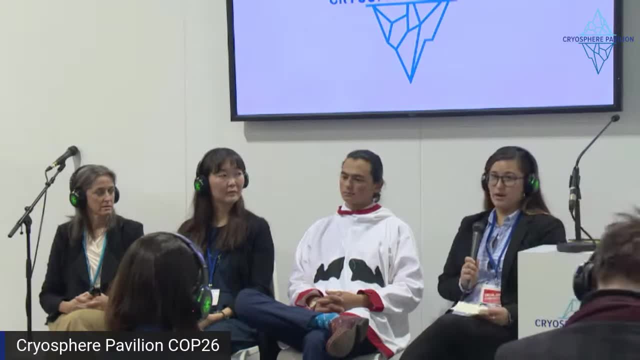 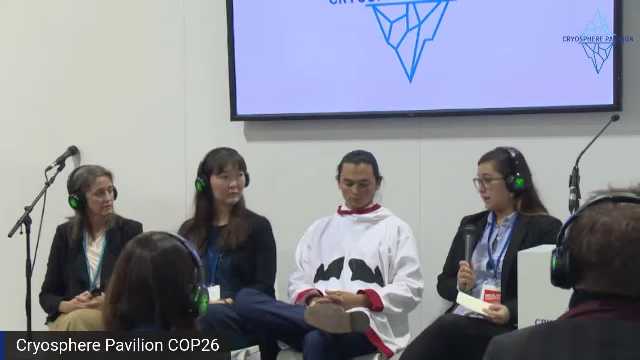 Like Sam said, work with communities, Not online, Not on them, Not alongside them. Work with them, Include them in your research, Give them financial compensation, Give them the credit where it's due, And realize that there are different knowledge systems and different ways of knowing and different value systems that are just as valid as Western ones, if not more. 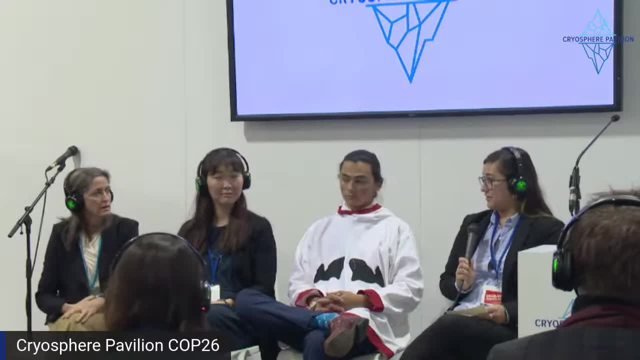 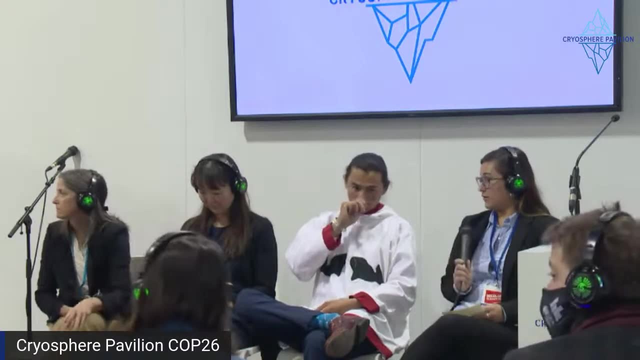 So, yeah, I guess that would be my takeaway message. I'm not sure how much time we have left, but we might have some time for questions. But I think that's it for us in terms of questions. Thank you very much for all the questions that I have. 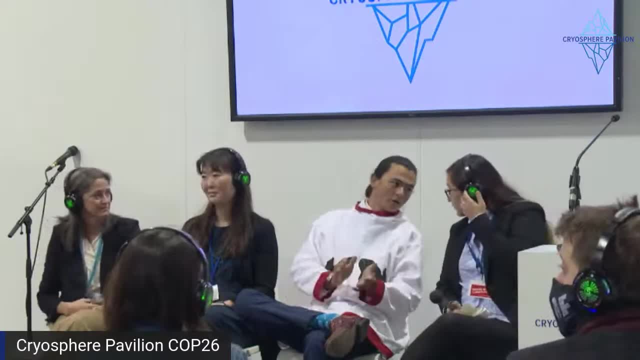 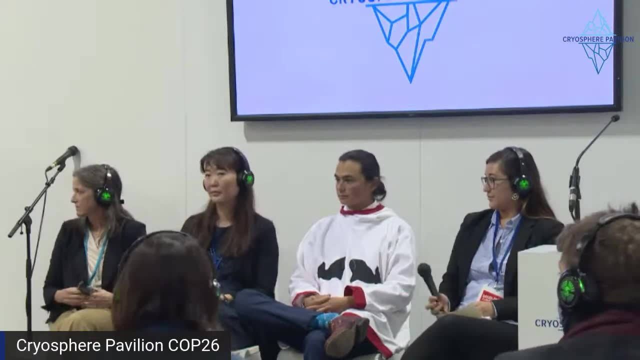 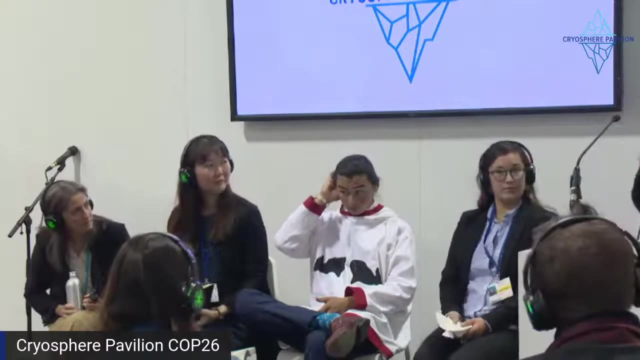 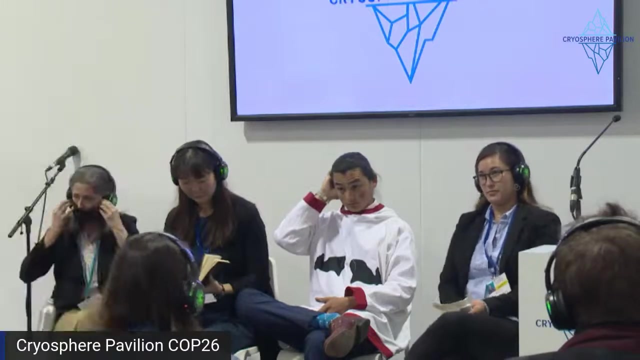 So thank you, Thank you so much, all of you. That's been another absolutely fascinating discussion. We do have a little bit of time for questions, So I'll just check if we have any of those coming in online, And otherwise we definitely, I think. 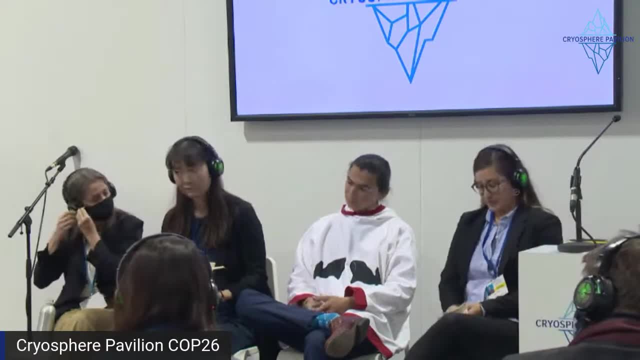 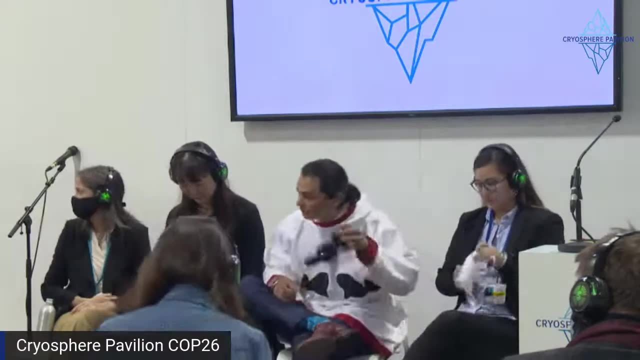 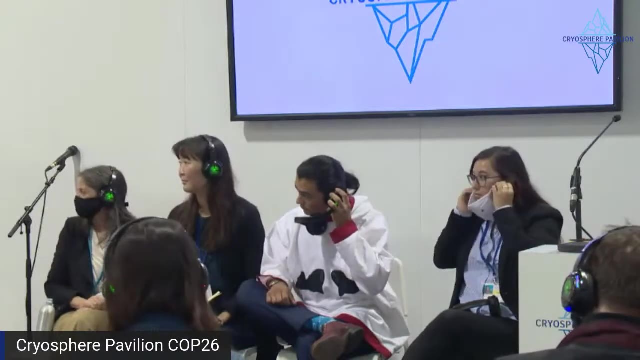 have a lot of time for questions. We do have some from the floors. Would you like to come up to the microphone and ask a question? Sure, Can anyone hear me? I don't have the headphones on anymore, So I think there was an announcement yesterday and I'm probably going to get the figure wrong. 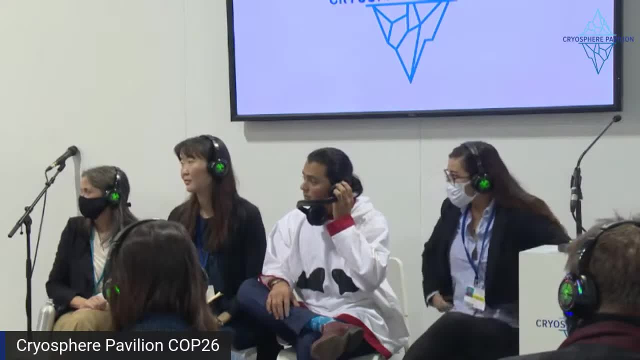 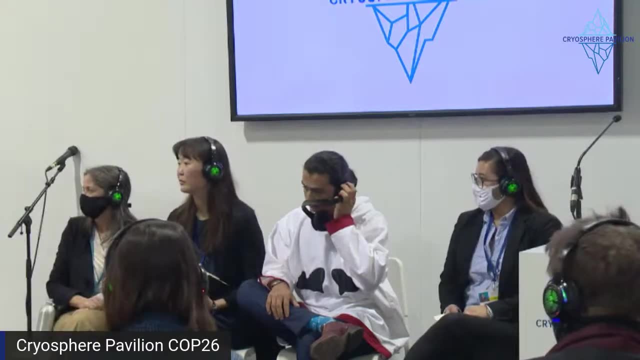 but something like 1.7 billion for supporting indigenous people to get land tenure rights, And I don't know how much. I don't know kind of which indigenous people that affected, but I just yeah, super interesting talk And thank you all so much. 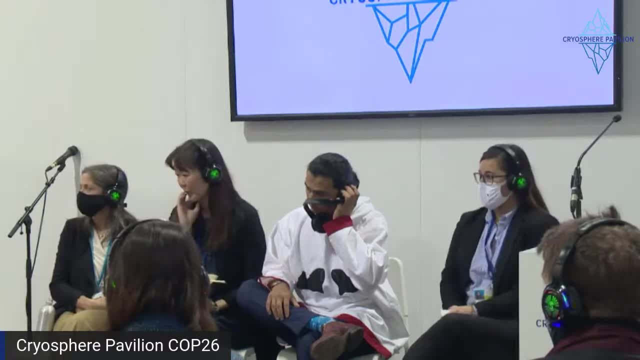 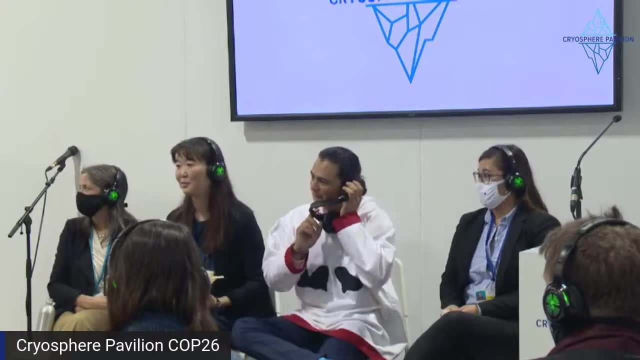 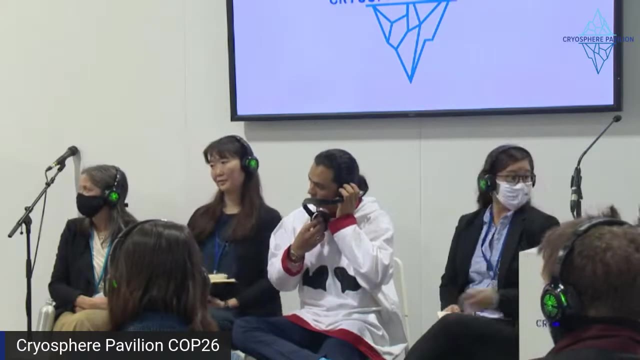 But I wanted to know your perspective on those kind of financial big pledges and commitments versus kind of what you've talked about in terms of actually working with you know, policymakers coming to you and involving you in those discussions, and kind of. do you what do you think about that financial announcement and what it will actually do for indigenous people? 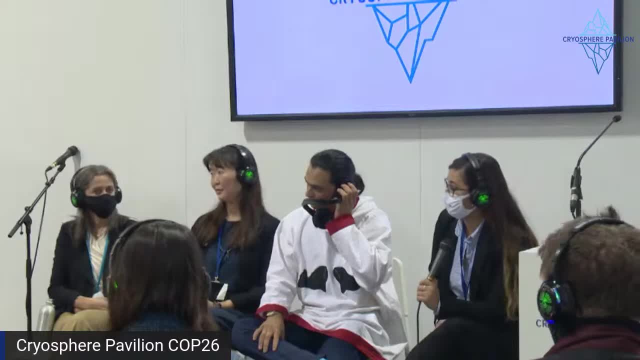 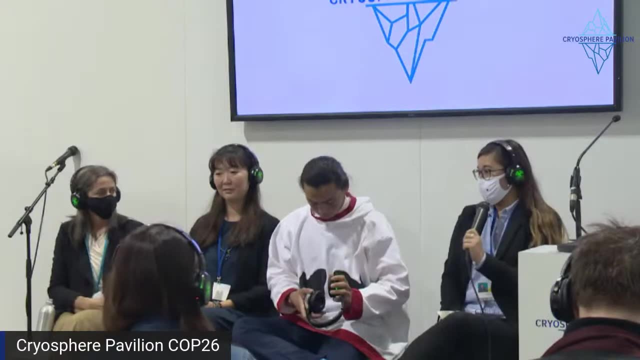 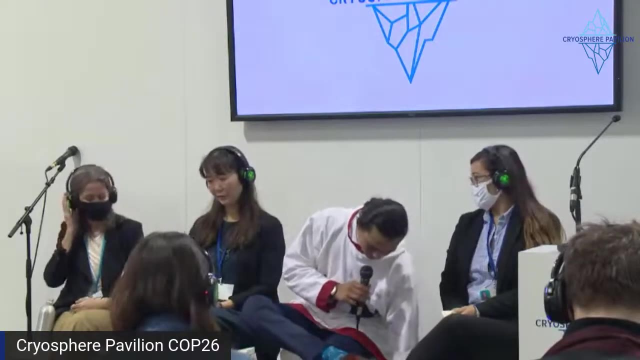 And how much can that solve the problem versus what you've already talked about? Yeah, so I'll just say really quickly: thank you for giving that money to indigenous people, period. You know, I think that when it comes to large donations, money is always a good thing when it's spent, right. 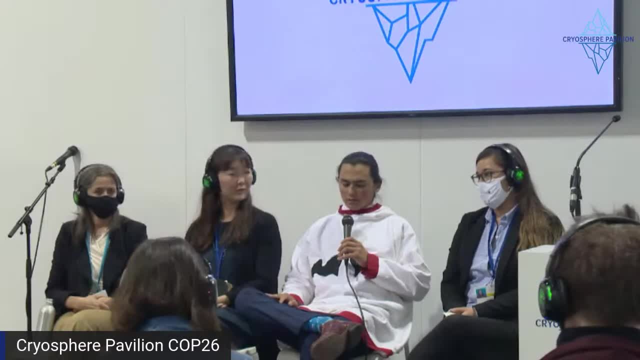 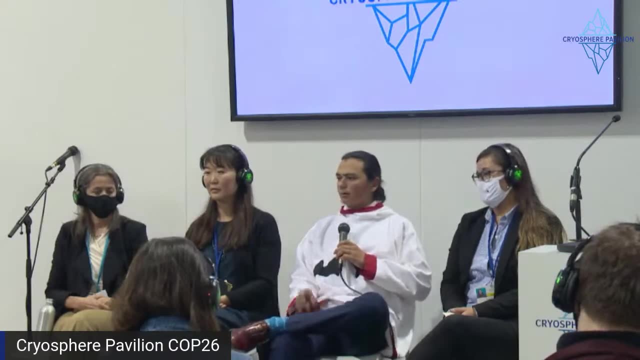 Money is a good thing because it helps us enact our policies. You know, there's this strange idea that without resources you can't actually be sovereign, And that's a reality for our sovereign Communities in the US. But in terms of large donations, they're big numbers. 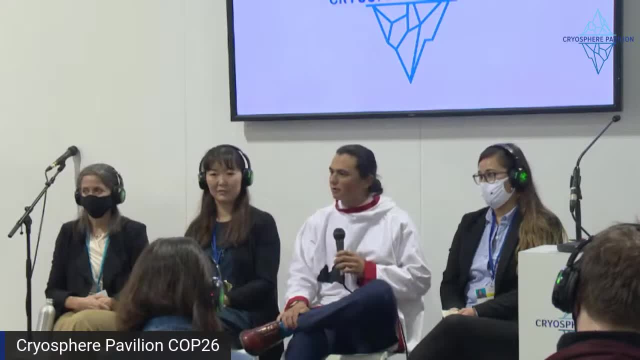 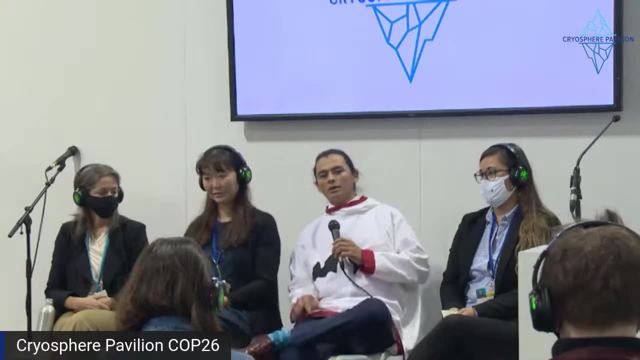 They're big numbers that go to big organizations that rarely end up on the ground. The best way to make investments in indigenous communities is on the ground. It's not from the top down, It's from the bottom up. We know how to manage our land best. 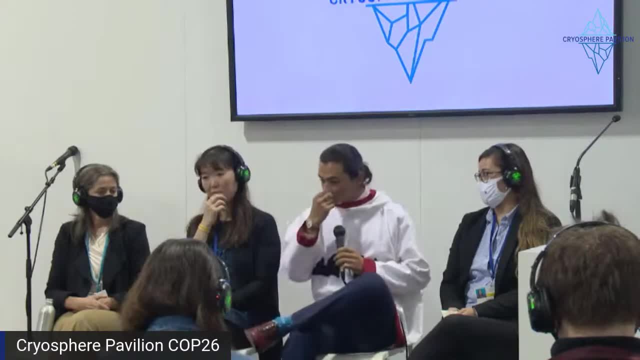 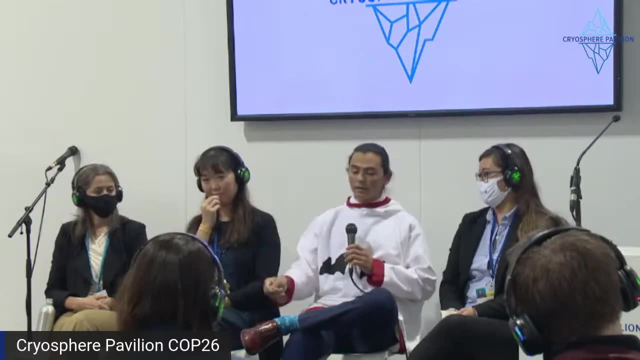 We know how to manage our people best And we know how to affect change for our community in the best way. We don't need organizations like Greenpeace or Anything else coming in and telling us, one, how we need to live, or, two, how we should be spending resources, or, three, spending resources on our behalf without our direction. 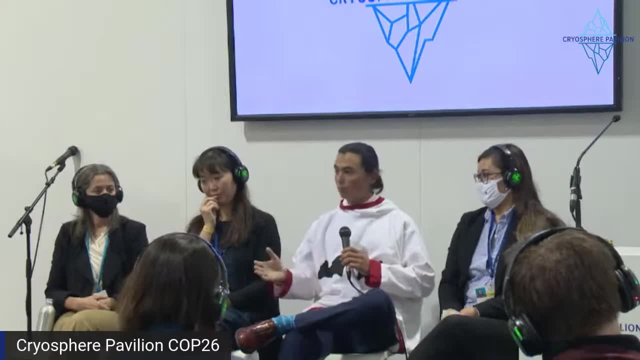 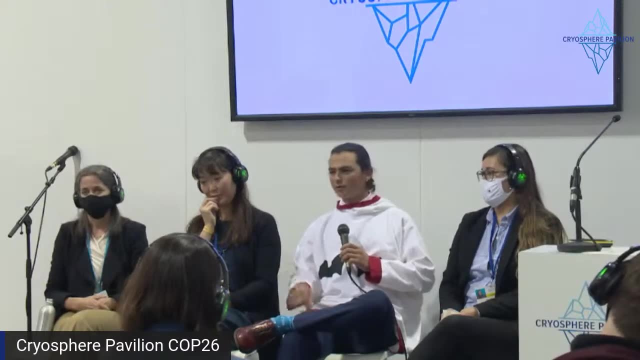 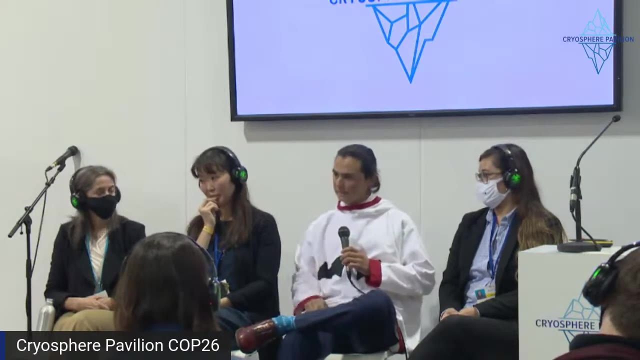 So large dollar pledges Wonderful, They do good things, But that money rarely ends up on the ground with our communities And the better place for it is is making those direct cash infusions to communities who are struggling with needs, And that's really what I, what I think there. 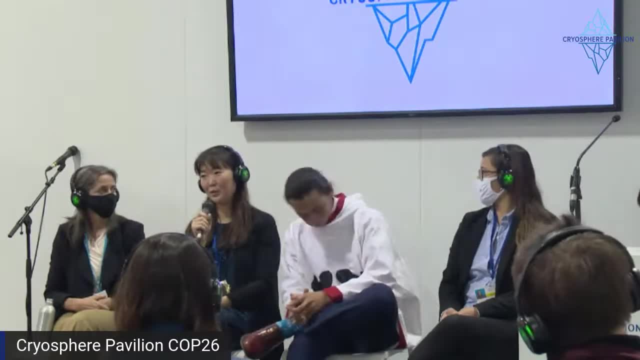 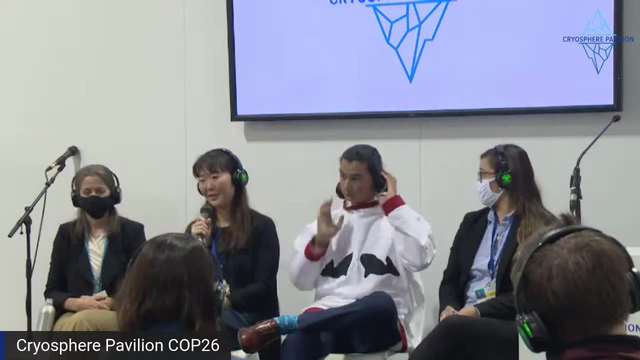 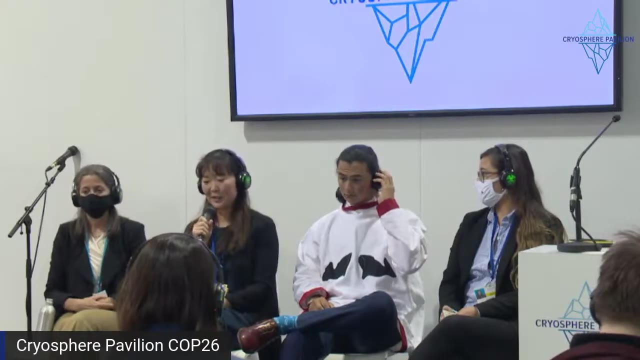 I am very pessimistic. I don't think any of this pledge is going to come to Russia. It started there and already provided some example where even our like community environmental program was kind of shut down because they can't receive any foreign money. So that's the starting point. 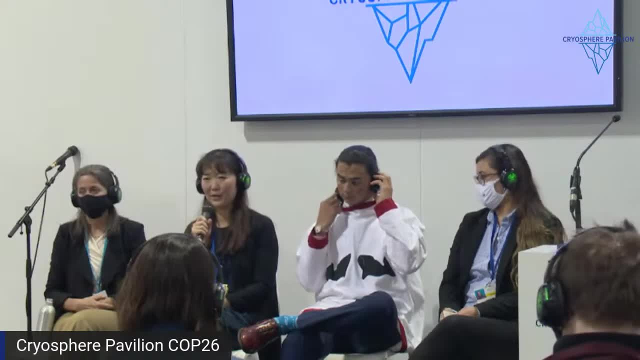 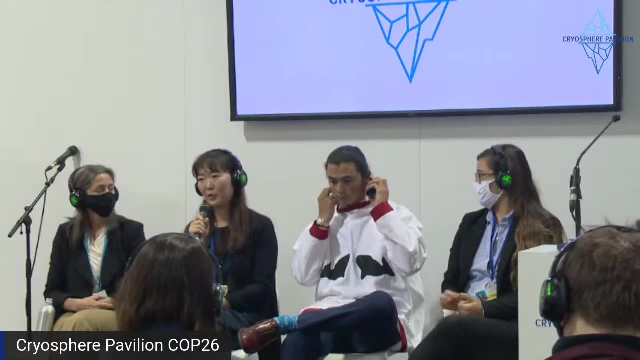 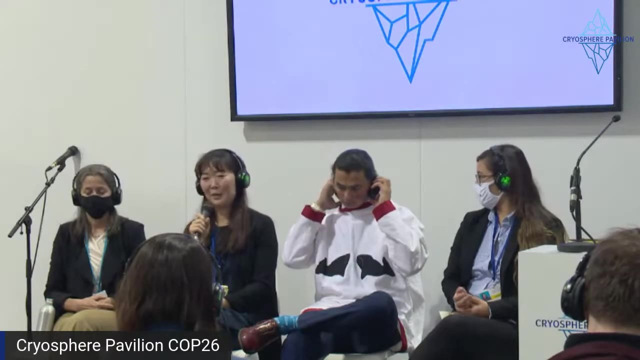 And then, yeah, just grassroots work with small organizations. So I'm personally part of two Philanthropic organizations and we only finance, you know, small, small community around community on the- I don't know if you would formally say- organizations. 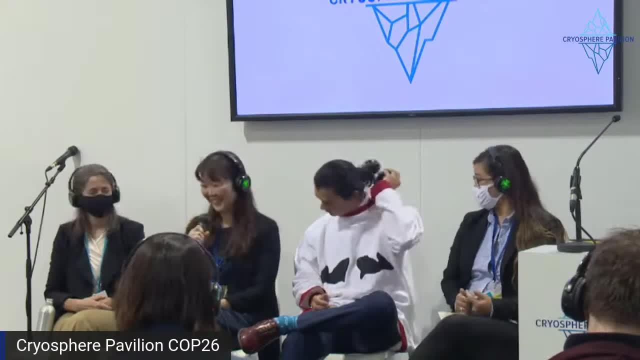 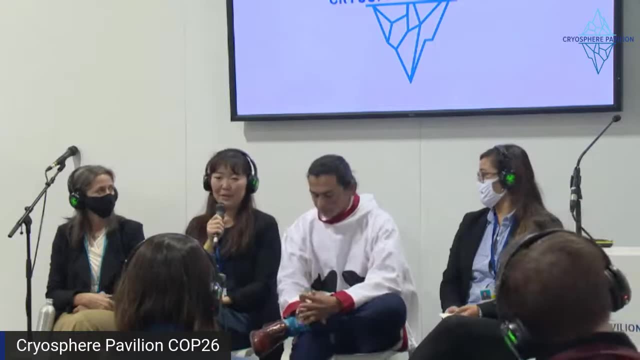 It's, like you know, community led initiatives. Yeah, That's a lot of work to make sure that it. all you need to co-create Like. my main thing is all about co-creation, Otherwise, you know, we're not going to go any like far. 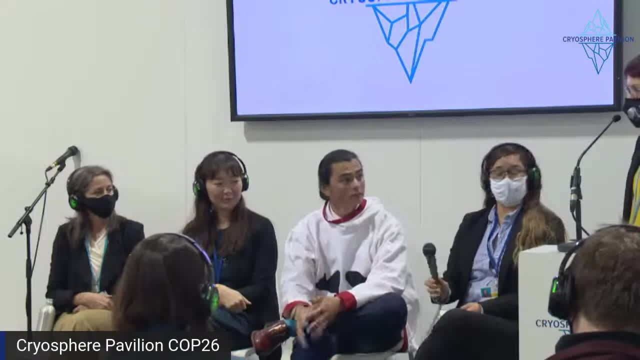 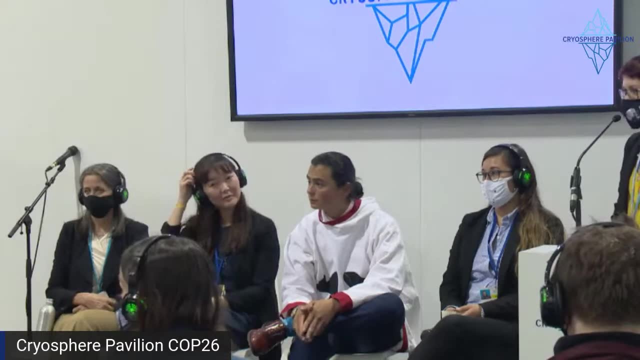 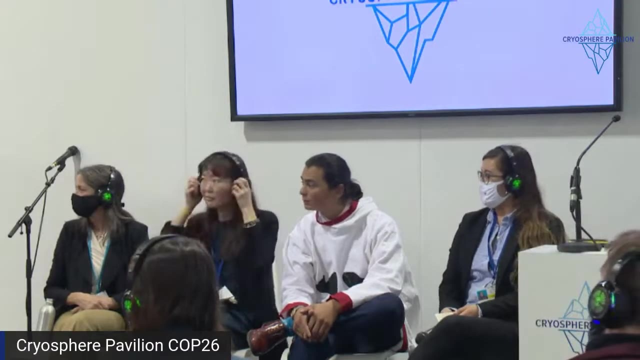 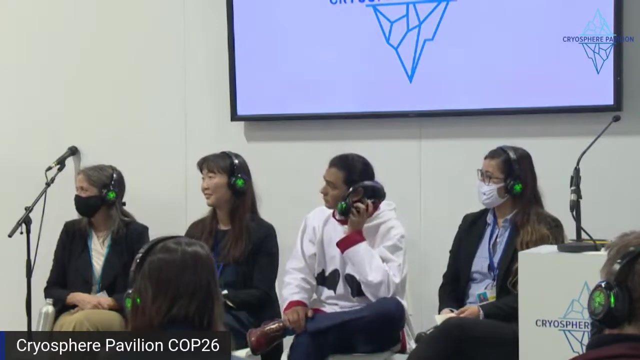 Thank you for the important question, Any. do we have any other questions from the floor today? OK, Oh, yes, we do. Hi, I can't. Yeah, it's very strange listening and not listening. I'm just wondering about any tips you might have. 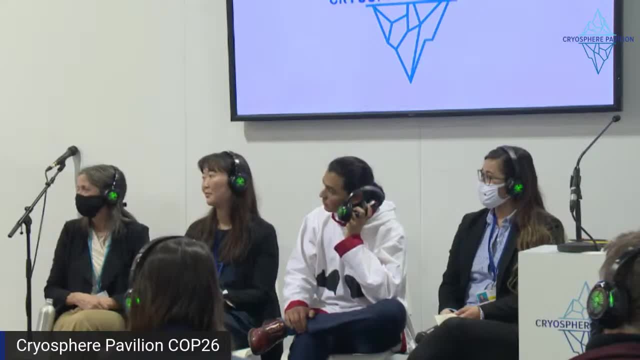 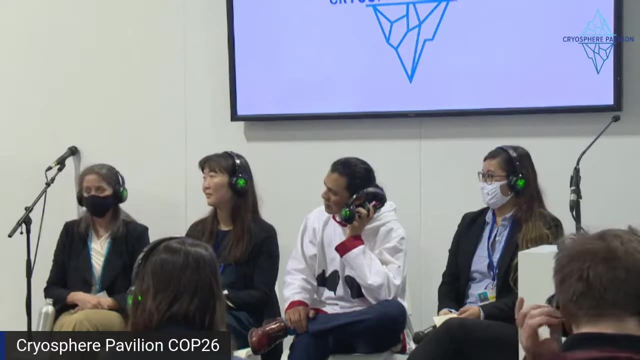 It might not be in your remit for how to get that funding to Include payments to indigenous people and communities that are participating in research and whether academic funders look at that favorably. You know you don't necessarily have to have answers to that. 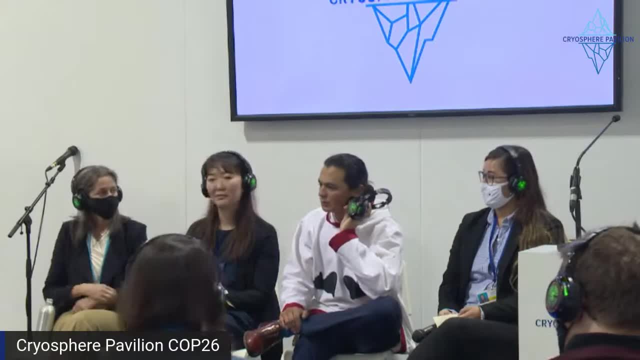 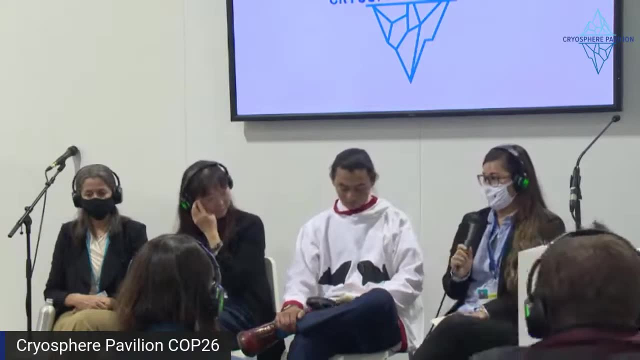 It's a good principle, but if you do have any, that would be great to hear. Thanks, Yeah, So in in my experience in Alaska, I know one person who's involving indigenous people in their research and is providing financial compensation, And so to collect. 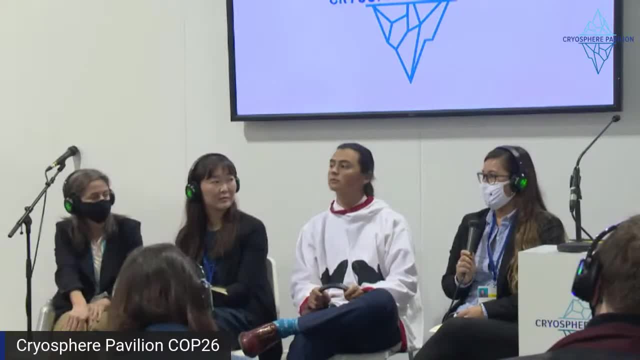 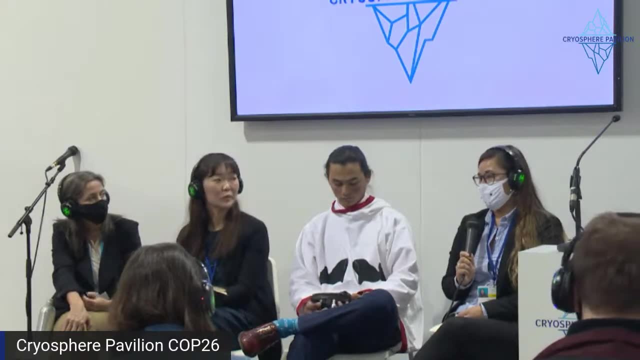 Collect data, things like that. That's one that I've heard of in the entire state And there are three universities in that state. in Alaska. He was my advisor for my PhD. that I did very briefly- Didn't finish with Drew because of ethical reasons. 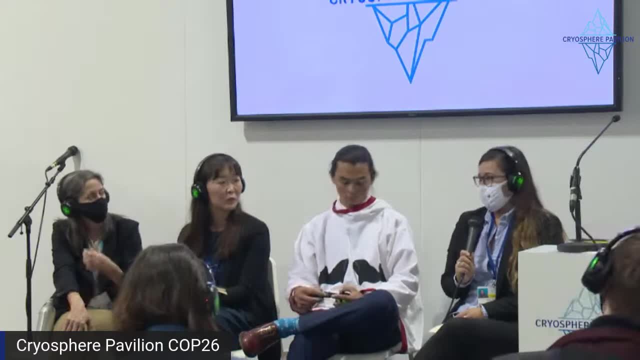 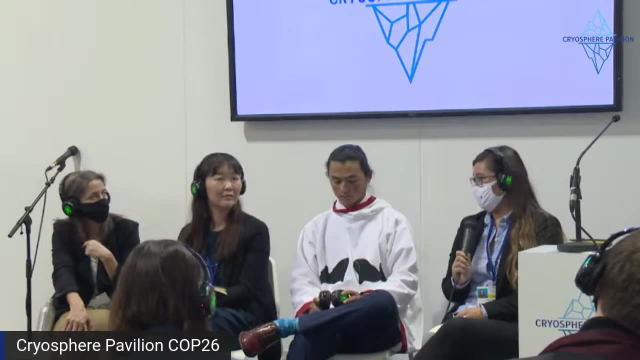 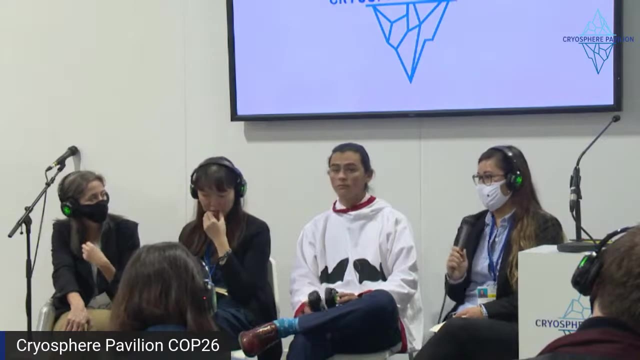 But yeah, I mean just do it period for in terms of advice on how to include indigenous people and get that funding to them. Um work with policy Policy makers, get lawyers involved, get other researchers involved, get all the necessary parties involved and just talk like get in a circle and talk and figure it out. 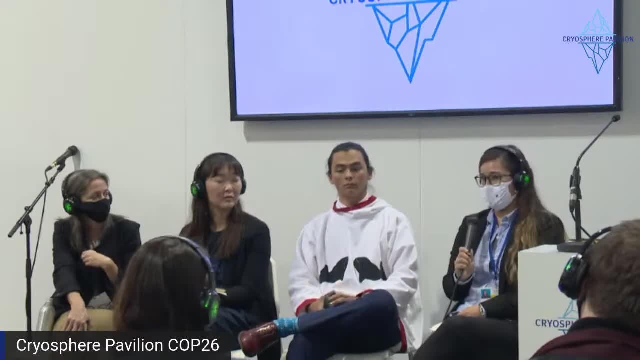 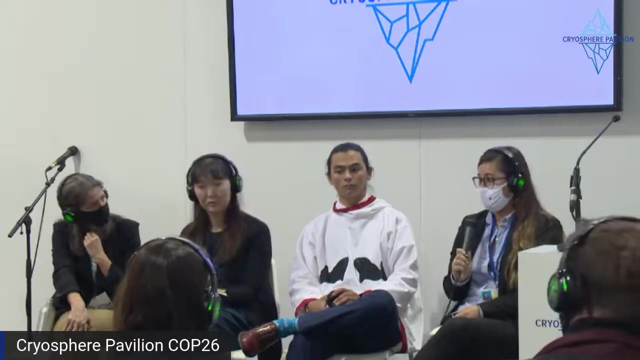 I mean, there are ways it seems really daunting because you don't learn how to do that in a PhD or in a master's, or you don't learn how to talk to people in academia. So I think that that is just a first practice that you can do in order to get the resources where they're going to be used best and just get indigenous people that money because they need it. I think that that is just a first practice that you can do in order to get the resources where they're going to be used best and just get indigenous people that money because they need it. So I think that that is just a first practice that you can do in order to get the resources where they're going to be used best and just get indigenous people that money because they need it. 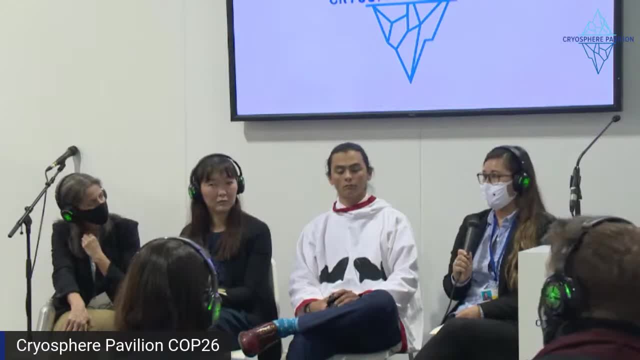 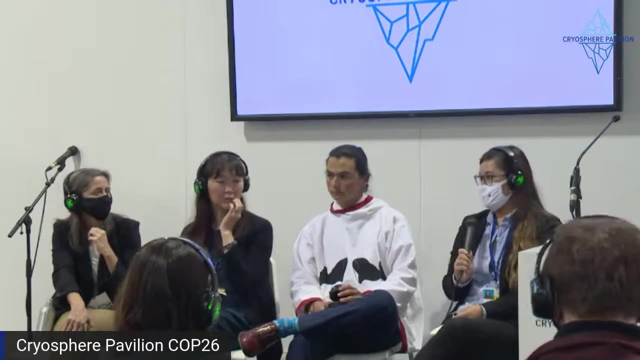 Money is always a good thing, but a lot of it usually, Yeah. I mean the amount that indigenous people get out of the total funds that are allocated is despairingly small, And it's in my- Yeah, from my- perspective. it's pretty, pretty polarized and not just at all.